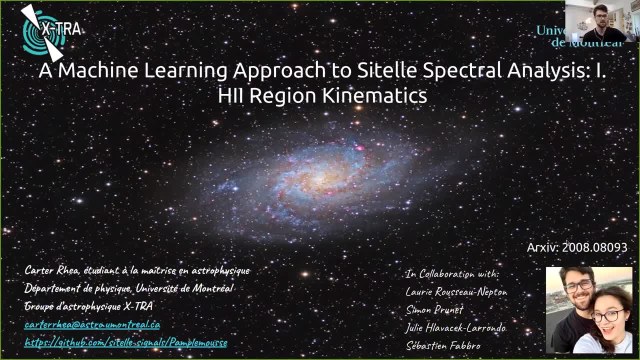 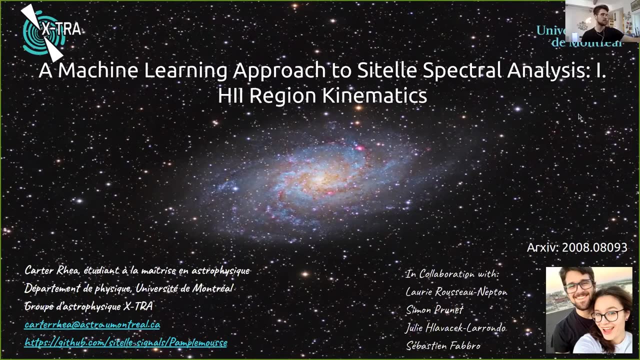 Journal two weeks ago and it's been put up on the archive so you can see it there. I also have included a set of kind of a manual of how we went through to do the machine learning and how to apply this machine learning at GitHub. You can see it at the bottom. It's under the Satell Signals. 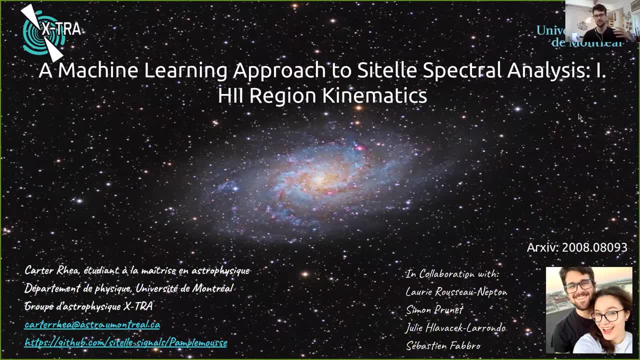 page named Pomplamoose. That's just a nickname for my cat. It doesn't stand for anything, I just like my cat a lot, So all right, well, let's get on with it, If it will get on Great. 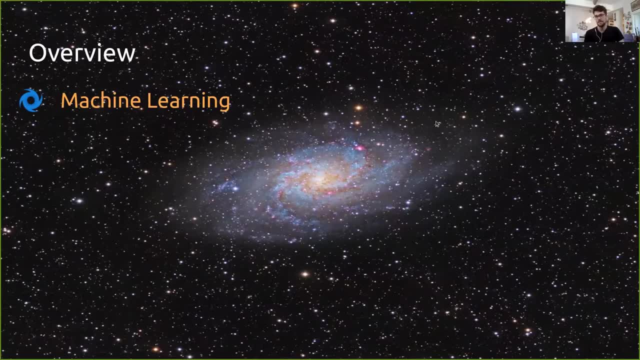 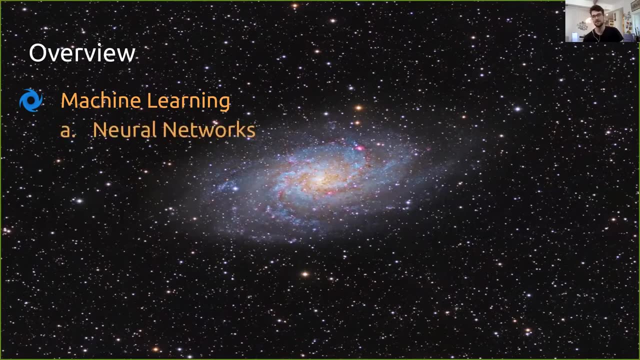 So, as an overview first, we're going to talk about, well, what is machine learning? It's certainly a black box for most people, quite understandably, but I hope to demystify it a little bit At least. I would like to demystify neural networks, which is a very, very powerful and 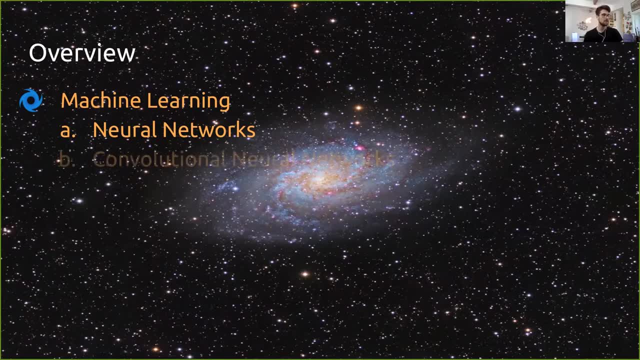 very popular algorithm for machine learning. We're going to be talking a little bit about convolutional neural networks and how the convolutional part extends a normal neural network, because that's what we used in this study. Again, very popular algorithm in machine learning. 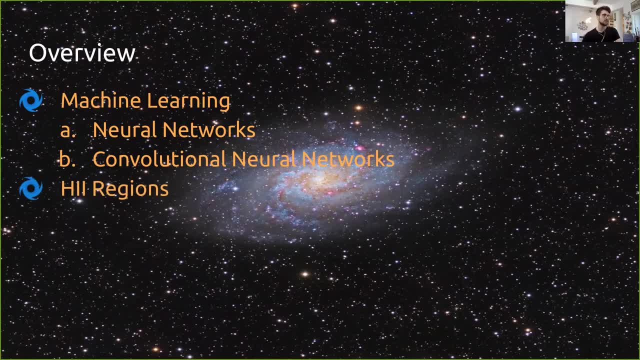 On the science side of things, getting a little away from it. we're going to talk a little bit about the computational part. We're going to be looking at H2 regions, so discussing what are H2 regions, how are they formed, how do they emit radiation and what might that radiation look like? 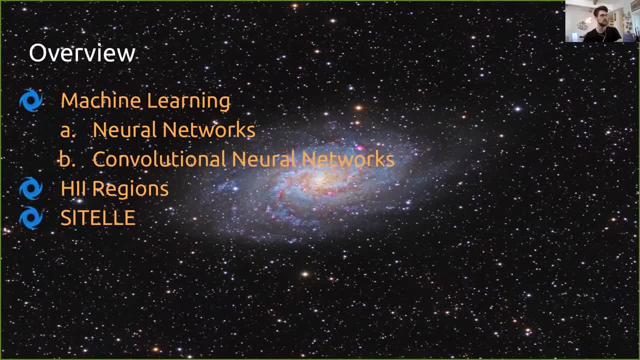 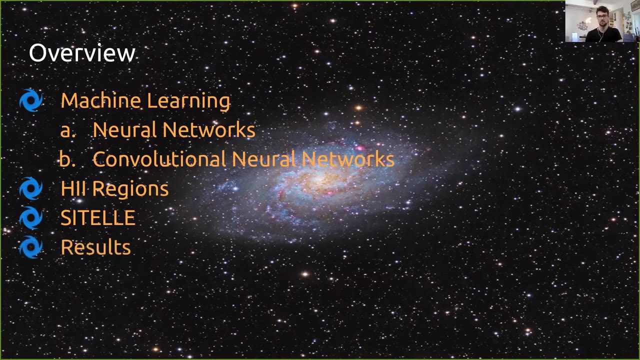 Finally, we'll move on to Satell, the relatively new instrument at the Canada France White Telescope, and also the Signals project, which is a long-term survey using Satell. Then we're going to talk about some of the results from applying machine learning to the Satell data. 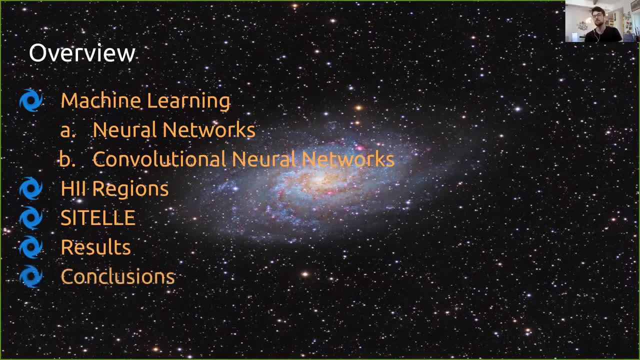 mainly the spectra. Finally, some conclusions and further work. so what we plan on working on next? I don't know if you saw, but there is a Roman numeral I. This is the first paper in a series of three or four papers. We have yet to decide, but we're actually almost done with the second and third. 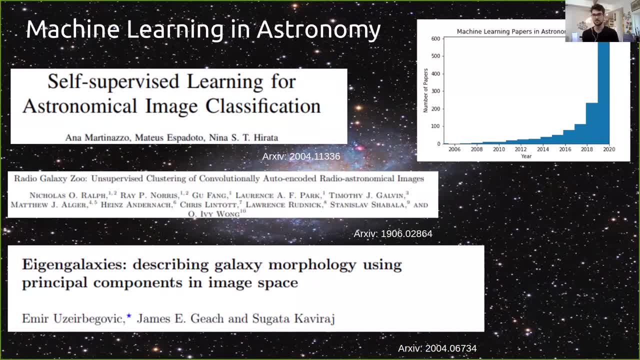 So machine learning and astronomy. I'm sure everybody's heard the word machine learning. It's been coming up a lot. It's very popular. I pulled together some of my favorite machine learning papers that I've read recently and you can see just from the titles that they cover a. 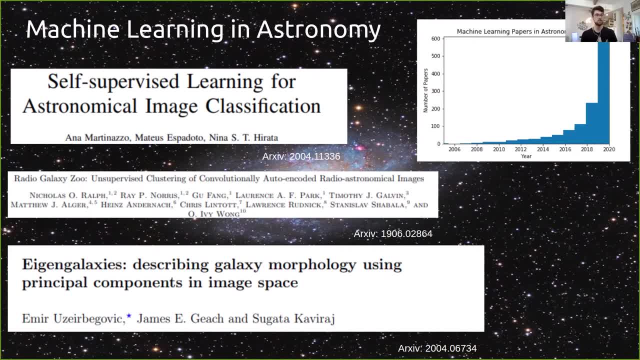 breadth of different topics. So you can use it for astronomical imaging classification. You can use it for clustering, in an unsupervised manner, different images. One of my favorite papers is this Eigengalaxies paper where they construct eigengalaxies like eigenvectors to build. 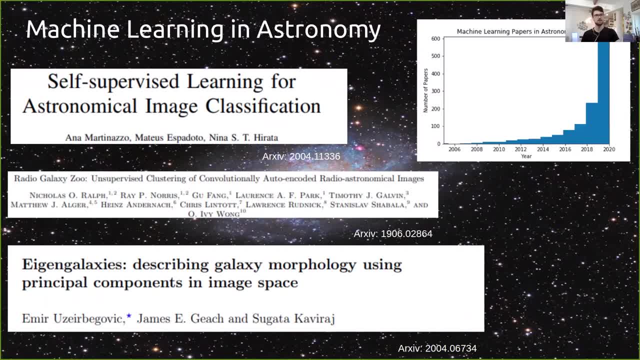 other galaxies and they can use that for its predictive properties. It's quite fascinating. I put together this little graph just to give everybody a good demonstration of how popular machine learning is coming in astronomy. So if you go into archive and search, 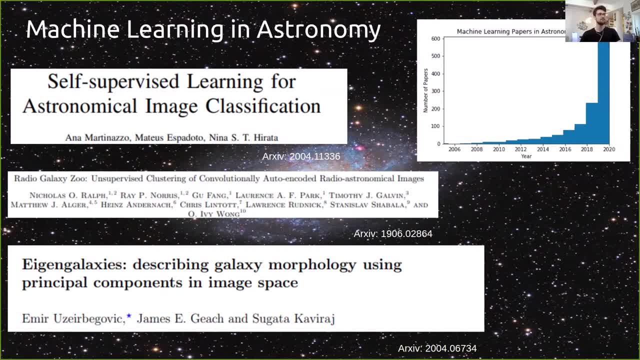 machine learning and astronomy, and you feel like plotting out the number of papers. this is what you'll see. So you can see that it's been exponentially growing significantly since about 2010,. and in the last year it's truly blown up. 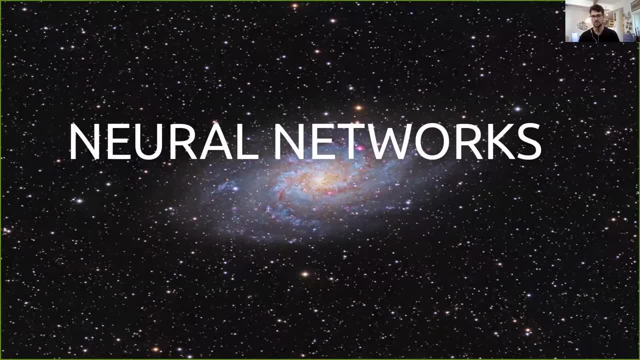 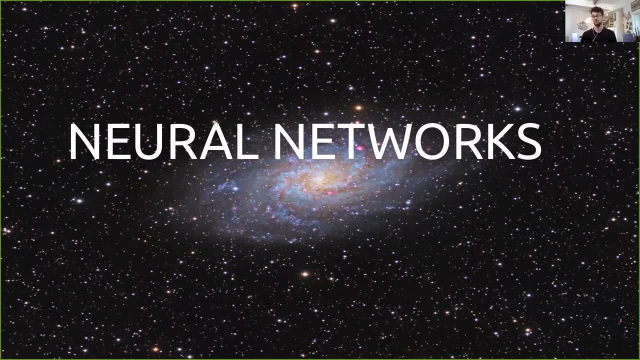 Okay, So now that we have a little overview on why machine learning seems interesting in astronomy, let's get into the actual weeds of what machine learning is in this context and what machine learning algorithms I'm using, or rather, my collaboration. 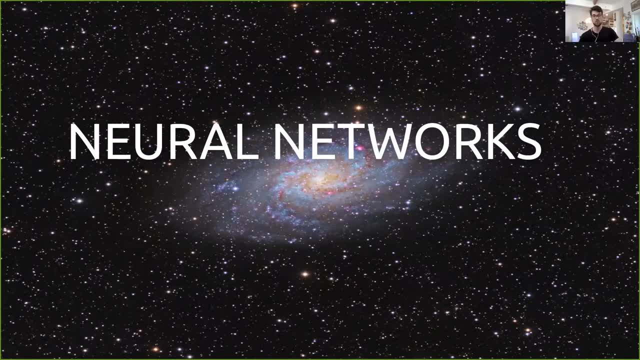 So we're going to be talking about neural networks. If neural networks make you think of biology and how the brain works, that's good, because that's what it's based off, and we're going to talk about that a little bit. So there are a ton of neural networks. 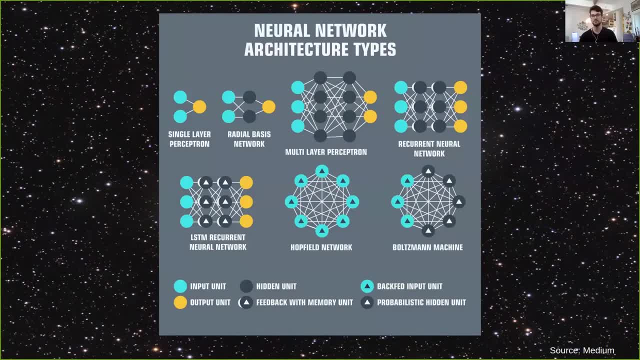 and these are the base neural networks that you can have. We're certainly not going to discuss all of them. The only one I really want us to focus on is this multilayer perceptron. I love this image just because it shows the variety of neural networks. 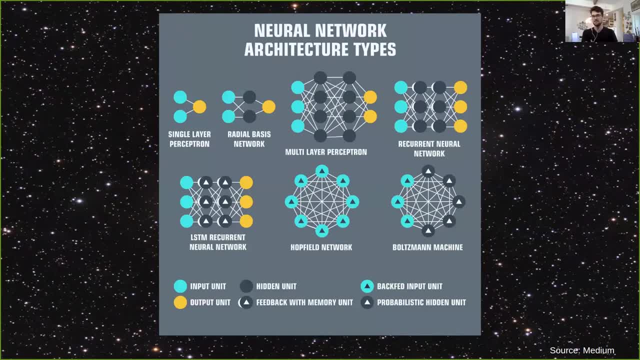 But the neural network that we're going to be using is relatively simple when you look at its architecture. So in blue you have your input layer. That's whatever input you're going to be putting into the algorithm. Of course you have these hidden layers, which is where a lot of that. 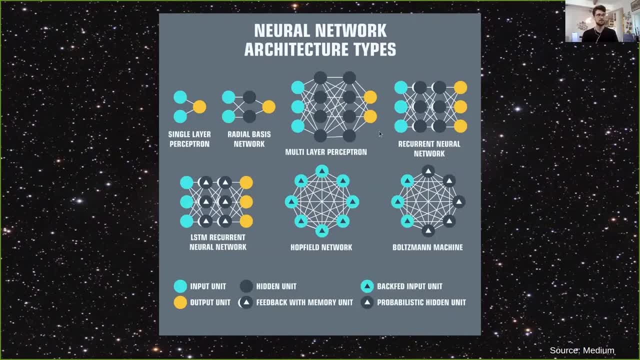 black box mystique of neural networks comes from. Calculations are going to be done there, and I'll describe what those calculations are. And then, finally, you have an output layer, and I'll be showing some examples of what that might look like, But for a neural network. 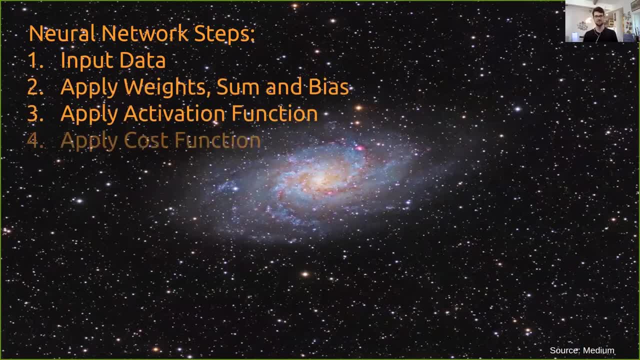 I like to think of it in some way like this. So I'm going to show you what a neural network looks like in seven relatively simple steps. Easy to say the steps. a little harder to do: the steps. So you're going to first collect your input data, which can actually be a real pain. You need 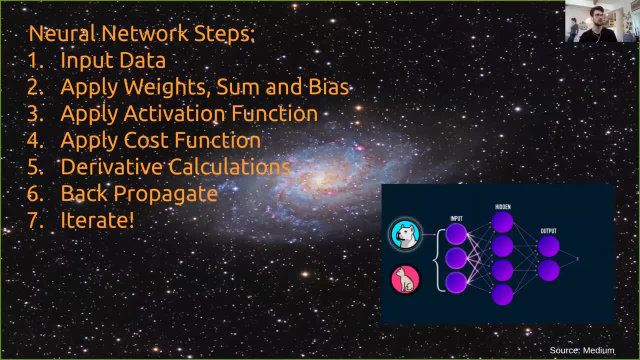 perfect or really really good input data and take a lot of time to do the preprocessing. Then, after you apply your input data, you're going to be applying a system of weights and biases at each one of those nodes in the hidden layers. That's what each one of those dots on the 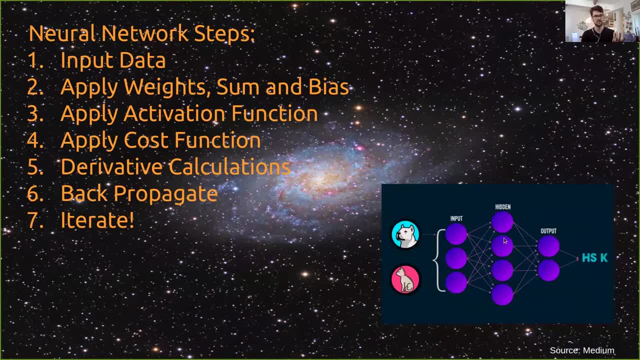 hidden layer represents, are called nodes. You can see it here At each node. after you apply those weights and biases and sum everything up, you're going to be applying something called an activation function, which you choose a priori. We'll talk about that a little as well. And then finally, 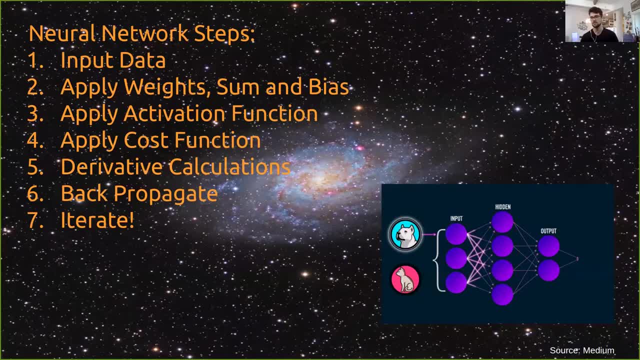 you're going to apply a cost function at the end And your cost function. what it's going to do is say, okay, here's what my neural network outputs, and I know what the answer should be And I want to minimize some cost function. So you want to see how well your network's doing with respect to 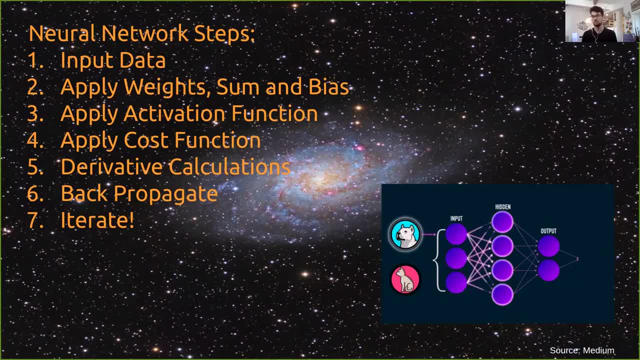 the known outputs. In this scenario, where you have known outputs, it's called a supervised machine learning algorithm. because you're going to be using a supervised machine learning algorithm, because you're supervising your network, because you know the final outputs- Great, So you've gone through. 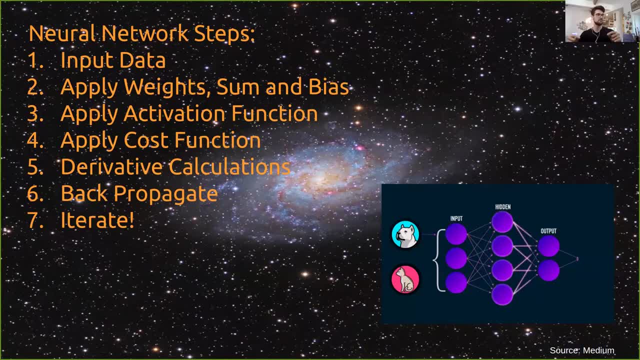 it. That's the feed forward part. We're going to get back to that terminology in a minute. But what if it didn't do very well? Well, if it didn't do very well, then we're going to go through a system. 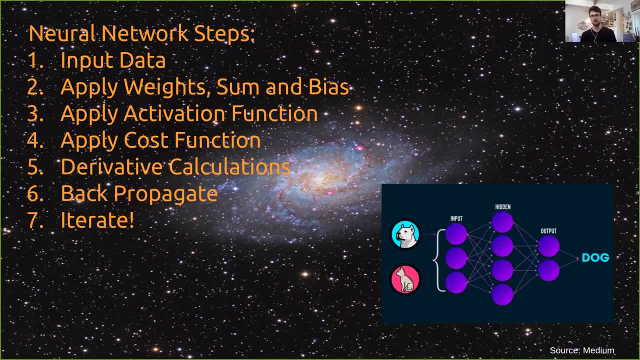 called back propagation, which is not too terrible as long as you're not actually doing the math yourself. It's a ton of derivatives. What you're going to be doing is calculating your derivatives to see which nodes have the most variance, And you're going to try to minimize that And when. 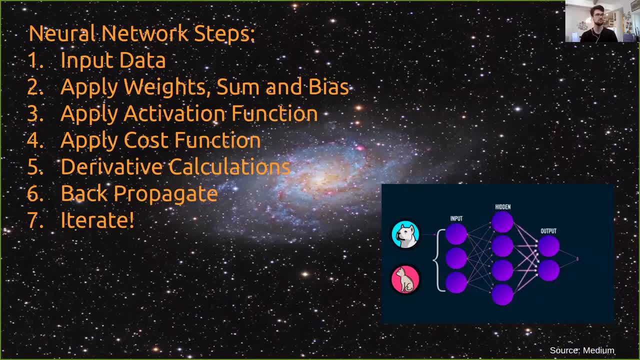 you're minimizing the derivatives, you're going to try to minimize that. And when you're minimizing the derivatives, it's going to be with respect to that cost function. And back propagation is the process in which you calculate those derivatives and then you update those weights that are on each 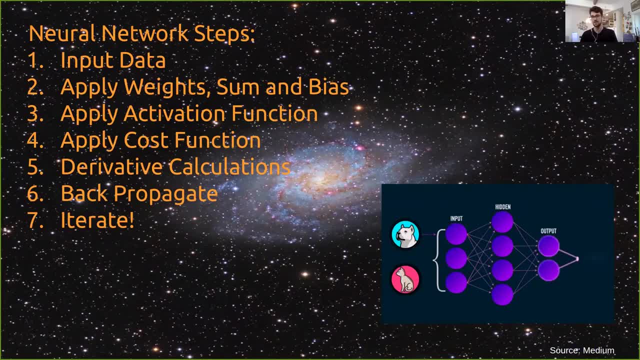 node. And then, of course, you iterate, See if you did any better, Reapply your cost function and go back and do that until you meet some certain threshold that you're okay with. So that's a really broad overview. Let's now go into each of the individual steps of how this neural network 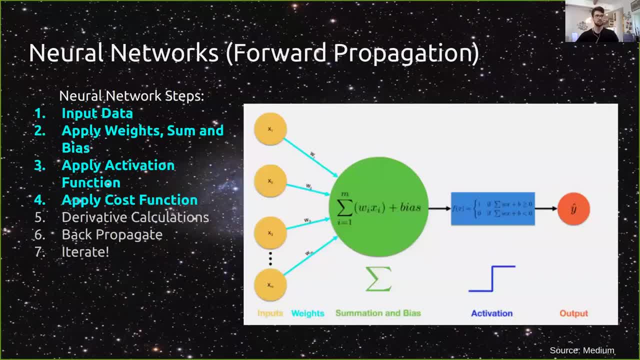 really works. So I break it up into three parts. So I break it up into three parts, So I break it up into two sections- And most people do. I certainly can't take credit for this. You'll see that the source is medium, It's a wonderful site And towards data science, they have a lot of 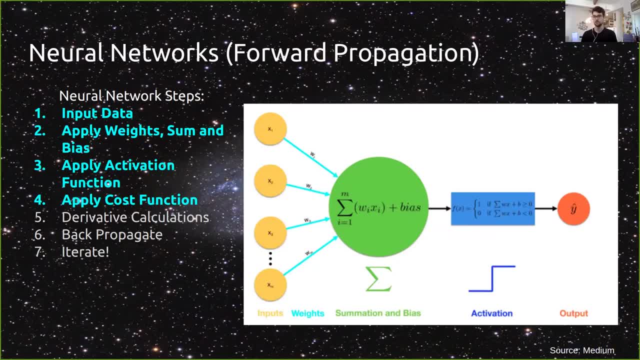 excellent articles, high-level articles on machine learning and other interesting data analysis techniques, And I suggest everybody take a look if they have more questions or, of course, write to me. So, during the feed forward propagation or feed forward step in your algorithm, this is: 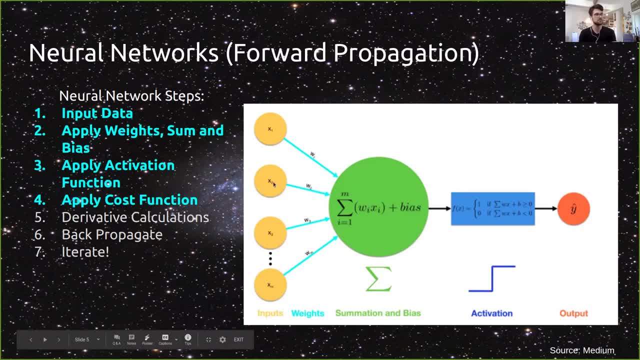 perhaps the most basic neural network you could ever come up with. You have a set of inputs, You have a single hidden layer with a single node And you have a single output. But it does a really good job of explaining how all other neural networks work, at least these types of neural 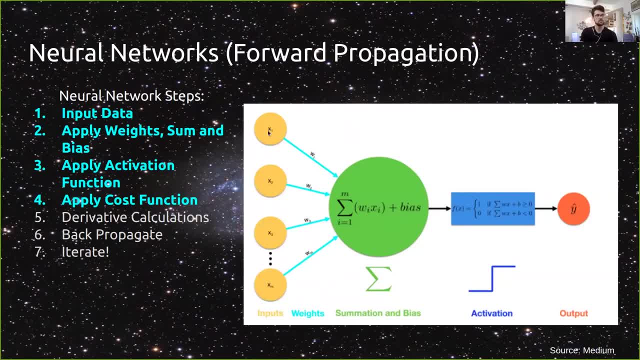 networks. So you have your inputs And for each input you apply some weight to that input And on your node you're going to be summing up those weights for all of the inputs. So weight times the input for each one of those And you're going to be adding some bias that you will choose. 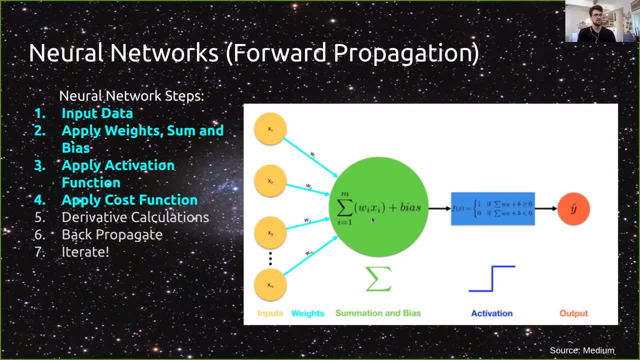 Or you can randomize it. There's a lot of different methods for that. And finally, you're going to be summing that up and applying some activation function. A lot of times, we use an activation function that ignores any negative value, So this is a really classic activation. 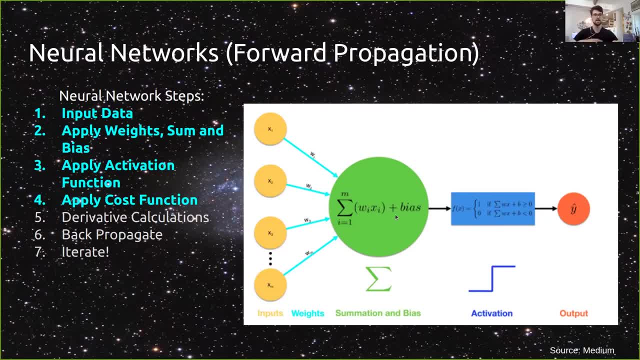 function that says: if, after my summation and bias, my node is positive, then I will give it a value of 1.. Otherwise it gets a value of 0.. That's just an example of it. So now we have our input data. 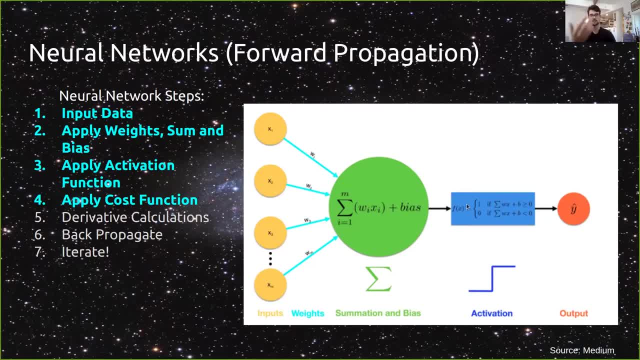 We've applied our weights, sums and biases, We've moved on and applied our activation function on the node And finally we have the output. This is where we apply the cost function that we choose. It can be something like a mean squared error is very popular mean absolute percentage error. It. 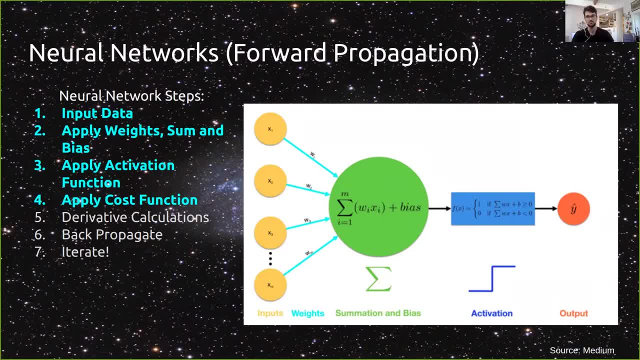 really depends on the problem And, of course, testing out to see which one works best for that problem. So you'll take a look at your output, See how it compares to the known truth, Calculate whichever cost function you want, And the idea is now you want to minimize that cost function. 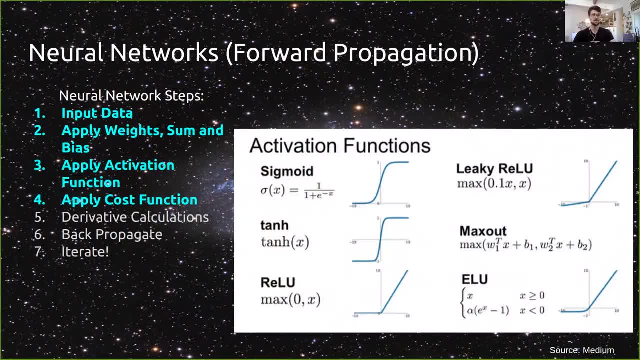 me give you just another look at some of the other activation functions. There are a lot of activation functions. They all get used to different amounts. One of the most popular ones, for good reason, is called the relu function. What it does is it sets any, if your node value. 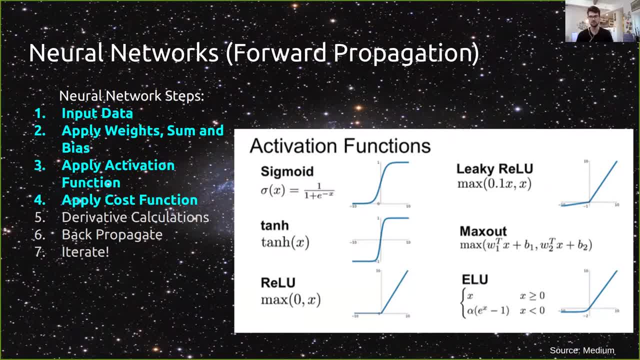 is zero after you or your node value is negative after you do the summation and add your bias, it activates it to zero. So it sets your node to zero, Otherwise it takes that value. It's a very interesting activation function. I talk a little bit about it more in my paper. 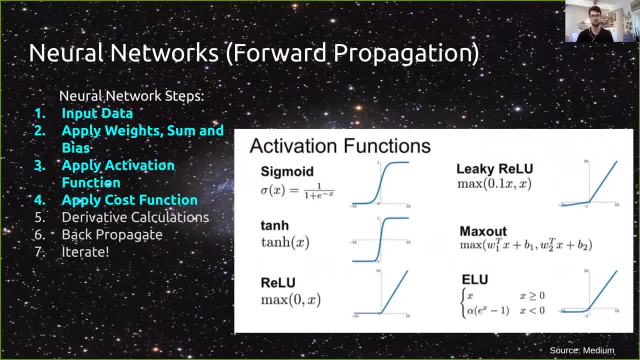 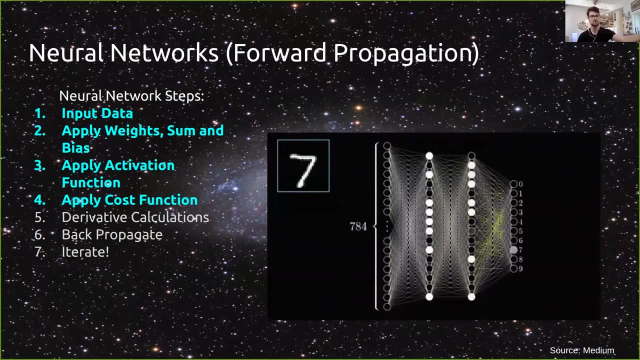 and the citations for it. What it does is it allows you to introduce a level of nonlinearity into your network. Here's a very simple example of how you might put an input. So they're taking this image, transforming it into a vector, It gets placed into the input And 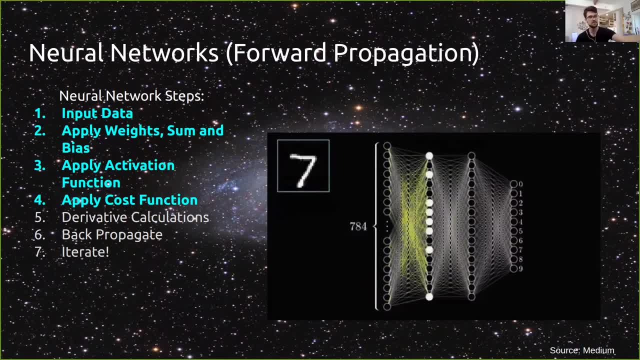 then you can see. after your input gets filled in, it gets moved through the network. The white nodes are the white nodes. The white nodes are the white nodes. The white nodes are the ones that are being activated And finally you get an output where you calculate. 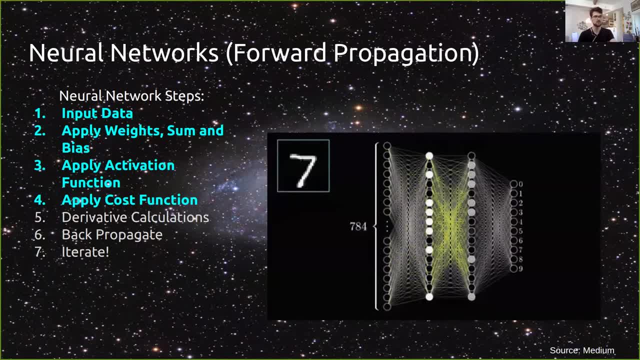 your cost function. This is a nice classification problem, Not always as easy as it looks, And I'll also point out here that those nodes between each layer there's something called fully connected, which means that each node in one layer is connected to all the other. 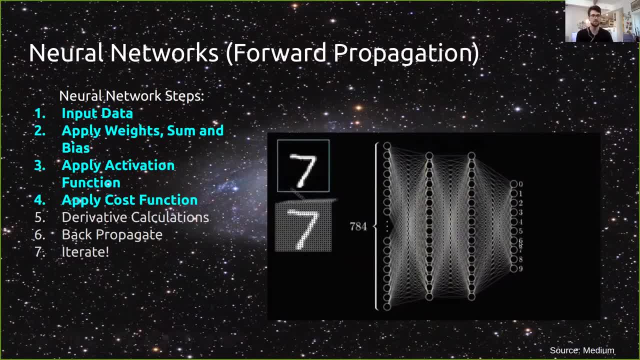 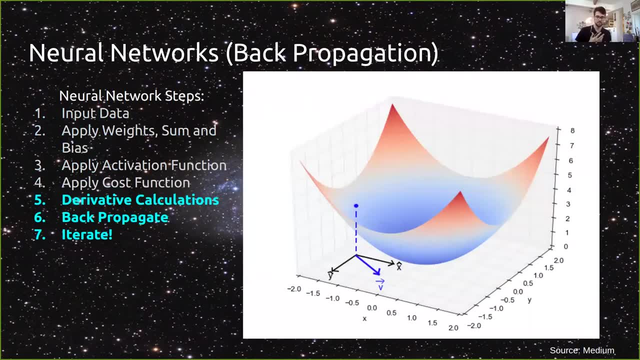 nodes in the layer right next to it. That's why you see all these crossing lines. All right, So once you've gone forward, you've you've got your input data, You've applied your weight and sums, You've applied your activation. 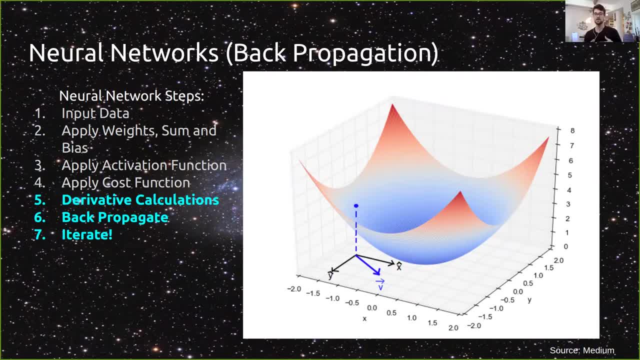 function And now you have your cost function to see how well you did. And now this is the point where we are actually training the algorithm. So that training step in machine learning is a step in which we go back and try to move those weights and biases a little bit, to try. 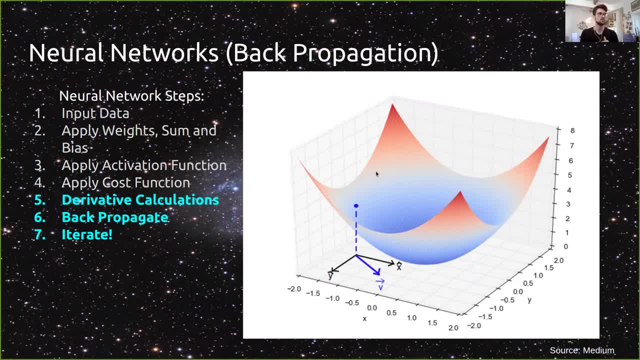 to optimize the algorithm to minimize our cost function. So here's a manifold that is meant to represent the cost function And we would like to minimize the cost function. So how do we go about minimizing our cost function? Yes, sorry, I would also like to mention this is a really beautiful cost function. 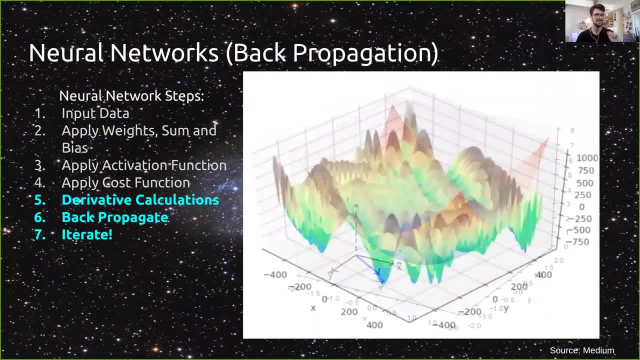 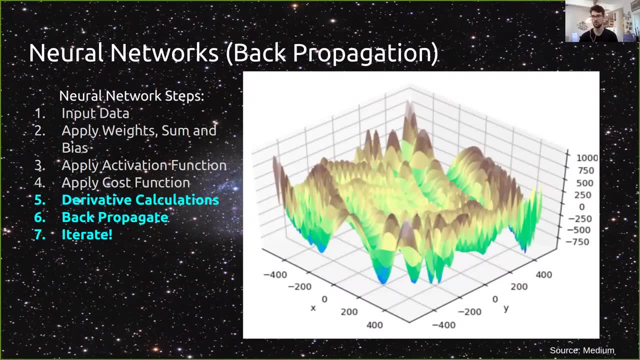 Really nice. There's a very clear minimum there. This is often what we're actually left with: very horrendous minimization problems that can be incredibly difficult to solve. So how do you go about solving these problems? I apologize- Not for the meme, but I apologize. 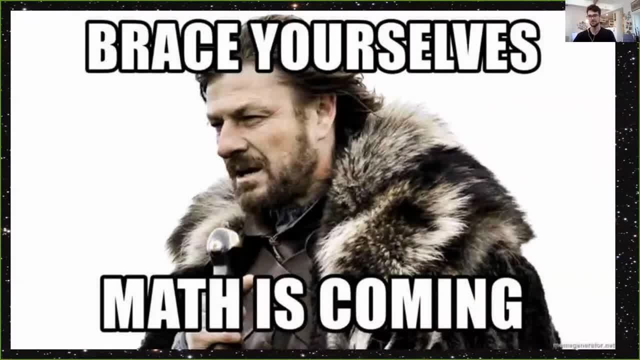 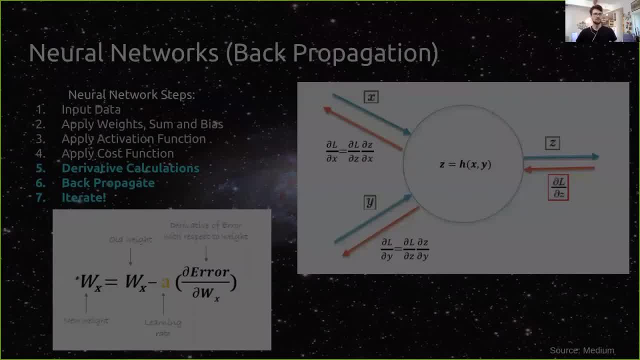 that math is coming. There's a little bit of math, but it's mainly just derivatives- For everybody who remembers our optimization in help 3 or whenever you did it. So this back propagation, step after we have applied our cost function and we see what our values. 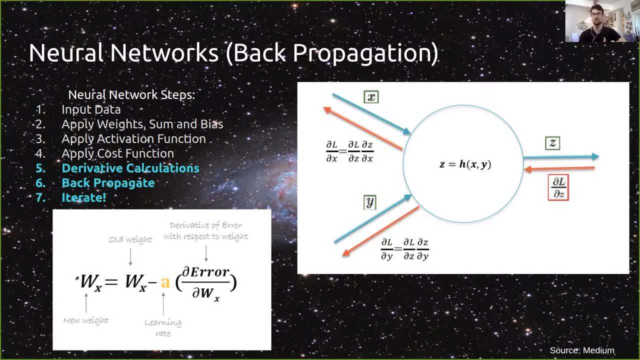 are. what we're going to want to do is we're going to want to go back and look at our nodes and see how those nodes change with our output and calculate those derivatives And how each node changes with other nodes, because it's a fully connected system. So you're going 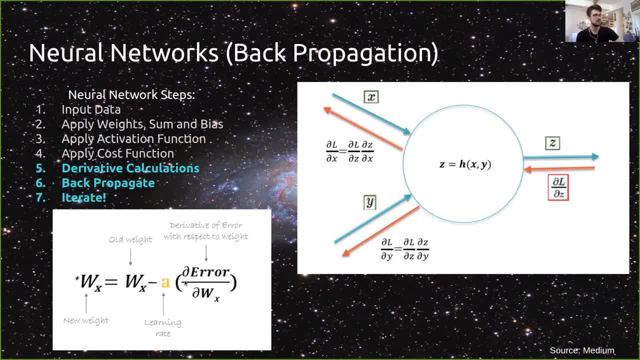 to be calculating all of those derivatives, And this is particularly important because The partial derivative of your error with respect to one of your weights. So this is your weight update equation. So our new weights are just going to be the old weight minus some learning rate, which is a fun hyper parameter. 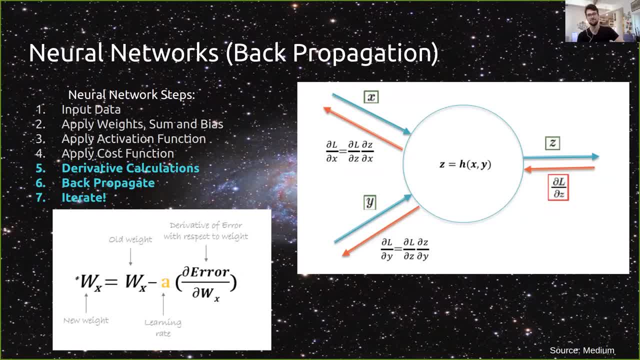 Which means it's parameter you get to choose a priori and change if you want. There is a large step involved to try to fine-tune this parameter. that happens later on. But the important part here it's the derivative of your error with respect to your weight. 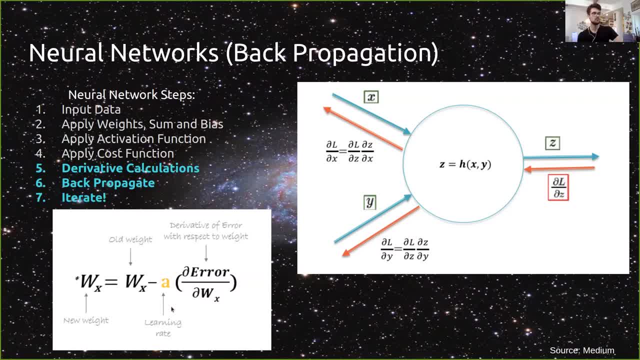 So you want to see how your error is changing With respect to the weight of a node, and you do this for all of your nodes and use this simple formula to update it With new weights. that is that derivative calculation and back propagation step. now we have new weights. 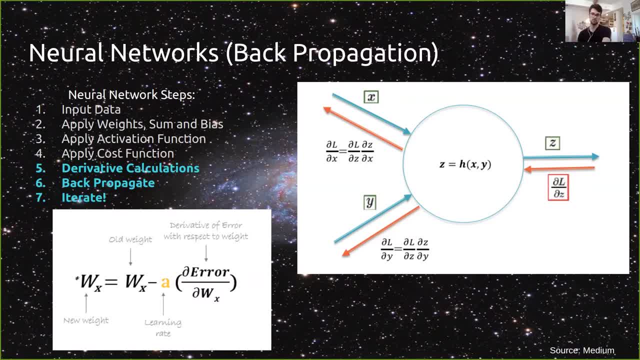 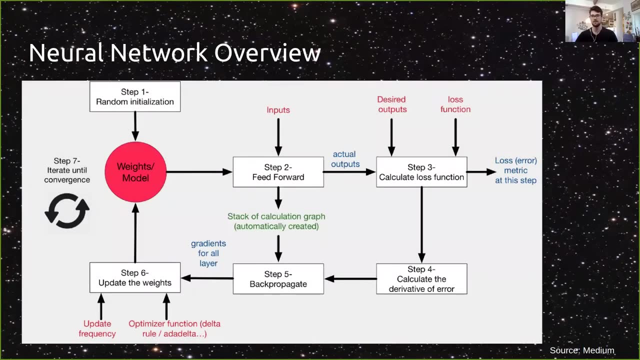 So now we can go ahead and do that forward program or forward step again, the the forward propagation, and Recalculate our cost function and see how we're doing and we're going to iterate that until you reach a certain tolerance. So that is a very Kind of high-level overview of how these neural networks 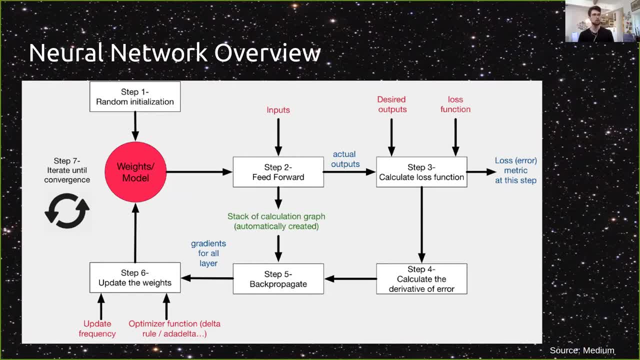 Actually work for a very simple perceptron neural network. I really like this. I think it's a nice diagram to bring you through. So the idea is: you have your. you have So step one: you randomly initialize all your weights. a lot of different ways to choose how to go about that. 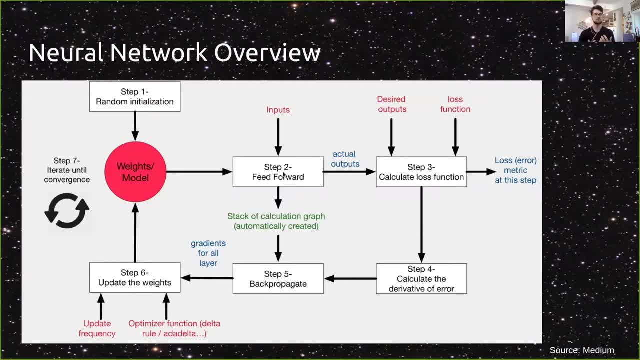 And you apply your input function. You do that feed forward step where you move through your network and then you calculate your loss function. See how well you did. Then you're going to be calculating. droid is your error. to try to do a better job, try to update your nodes. 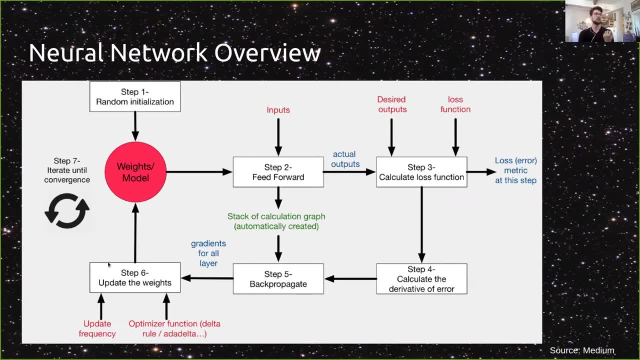 That's this back propagation step, Also updating your weights, and then you're going to go through the same thing again And you're going to iterate this again and again. a step seven says, until you converge to some value in whatever loss metric You're using. so, whatever your cost, function metric is to reach a certain threshold. 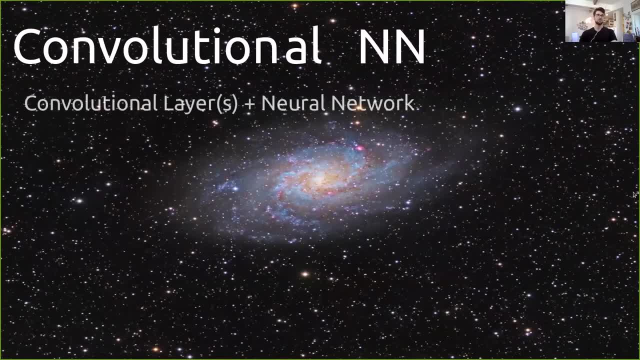 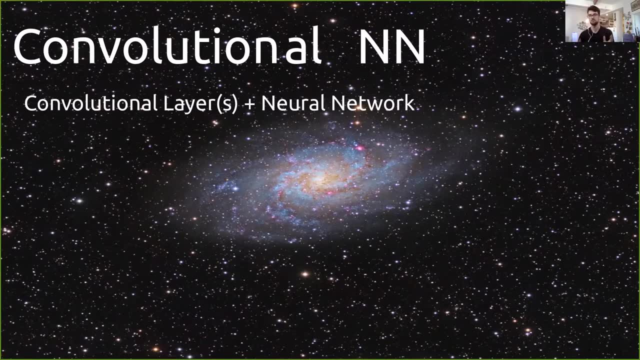 Great. so we talked about neural networks, but what are convolutional Neural networks? well, as the name suggests, they are a convolutional layer or multiple convolutional layers plus a neural network. the convolution Convolutional layer does not work as a neural network. It is in fact the convolution that you know from. 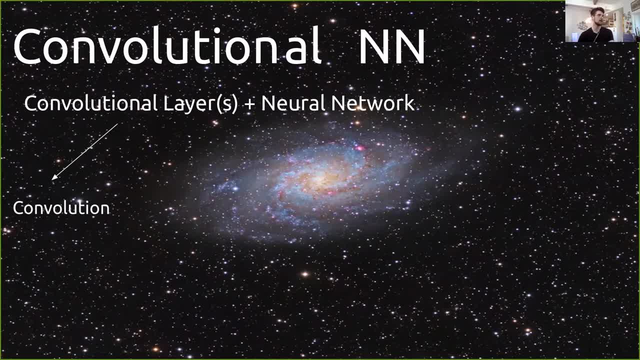 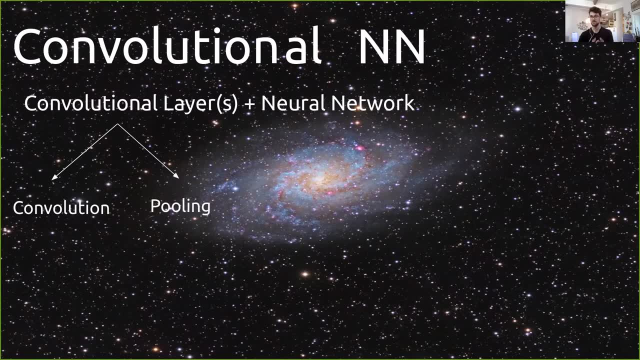 Math if you had to take it then an undergraduate- or perhaps quantum mechanics and treated some convolution there. But the idea in the convolutional step is you're going to convolve your input with something. we'll talk about that- a convolutional kernel, and there's normally a 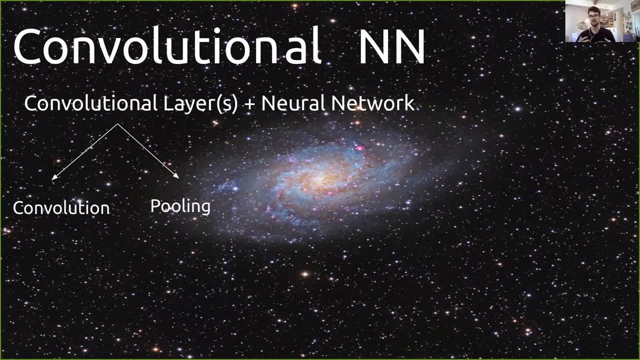 pooling step, which is a way that you can downsize the data, make it a little bit more manageable for the neural network and Really try to pick out the important pieces. So this whole convolutional layer piece came from image processing. mainly convolutional neural networks have been used for. 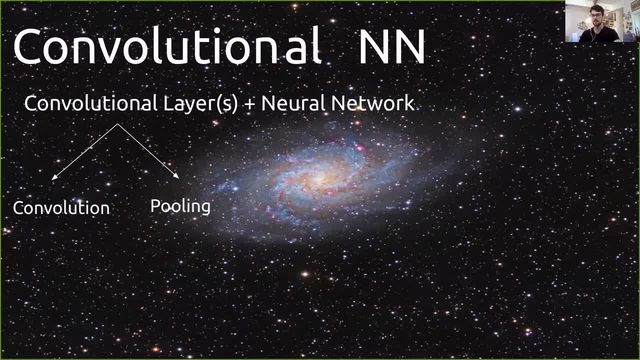 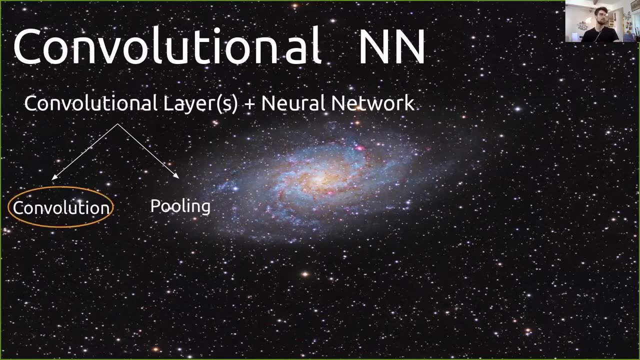 Image problems, so image classification problems in neural networks and in machine learning, and the whole idea of that convolutional, convolutional layer before the neural network is to Make the data is to ignore the unimportant pieces of the data and find the important pieces. So I said there are two pieces. we have the convolutional part and then a pooling part. So what is convolution? 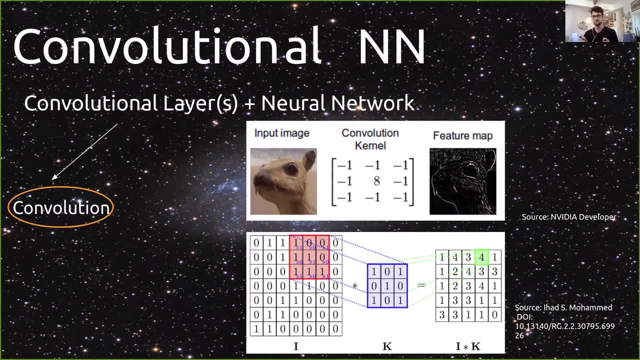 convolution is just a matrix operation and The idea is you have your input image, you pick some convolutional kernel and after you apply the matrix multiplication, You're going to be getting something called a feature map and the idea is you want that feature map to be representative of the most. 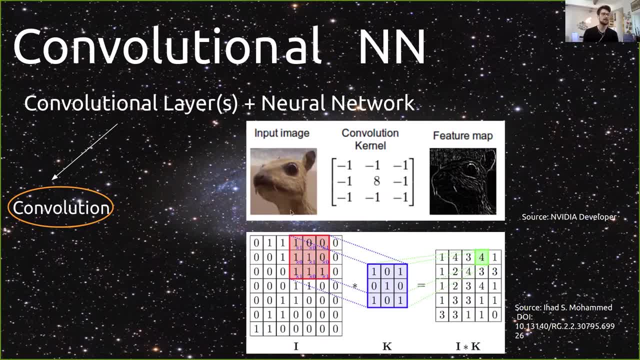 important features in the image. I Have no idea what this animal is but I love this demonstration. So they applied a convolutional curl to the kernel to be. I put image this guy and you can see his feature map. You can see that it's really pulling out the big changes in that picture, the most important pieces of that picture. 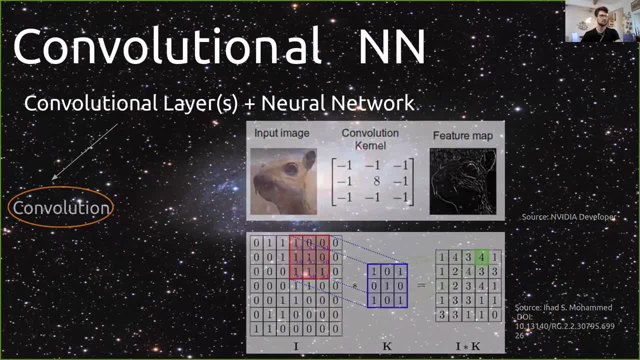 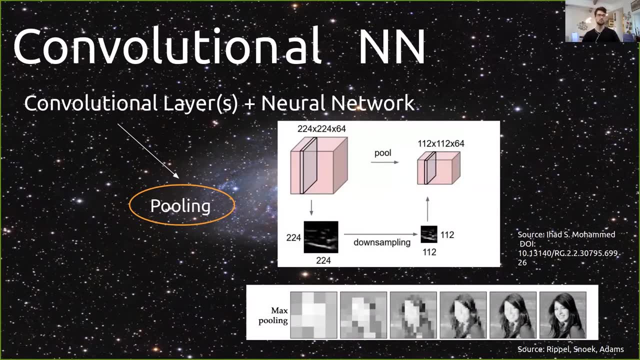 So that's a convolutional step. you can do this multiple times To pull out different levels of important features. Then, of course, we have a pooling step, the pooling step in its most simple form. what it does is it takes a high resolution image And it it pulls it. it down samples. It pulls it down to a smaller size. Of course you're gonna lose information. 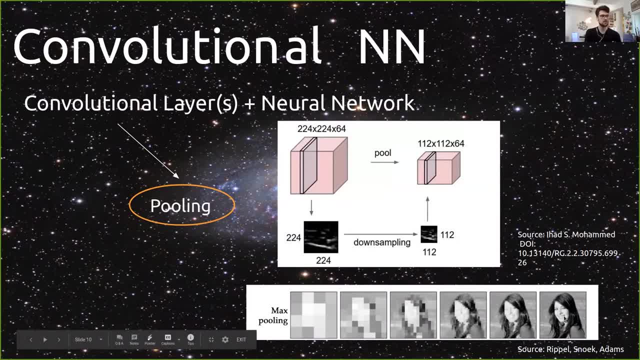 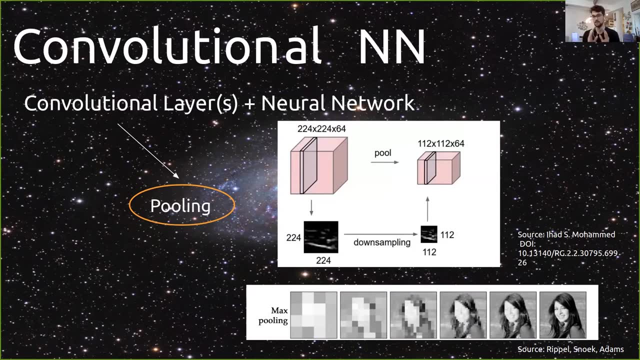 This is a wonderful image That demonstrates this. so on the right, we have a normal high resolution image and what they're doing here is they're taking little chunks, Four by four chunks, and taking the max value within that chunk Chunk of the image and then taking that as the true value for that region. So this is the max pooling. 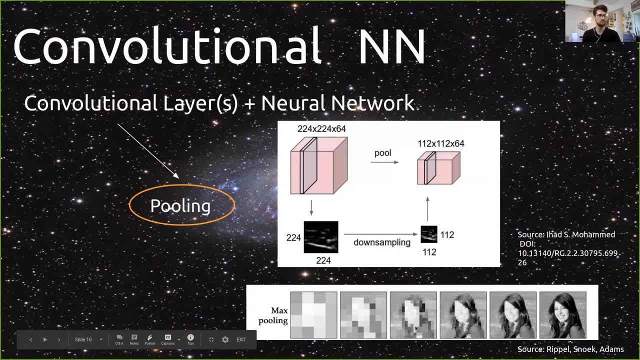 Sorry, max, not the average. This is a max pooling system and you can see that it's. you're losing information, certainly, but there's a question of: do you need all that information to actually answer the problem correctly, and is it perhaps introducing more errors into your neural network? So those are. 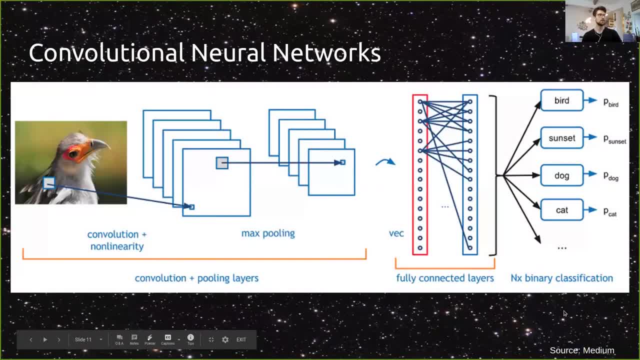 the two steps in a convolutional layer. When you pull together a convolutional neural network, what you're doing is you're taking your image or vector or whatever. it doesn't have to be an image. In our case, we're using spectra and you'll see that in a moment. So you take an image. 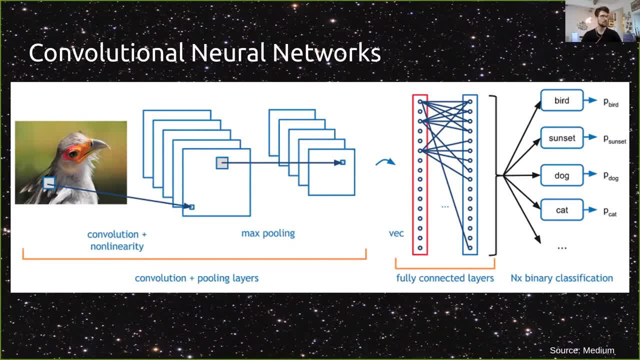 you convolve it with the function that you choose a priori. You often then pull the image to make it smaller, lower the input vector Again. this is not necessary. Then you're going to take that and run it through your neural network like normal. So everything over here on the right. 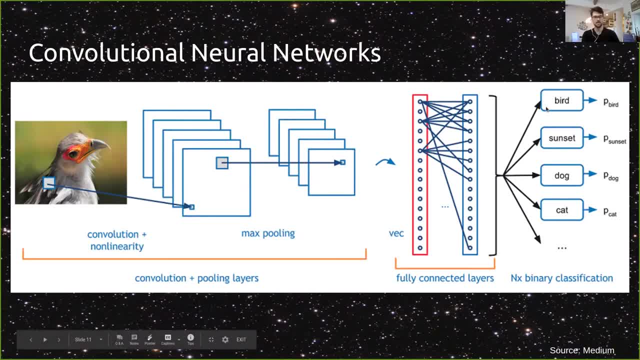 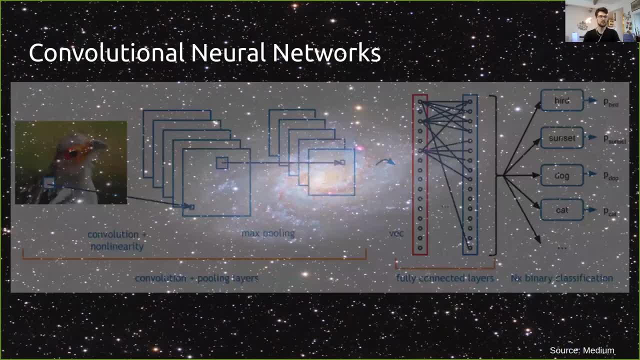 side is just your normal perceptron neural network. It doesn't have to be a perceptron neural network, but that's what we use and it's definitely one of my favorites. I have a video demonstrating how these convolutional neural networks work. So on the 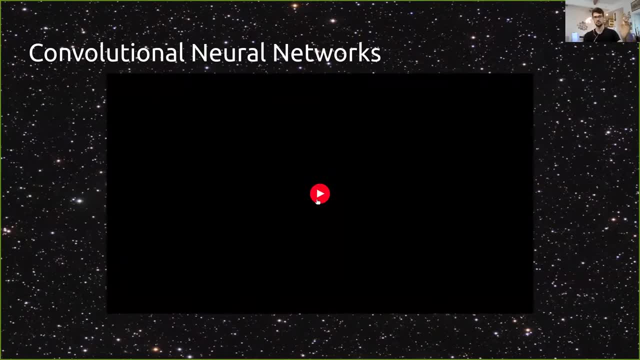 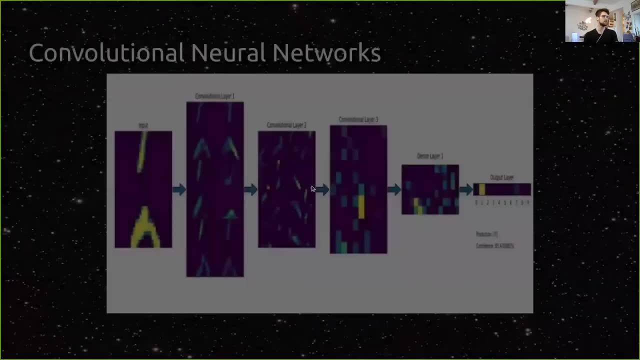 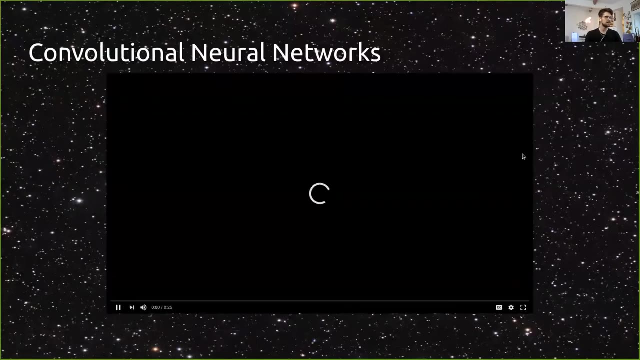 right, you're going to see an image. It's going to go through several convolutional steps and then be passed on to the neural network to do the actual classification. Oh no, to do the actual classification. Maybe it won't work. Okay, So, as you can see, they take an input, they convolve it. 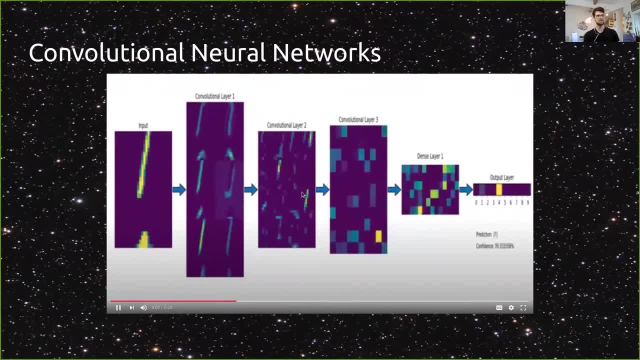 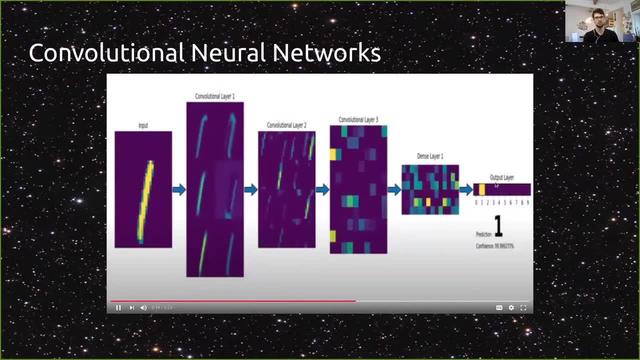 pick out the most important pieces, Convolve it again to pick out some other pieces, Convolve it again to try to see what's most important and then pass it on to this dense layer which would be a neural network and, finally, an 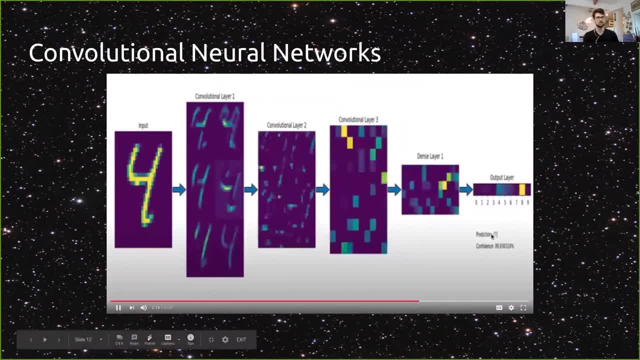 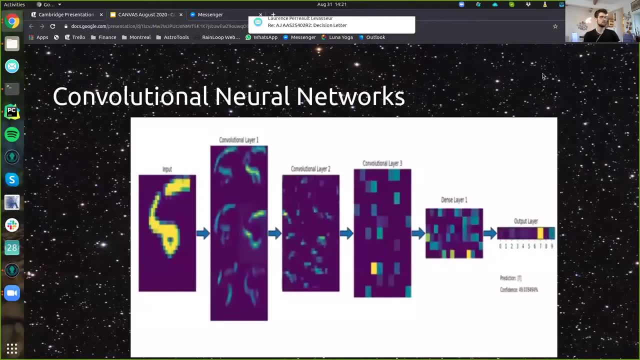 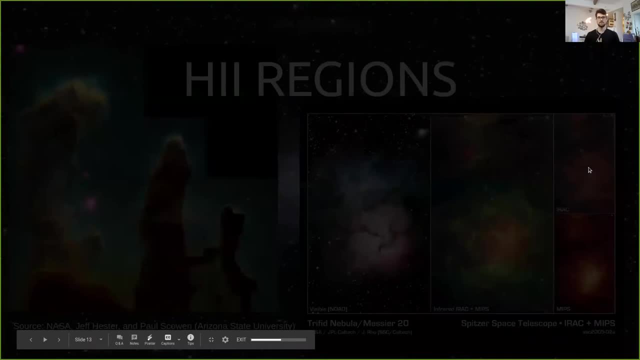 output. This is a very rough image of what a convolutional neural network might look like. Okay, So now that we hopefully have a decent idea of how convolutional neural networks work, and if there are any questions, please feel free to ask them in the comments. 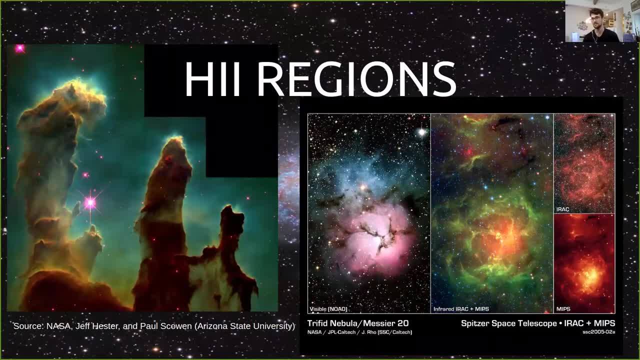 If you have any questions on convolutional neural networks, I would suggest asking them now, or you can wait till the end, of course, But if there aren't any, then I'm just going to go on. So onto the science side of things. right, We're all astronomers here, So where's the fun science? So we're looking at. 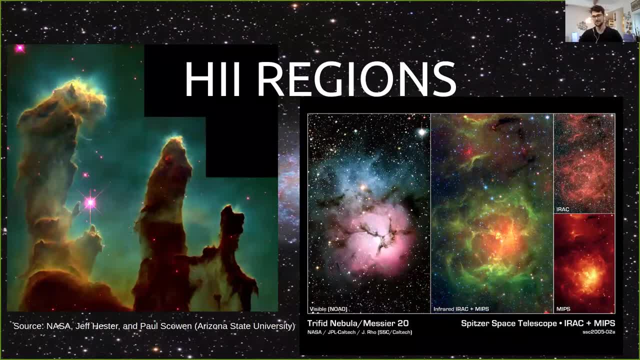 each two regions. Each two regions are regions of dust and gas, mainly in hydrogen and helium- A big surprise. as the name suggests, There are also a significant amount of other metals in there. But those H2 regions are the images that you see from the Hubble Space Telescope, for example. 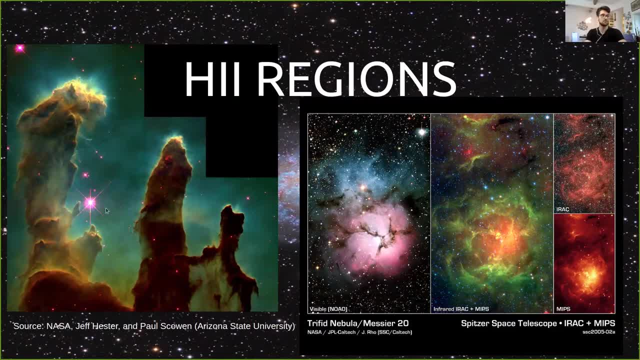 that are absolutely fantastic and beautiful. Here's pillars of creation: Very, very popular H2 region. Here is Messier 20, or Trifid Nebula, taken in multiple different wavelengths, And what you see, and what's interesting about H2 regions is it's where stars are formed. These are the 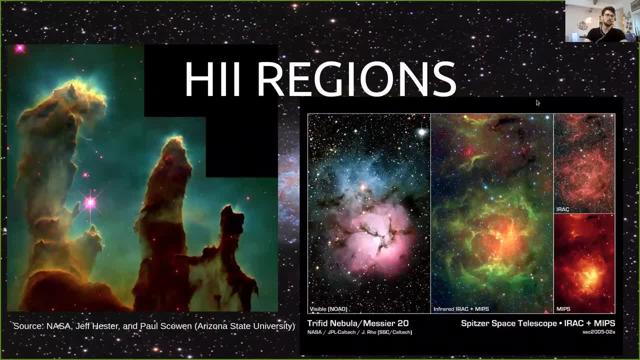 stellar nurseries that are so interesting. A lot you can see in the visible. There's a lot of dust here that's obscuring. You have the infrared- We'll track again the infrared- And this is pulling out some of the UV, if I'm correct, looking at some of the star clusters. So how do H2 regions work? 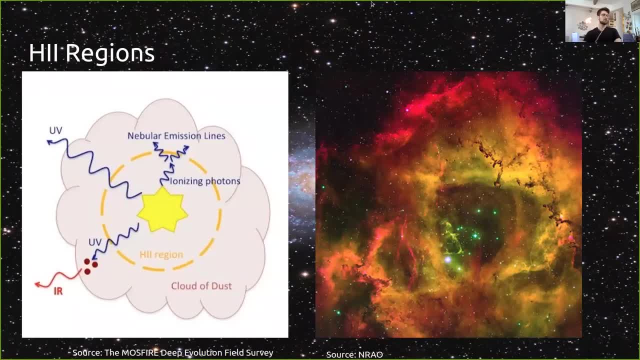 A simple image for an H2 region is this one: on the left, You have a cloud of dust and gas mainly comprised of hydrogen and helium, with some other metals. You have a very bright O, b or b star or a globular cluster of O- b stars, And then you have the star clusters And then you get a very bright. very bright O? b or b star or a globular cluster of O? b stars. At the top there's a bulb like a bit of an O b, O r or a globular cluster of O? b stars, And then you have clouds of iron which are entirely 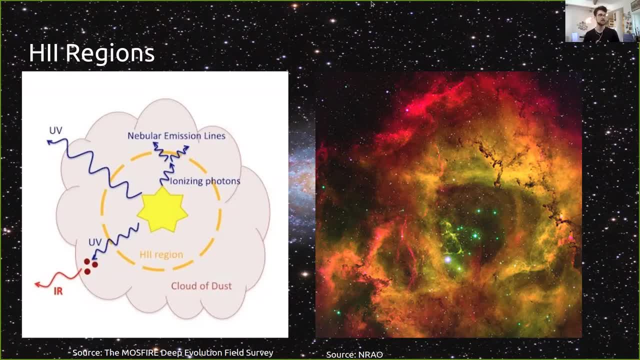 center that are just born. so they're incredibly hot, they're radiating a ton, they're letting out a lot of UV emission That's going to affect that cloud of dust. It's going to, and we'll talk about how this happens. but you have two. 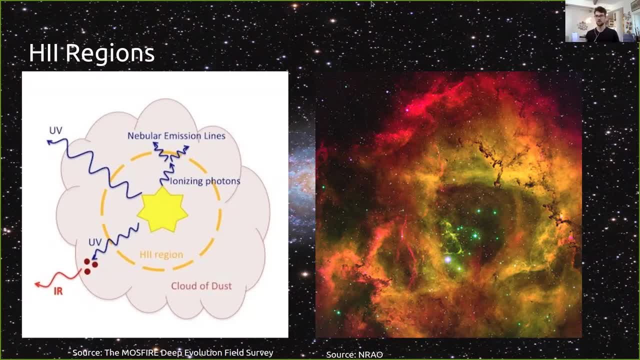 different types of photon emission processes that happen in the dust due to these ionizing photons coming from your central star or globular cluster, And what happens is you're going to have these nebular emission lines And nebular emission lines are coming- that's that radiative signature coming from the 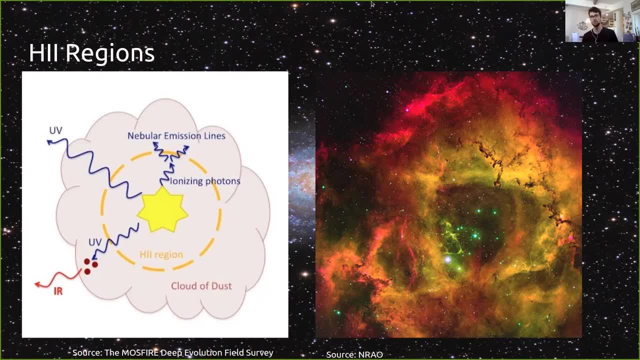 cloud of dust, And that's what we are interested in. when we use Sattel, for instance, You can see these in the optical quite a lot. So what are those radiative processes that lead to nebular emission lines? So keep in mind we're. 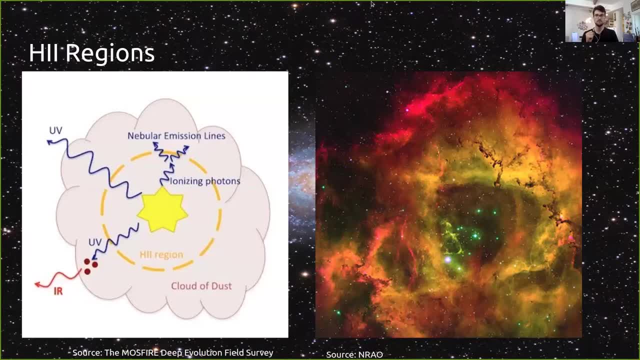 talking about a very hot young OB star at the center of a massive cloud of dust full of hydrogen, helium and sodium. And that's a very hot young OB star at the center of a massive cloud of dust full of hydrogen helium and sodium, And so 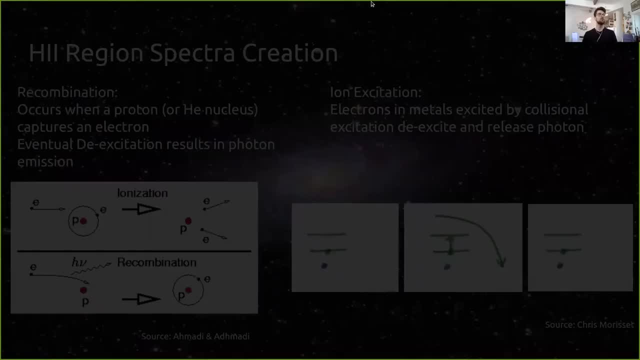 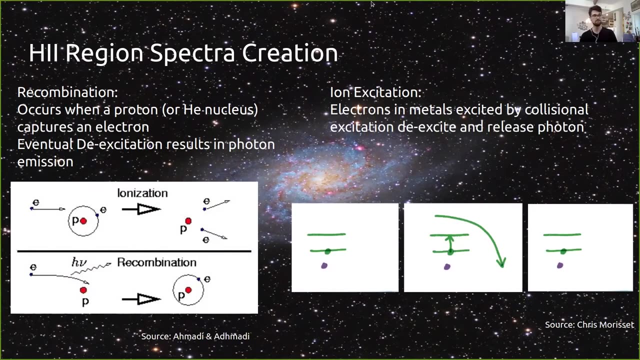 other metals. So there are two main ways to create those nebular emission lines or those or the resulting spectra that you might see in an H2 region. So of course we have ionization happening right. We have our cloud of dust, we have 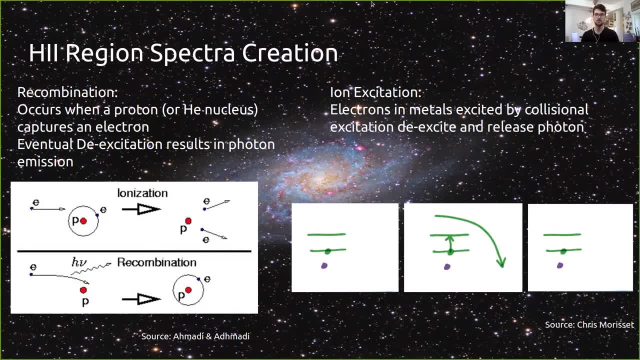 our hot star. it's emitting a ton of photons and those photons are ionizing the dust and gas. But there are other electrons hanging out and those get recaptured by the, the atoms, or in this case a proton, in this example, and 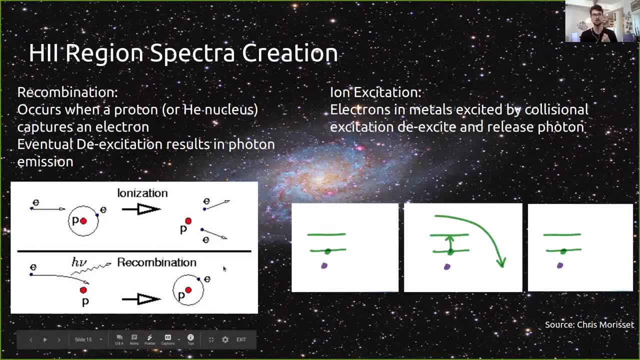 what is known as recombination. Those recombination lines are often found in hydrogen and helium and it's really that capture of the electron. and when the electron gets captured normally by a proton or helium nucleus, it ejects a photon following normal quantum mechanics collisional calculations. So 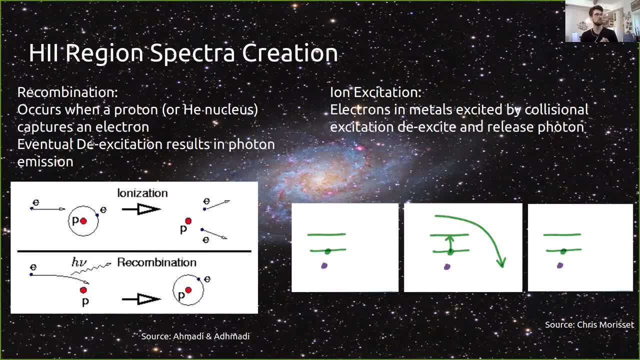 the other main mechanism. so recombination mainly applies to hydrogen and helium. The other main mechanism of emission- lines in your nebula are gonna be from ion excitation. I stole these fun images from Chris Morissette. I thought they were very appropriate for showing how ion 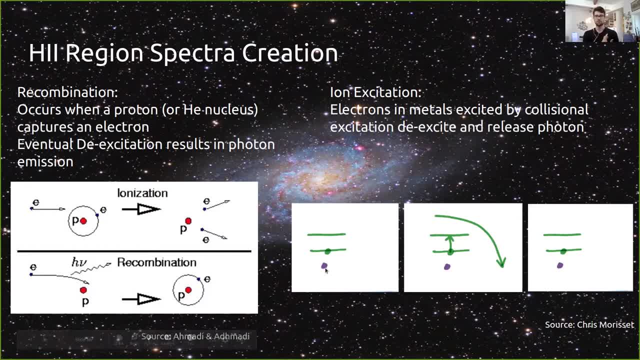 excitation works and the idea is here in purple. you have your. normally this is a metal nucleus. you have your metal nucleus or a metal atom that's missing an electron and there's a collision. so another electron passes very closely and 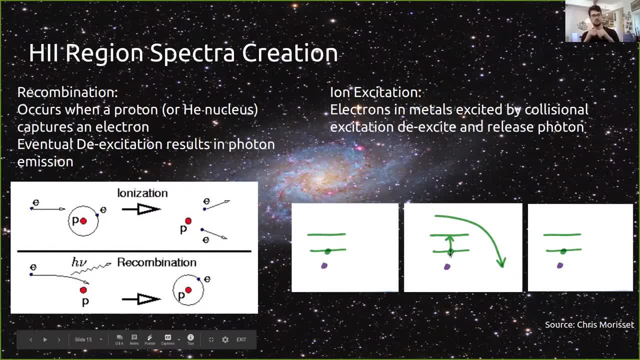 one of the electrons that's bound to the iron- or sorry, not iron, that's a common one, but it's bound to the metal. it jumps an electron state right, It gets energized and jumps a state. Well, eventually quantum mechanics tells us that it's going to jump back down. It wants to be at. 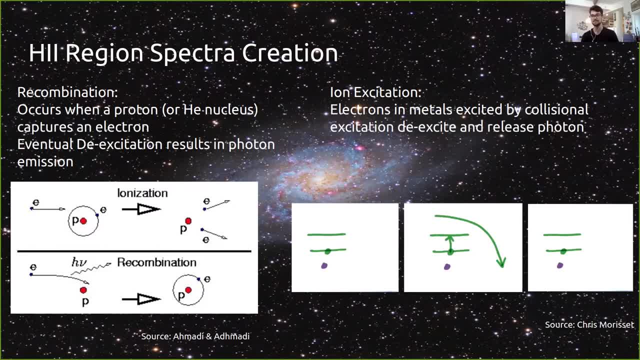 its lowest state possible. When it jumps back down, it again releases a photon. So those are two main methods for generating emission lines in nebulae. Okay, what do these H2 region spectra actually look like? I have two examples here, kind. 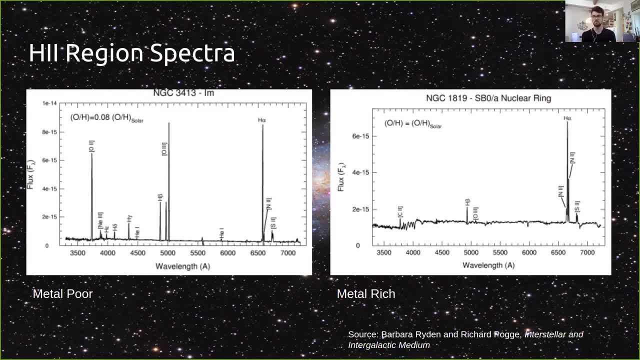 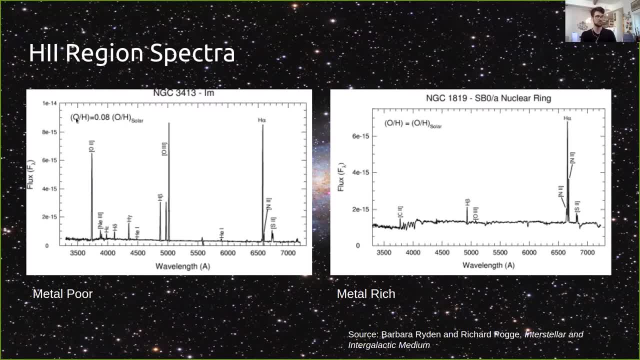 poor on the left. You see it's 0.08 solar O over H is a wonderful metallicity proxy. so oxygen or hydrogen Over here for the nuclear ring. you see that it is approximately solar level metallicity In both images. you probably. 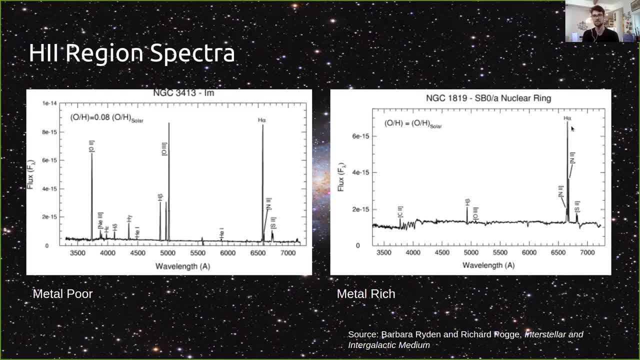 note that H alpha is your strongest line or one of your strongest lines. That's very common. Some of the most important lines are H alpha. You have this N2 called a doublet. There's actually two peaks to it, Nitrogen and sulfur. that's actually doublet hanging out there too Kind. 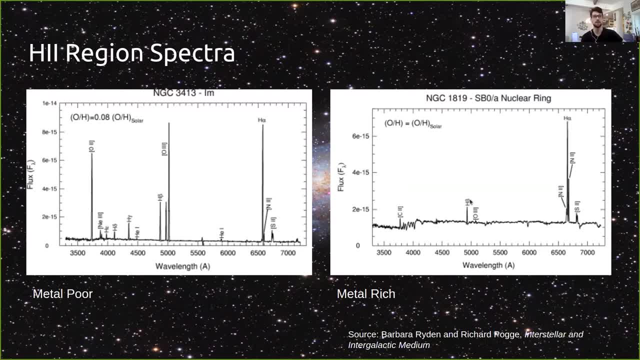 of hard to see. You have the other Balmer lines such as H, beta, H, gamma, H, delta, so on and so forth. They're over here. You get other important lines like helium And oftentimes metal poor. you can see strong oxygen lines. You might be thinking: well, it's metal poor. 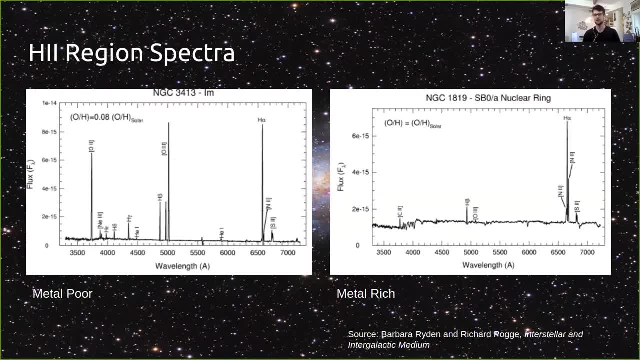 so why do I have so much? why am I seeing oxygen? that's a metal, especially an ionized metal. Unfortunately, it's not as simple as if you have a lot of oxygen, then you're going to be seeing a lot of oxygen lines. It really matters on the density of those metals within. 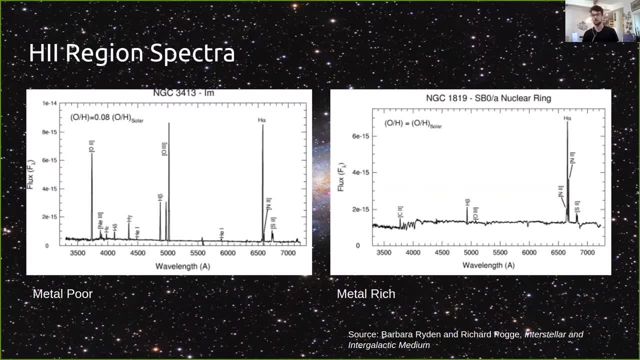 your nebula and the temperature of the central star or globular cluster. So it's not a simple linear relationship. It's actually rather complicated. There are a number of excellent papers on that, by the way, by Chris Morissette, and he uses some software that he has worked. 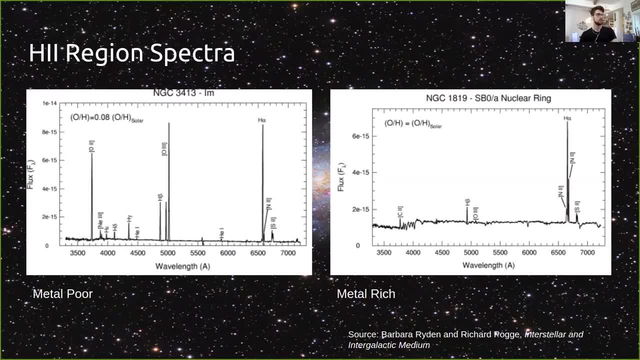 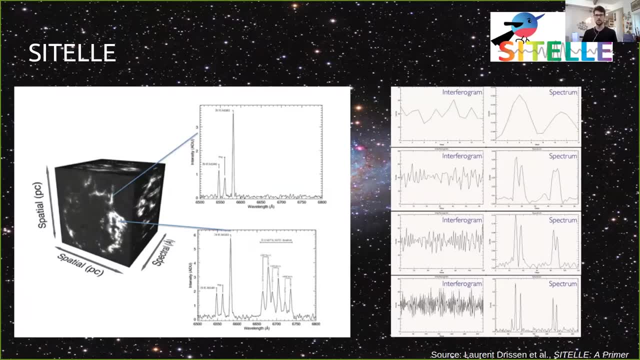 on developing called Cloudy. It's quite excellent. Okay, so now we have a basic idea of what happens with H2 regions, how they're ionized, what type of emission they might emit, how we would see it in the optical with H alpha. 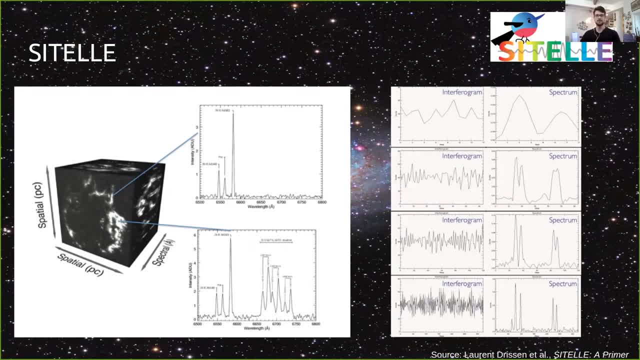 that N2 double it, S2 double it and some other pieces. So let's get over to some instrumentation. So this is the instrument Sattel. I don't have an image of it, so this is not actually Sattel, But Sattel is. if you are familiar with Nicholson interferometers, it is very similar to that, but it is not Sattel. It's a very similar instrument to the Sattel interferometer. So this is the instrument Sattel. I don't have an image of it, so this is not actually Sattel. 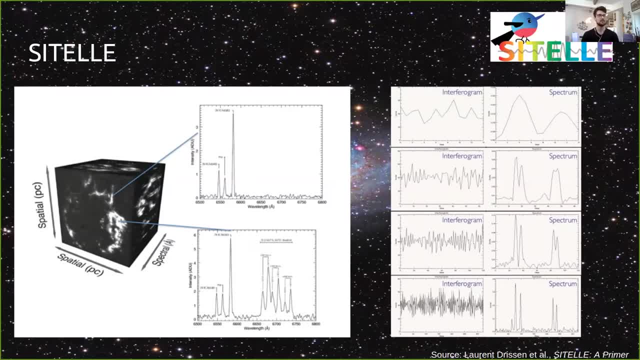 It's not the same thing. The base idea for Sattel is that it takes its samples. your wavelength takes an interferogram and then you can do a Fourier transform to pull out a spectra. And the power behind Sattel is that it doesn't just take a spectra for one. 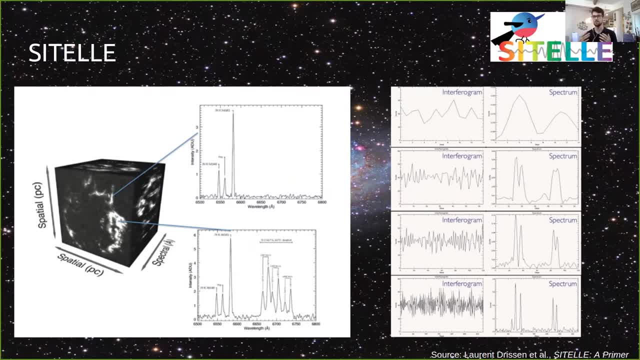 location or on one band. It actually takes a spectra at each point in its viewing. So here's what we call Sattel Data Cube. In the xy-axis, we have the spatial information. So here's the superlunar remnant, for example. You have the spatial information, so you have a really 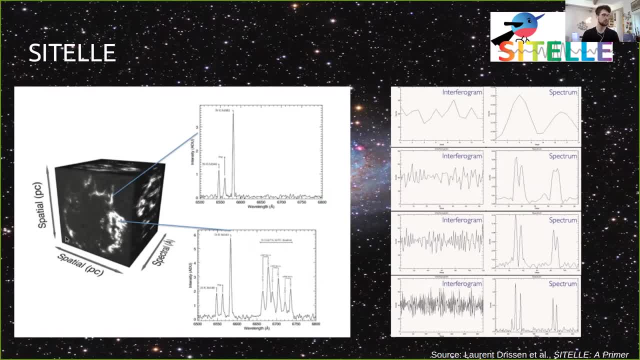 beautiful image of whatever you want to look at- in this case supernova remnant- but you also, at each one of those pixels, have the spectral information. So at each pixel, you have a spectra which is incredibly powerful: Sattel's spectral. 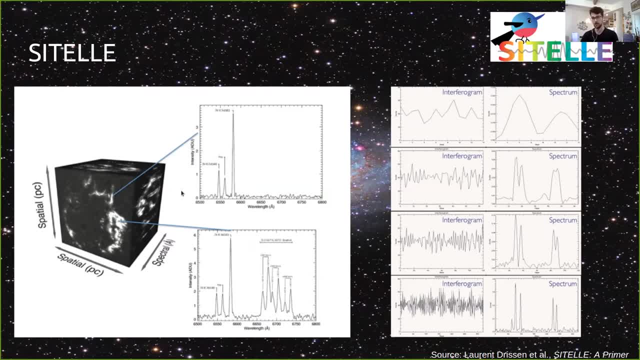 resolution goes anywhere from approximately 1 to 20,000.. The highest that's been used for observations is 7,000, and that's of the Perseus cluster And I actually have that data and it looks quite exquisite at 7,000,. but 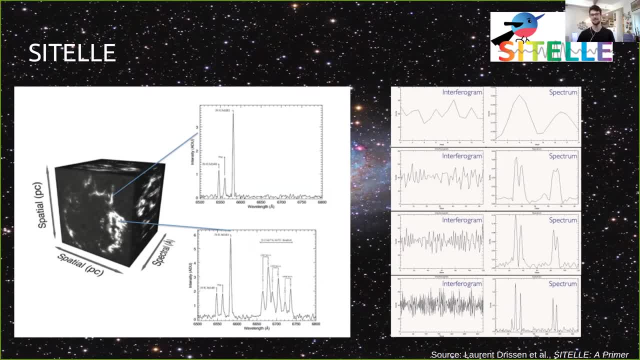 Sattel's real power comes from the fact that you're not just getting a spectra of a small region and you're not just getting the spatial information, but you're getting everything: getting the spatial information and the spectral information. So another important piece about Sattel, to kind of make it. 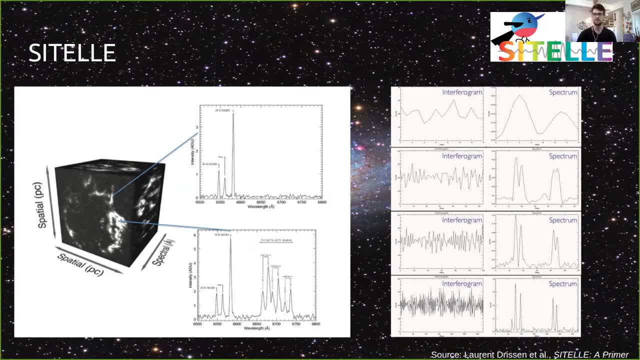 different and distinguish it from other IFUs such as Muse Sattel has an 11 by 11 arc minute field of view, which is huge. It is a very large field of view. It's a very large field of view. It's a very 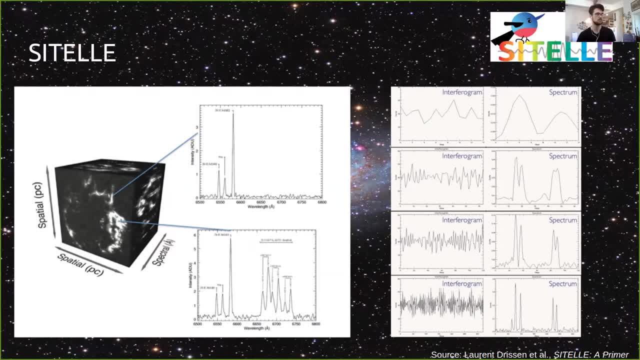 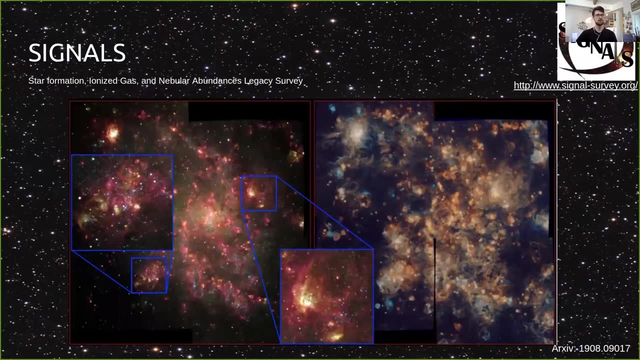 large field of view. It's by far the largest field of view for any IFU. IFU stands for Integral Field Unit. That is the type of instrument that takes the 3D cubes. This work is done as part of the SIGNALS collaboration. SIGNALS. 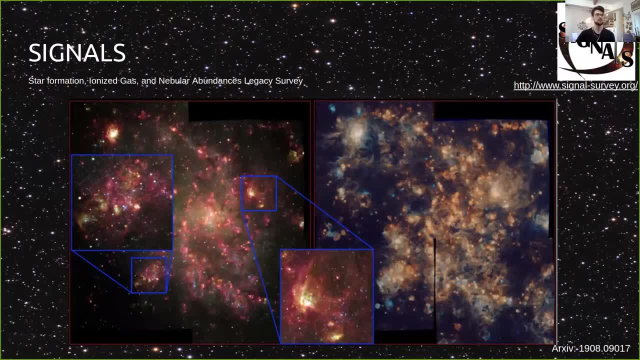 stands for Star Formation, Ionized Gas in Nebula Abundance's Legacy Survey. This is a multi-year, about six-year, program. They're on their third year at Sattel. It is taking a look at over 40 galaxies and expected to find over 40,000 each two regions Here. 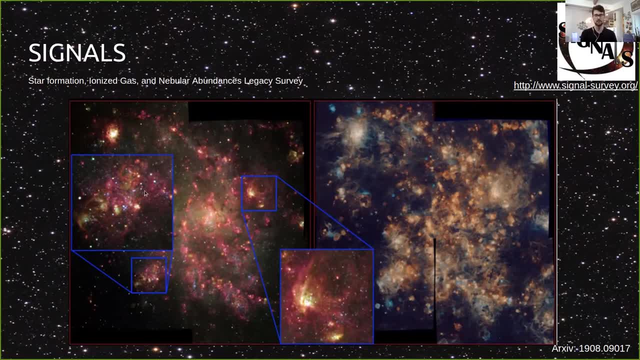 I have a image of M33, and you'll see why I chose M33 later. This is the central regions of M33, and then over here, this is the Sattel information from L33.. After the spectral analysis, each color represents a different type of. 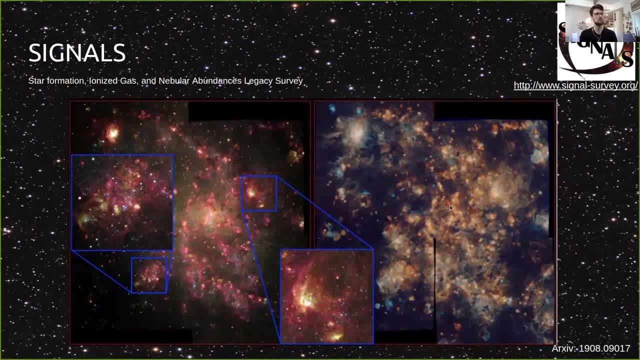 emission. If I remember correctly, blue is oxygen and orange is N2H alpha. So it's really fascinating type of information you can get from Sattel, And SIGNALS is led by Piyai-Lohi Kusonetan. She is the instrument. 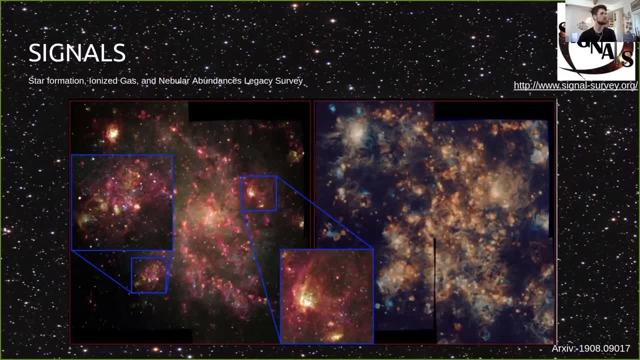 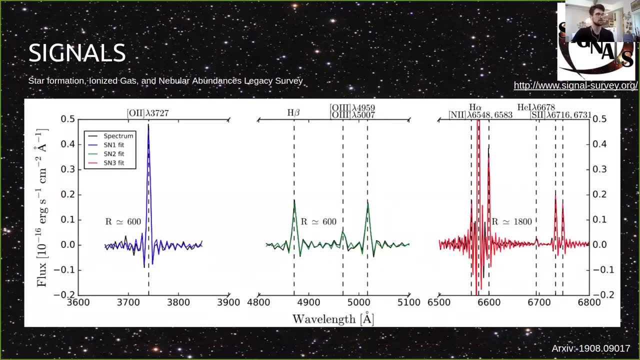 scientist for Sattel at this moment. So what kind of data are we looking at for SIGNALS? This was the test run for SIGNALS. Sattel looks in three main filters in the optical band. Here you can see the wavelengths. here The first. 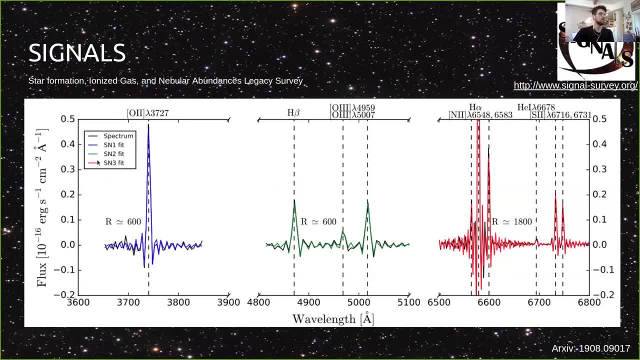 optical filter which is called SN1, and the first optical filter, which is called SN1,. one of the main things you're gonna pull out from SN1 is this O2 line. You have your second filter, SN2,- very original. You get this oxygen. that's. 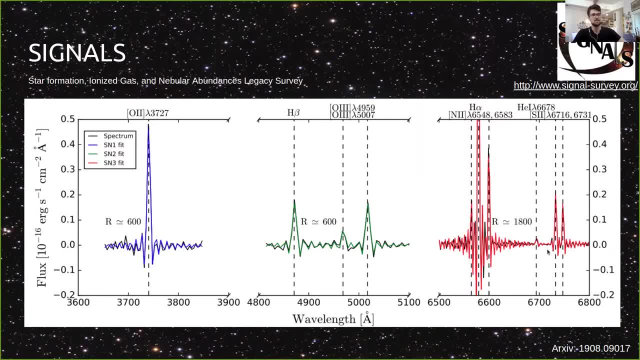 been excited three times: O3 and H beta, And then SN3, which is kind of the, the workhorse of Sattel. the main filter used gets your H alpha, this N2 doublet and your sulfur doublet, and sometimes helium-1 if you're very lucky. 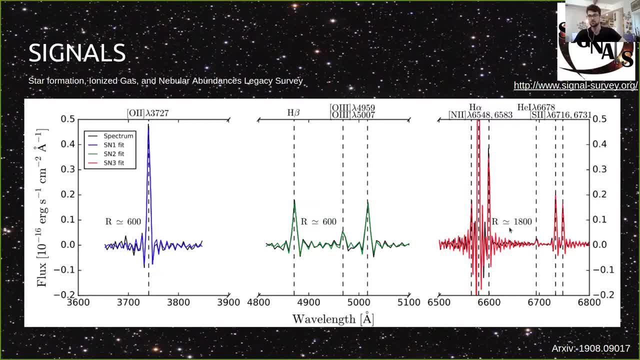 These are taken at two different spectral resolutions. lower spectral resolutions for SN1 and 2 because they're less crowded, It's easier to find the lines and then do flux calculations. for instance, This is at resolution 600 for SIGNALS, The actual program, the resolution, is 1000 for SN1. 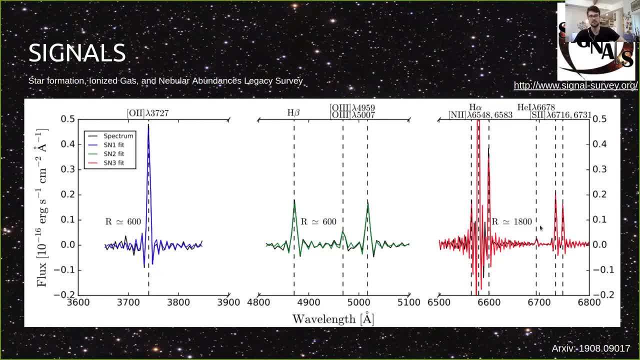 and SN2.. SN3 in this example is at 1800.. In reality, it is at 5000 for the SIGNALS program. So it's truly exquisite data that we're looking at, And I'll show you an example of what one of these SN1 and SN2 are. 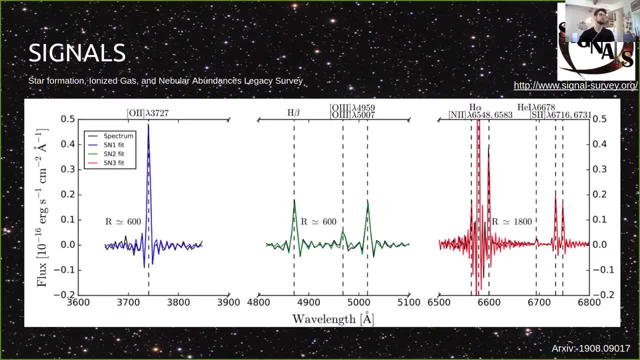 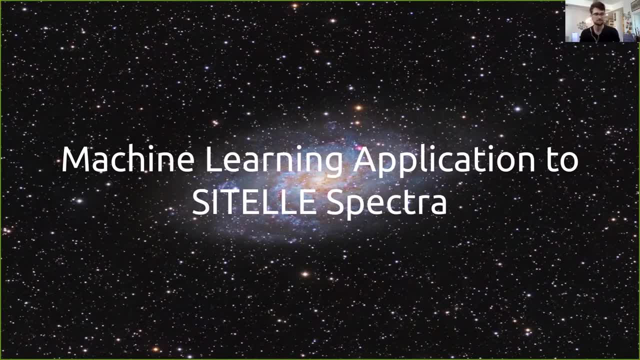 So this is what SN3 blocks look like- Great. So we've done our homework. We have the basic idea of neural networks and how convolutional neural networks work. We've seen H2 regions. We know how they're ionized. We kind of know what to. 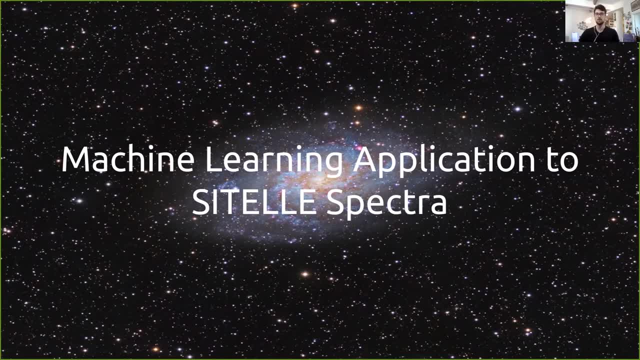 expect as far as their emissions go. And we know what Sattel is, We know how it works and we know what a normal Sattel spectrum might look like. So, for this work, what we are going to be doing is we are. 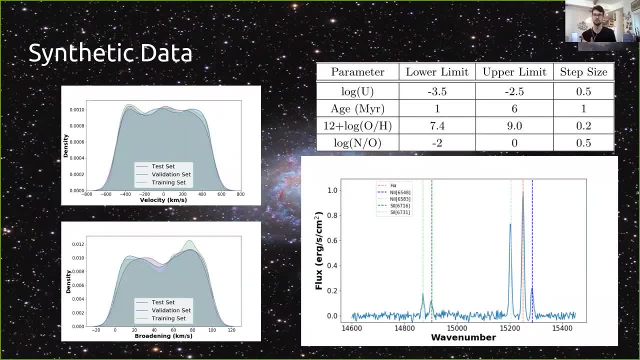 going to be taking those SN3 filters of Sattel. so the resolution 5000 with H alpha, your N2 doublet and your S2 doublet. We're going to take the vector of fluxes as our input and we're going to pass it through a convolutional neural network. 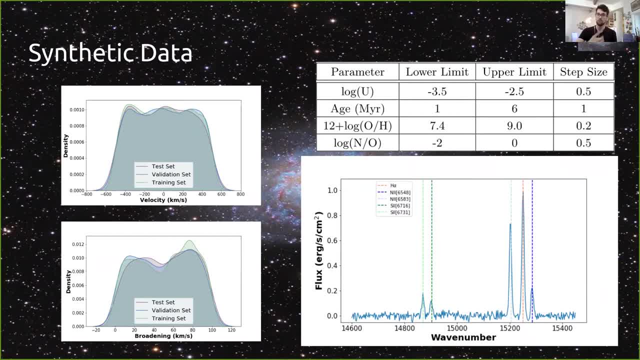 which I'll describe in a bit, And the idea is to output the velocity and broadening parameters that are associated with that gas, that cloud of dust or gas that's being ionized. These are two really important parameters for a number of reasons. One, it's the kinematics of those H2 regions. 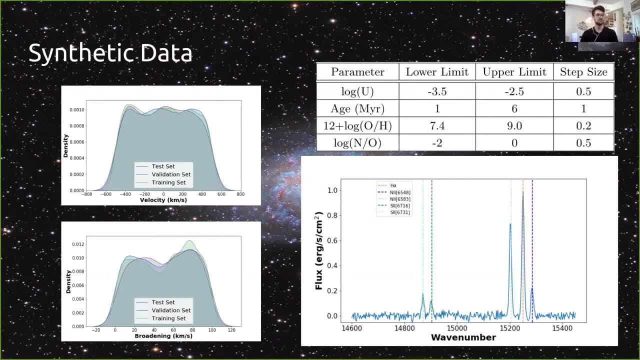 Which is incredibly important. Also, there is a wonderful software called Orcs that is used for Sattel data analysis. There is one pitfall of Orcs, and that is that you have to input an initial guess for velocity and broadening. If they are terribly wrong, you will get horrible fits. So this also. 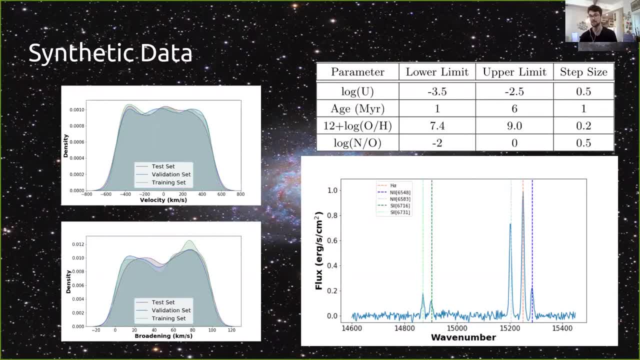 goes around that problem and helps you get good initial guesses, And I'll also mention that it is being changed a little bit to be the normal implementation in Orcs. So it's this machine learning problem. For everybody who's done machine learning, you know that the most important part of machine learning is your input set and 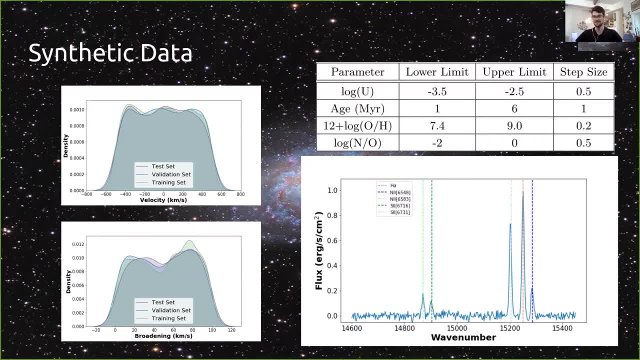 really your training set. If you don't have a good training set, garbage in, garbage out, You're not going to get anything meaningful out. So what we did is we created a set of synthetic SN3, so that third filter of Sattel. Here is an. 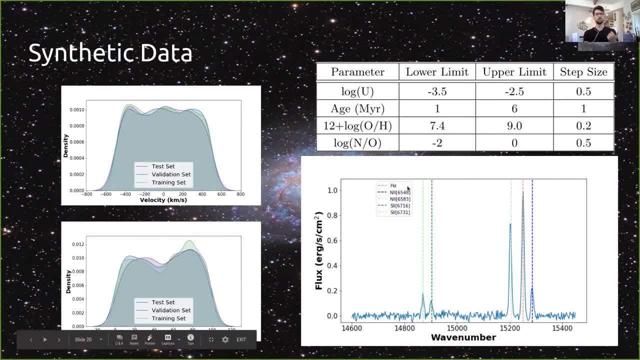 example, here We modeled the H-alpha, N2W and S2W emission, added them up and added some noise. How did we come up with these amplitudes that we used? Well, we used the bond calculate, bond survey and bond calculations. It's a really wonderful survey and a really wonderful. 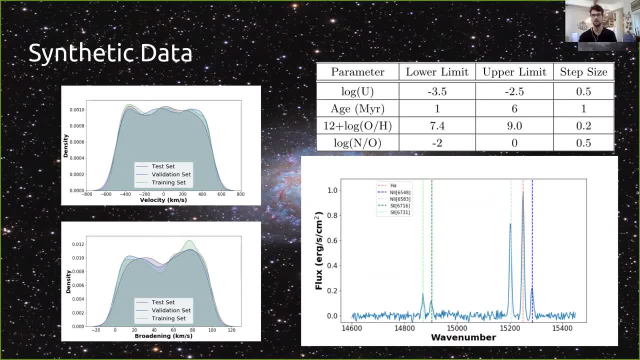 set of calculations that are done using Cloudy that are available on the 3MDD database. It's the Million Mexican Model database handled by Christoph Moisette. Here are some of the parameters, If you're interested. I'm not going to go. 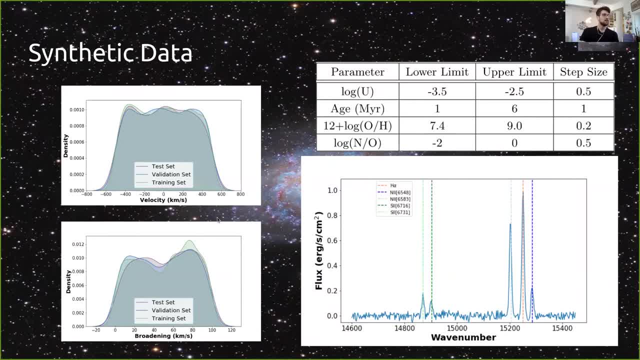 into those, but you can find them in the description If you're interested. I'm not going to go into those, but you can find them more in the paper. And next, we wanted to make sure that our data was, or that our 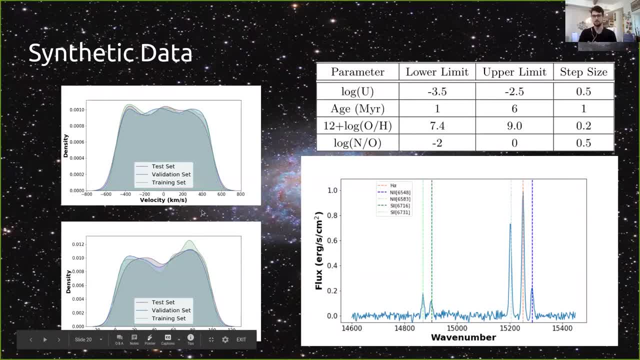 training set was pretty well broken down into different velocities and different broadening Right. If we want to train our algorithm to pick out the velocity and broadening parameters, we want to make sure that we have a good amount of broadening velocity parameters that it's learning from. You can see here that 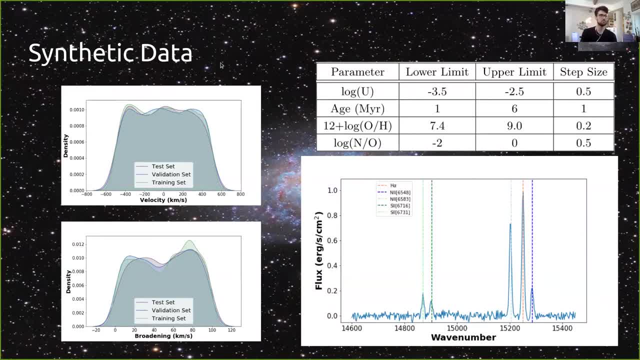 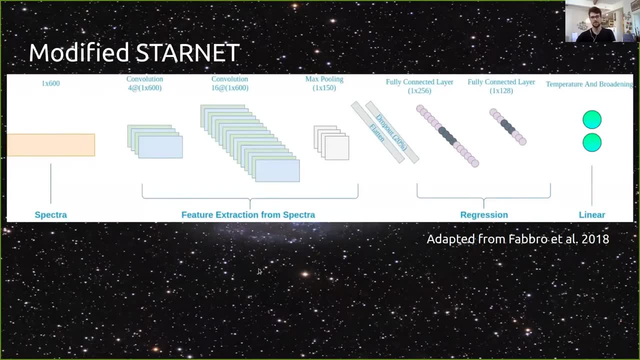 everything's pretty even. We have a good number of broadening and velocity parameters, and the test, validation and training set are all relatively homogenous. in that regard, The convolutional neural network that we use here is absolutely not my own. This is taken from Fabro et al 2018.. Thank you, Sebastian, And the idea is we start off. 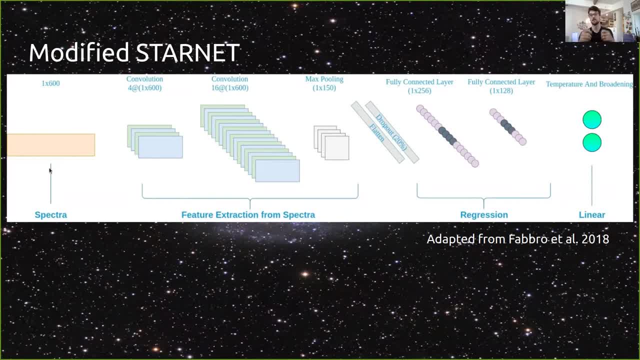 with our spectra, That is our. it's not an image of a spectra, just to be clear. This is the vector of amplitudes for our spectrum, for SN3 spectra, We run it through two layers of convolution. The first layer is just to pull out the main. 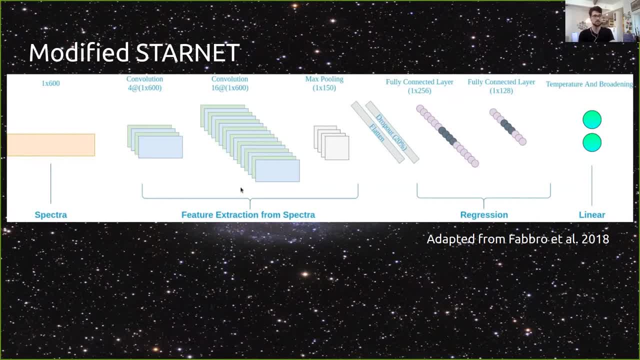 features. and the second layer is to pull out some of the more fine structure in the spectra And then we pool it to. we just use max pooling to downsample a little bit and make the input smaller. It's that feature extraction or the 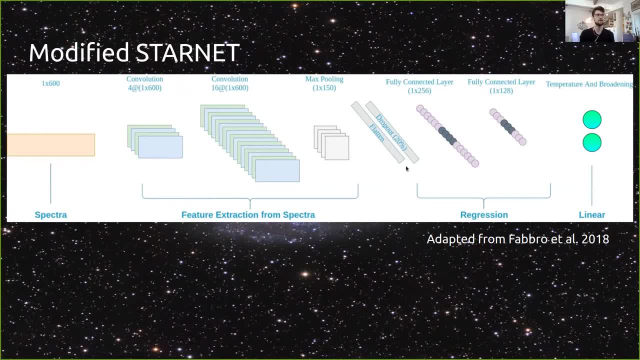 convolutional step of a convolutional neural network. We then need to flatten it. That's just a neural network fun part. You have to have it as input vector When you do something called dropout. dropout is a way that you can get around. 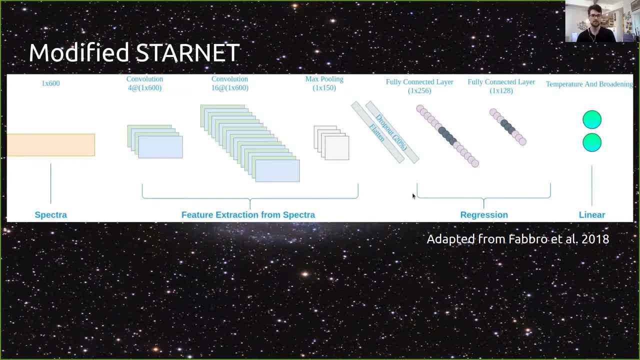 overfitting, which means if you're overfitting, that means your network is learning your training set really well but will not generalize to other things at all. So one way to get around that is adding a dropout layer, and a dropout layer means you're randomly throwing away pieces of input. so your network 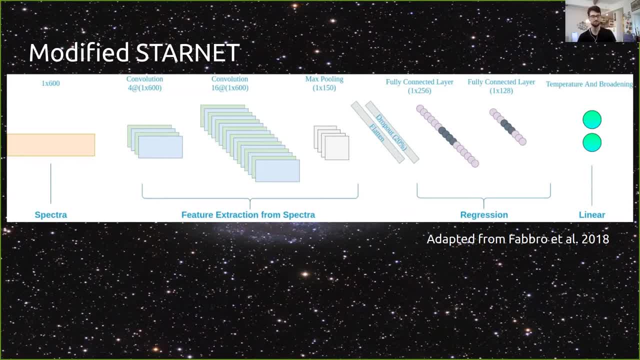 doesn't learn from those pieces of input, and that actually changes each iteration. Then we have our two fully connected layers. First one contains 256 nodes, second, 128 nodes, not super important, but that's our neural network step. This is a regressional problem. so, finally, we're going to be calculating our 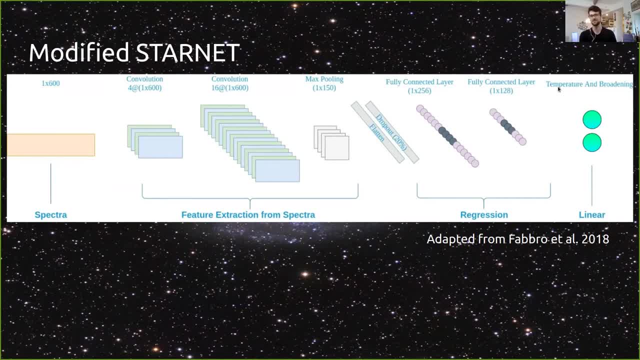 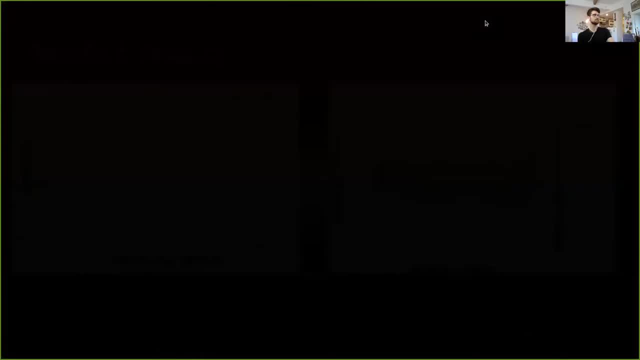 velocity and broadening. Forgot to change that typo. it should say velocity, not temperature. and we use linear activation function to determine your broadening, your velocity. So how does this look? when we do it, We have our set of, we have our 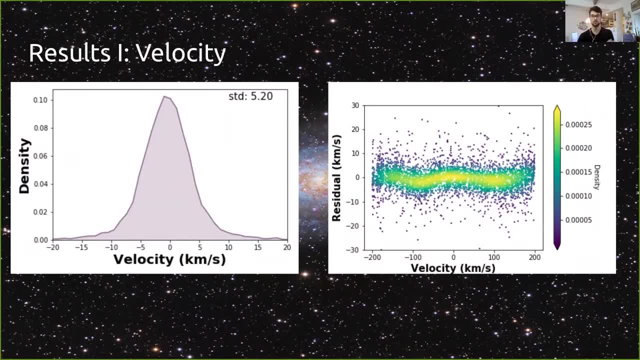 training set. we train our convolutional network that I just showed. By the way, the training set has about 24,000 mock spectra that we've created. We train our network that we're happy with it and then we apply our test set. 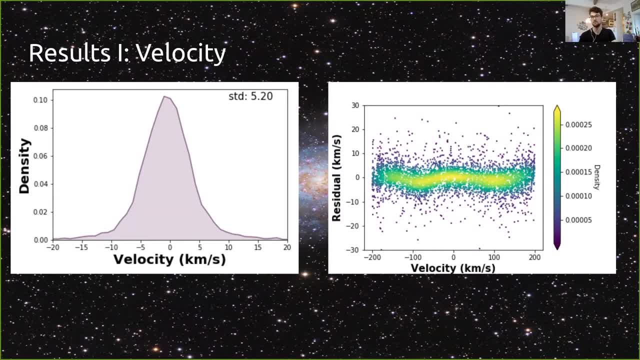 Our test set is 3000 of those spectra that we held off that. the neural network has never seen our test set. That's the whole point. it has no idea of what it looks like. after we train it, Then we give it to them and see how well do they do, or how well does it do, how well? 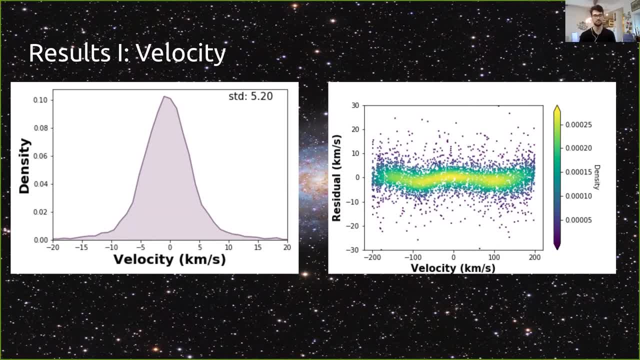 does our neural network recover the base parameters from our test set 일이 and and once again al test. that is more synthetic data. So what we see for the velocity- we're incredibly happy with the velocity You can see here. here is a residual density. 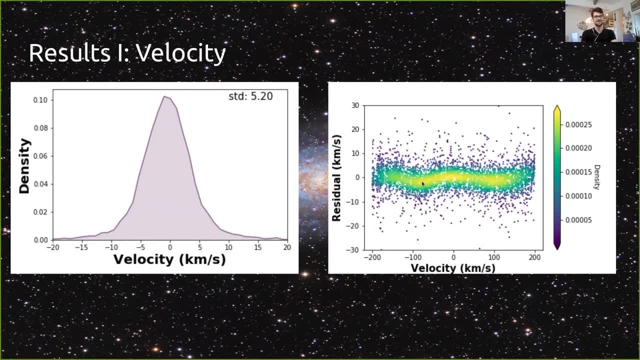 plot. So this yellow means higher density of those residuals over a set of velocity parameters. This is your velocity, which means the residuals are low. You can see here this is a residual density plot. So it's basically the errors on your velocity, with the standard deviation of approximately five kilometers per second. 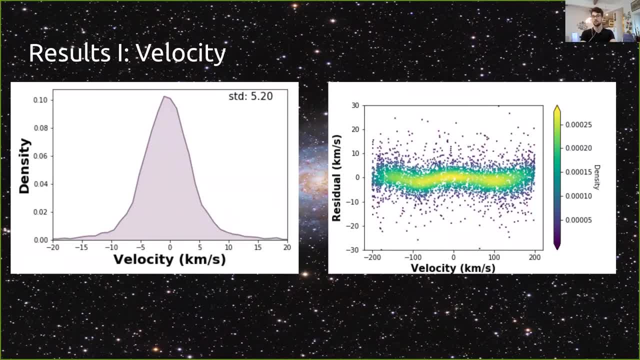 which is very good, very comparable, In fact. ORCS gets about three kilometers per second if you have the perfect guesses for everything, and everything's set up wonderfully. So it's very comparable to the main fitting algorithms used for SICL data cubes. Roddening is admittedly a little bit. 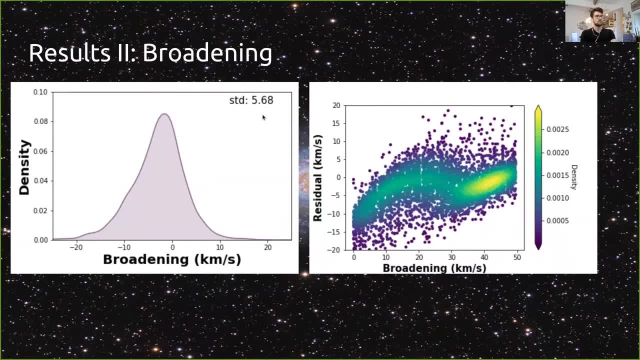 worse, The standard deviation drops or actually increases to about 5.7 kilometers per second. We can see here, and this is mainly why there's this large tail, So this is a large tail For low broadening. at high broadening parameters. we're doing a pretty good job. 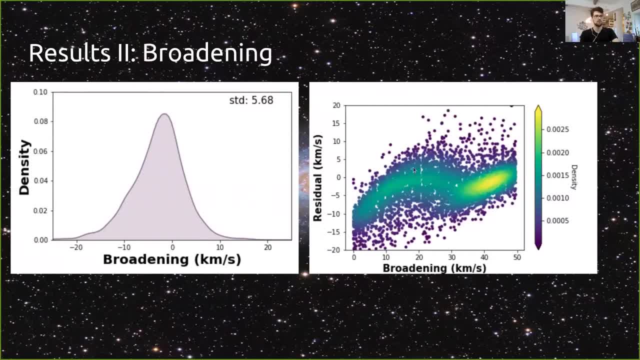 You can see, this yellow region's really around zero, But really above 20, we start really below 20,. we're not doing too well, Or we? this is something that we will probably be looking at additionally later, But one of the main reasons is: 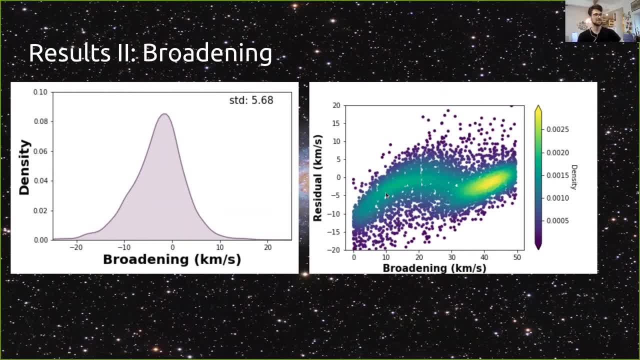 likely how to put this. it's likely tied to our training set something wrong with the broadening. It's also potentially an issue with SITEL. SITEL, even at high resolution, actually can't distinguish broadening parameters lower than approximately 14 kilometers per second. 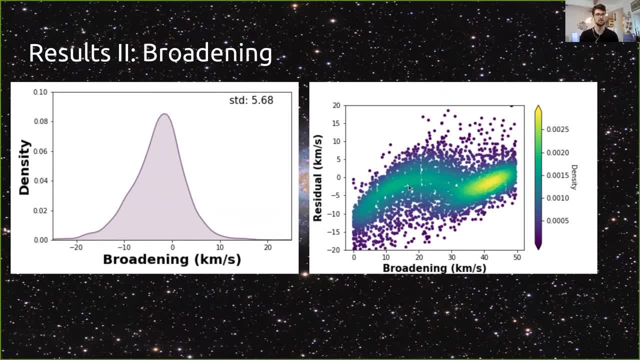 So, as far as SITEL data goes, we're really right about here, and that's when we start to see some pretty good results in our broadening parameter estimations. Great, We've tested it, We've trained our network, We've tested our. 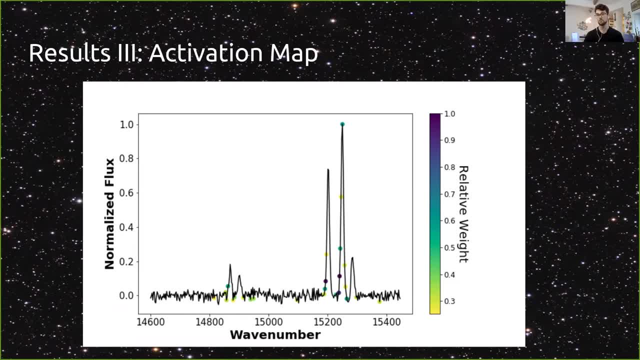 network. The network shows us that we're doing pretty well, Certainly comparable, a little worse, but comparable to the main fitting techniques. But we kind of need a sanity check at this point. How do we know that our network's actually learning the? 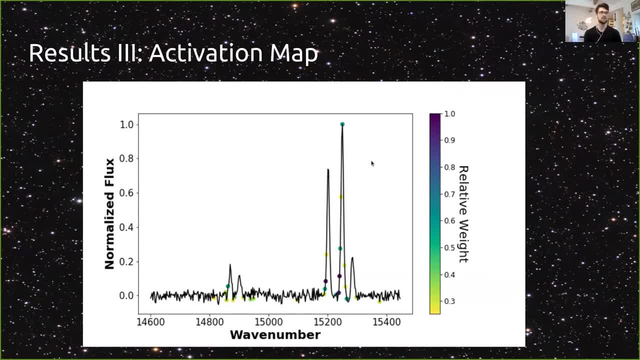 important pieces that we want it to learn Meaning. how do we know that it's looking at that H alpha line, the N2 doublet and the S2 doublet, and learning from the structure of those and the related structure of those, how the 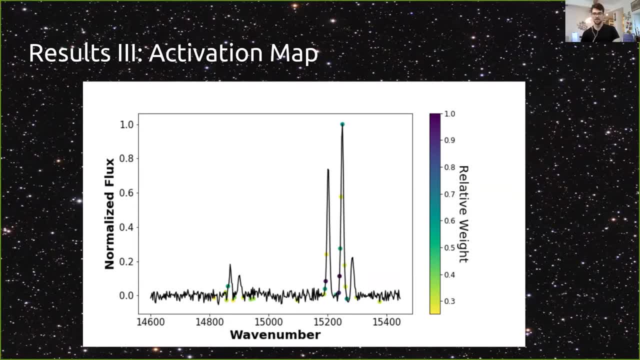 broadening and velocity parameters are going to be changing. What we did is we created an activation map. An activation map looks at how your inputs affect your output. So basically it's telling you what's important in your input for the input, And we see here what the relative weights in this activation map that the 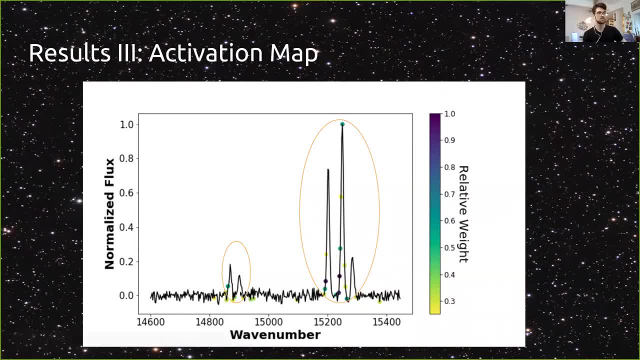 weights are centered on the H, alpha and N2 emission and also your S2 emission, which is perfect. That's just a sanity check to make sure that our neural network's not learning from all this noise in between those peaks, but is really focusing on those peaks. 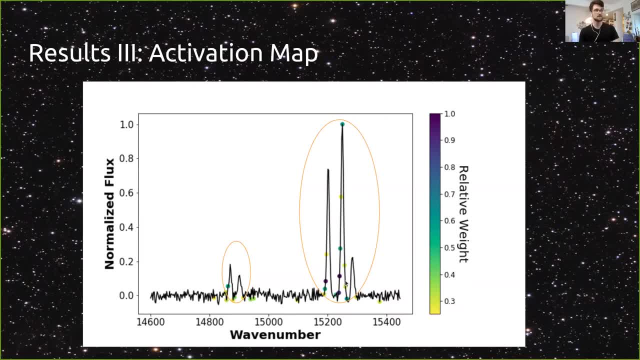 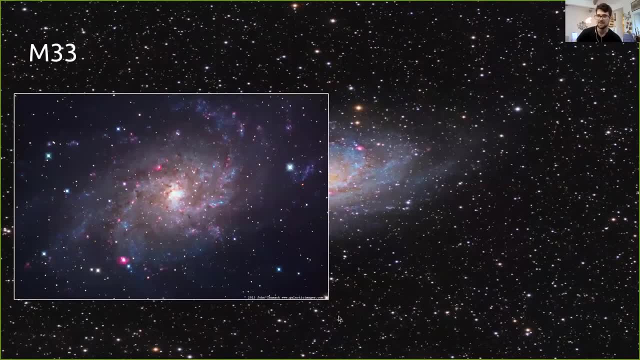 Not just the peaks, but also the area in between the immediate peaks. Great, So it works. We feel comfortable that it's looking at something that it's supposed to, and the input vectors. We trained it and we know it works well in test data. but how about real data? 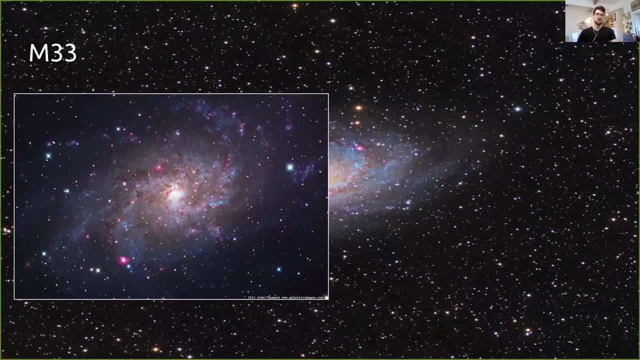 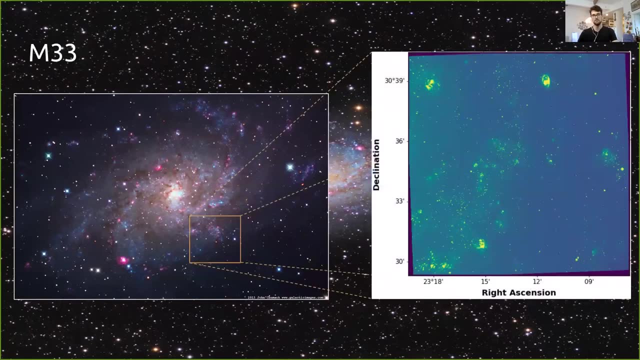 That's always a little different. So we took a Sattel cube from the signal survey. This is N33 and this is called the seventh field of N33.. You can blame Laurie for the naming of that, but this is what the deep image of Sattel looks like. 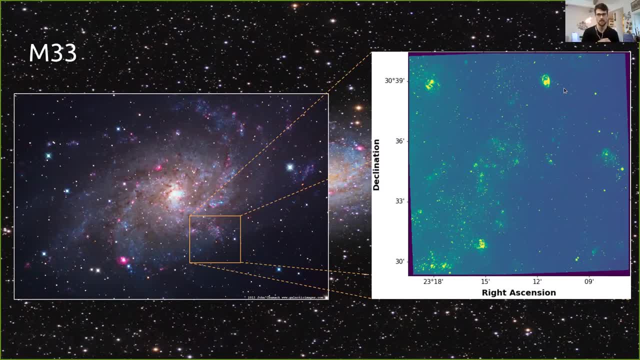 So if you take that data cube and compress it, so no more spectra- this is what it would look like. You can see that there are a lot of different H2 regions here, not necessarily classical H2 regions like you have here, but you also have supernova remnants and planetary nebulae. 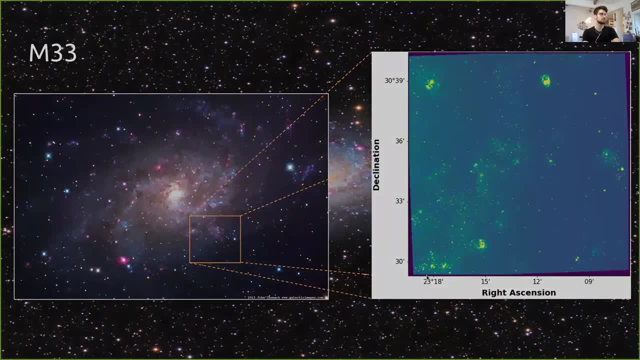 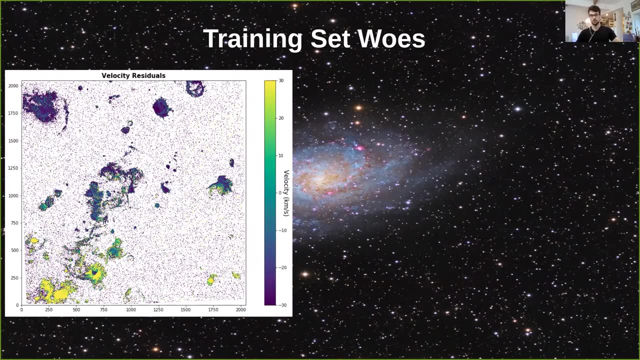 So we applied our neural network to the spectra at each pixel in the Sattel cube right. Each pixel has a spectrum, so we apply those to our neural network And what do we see? These are the velocity residuals. We see that they're not. 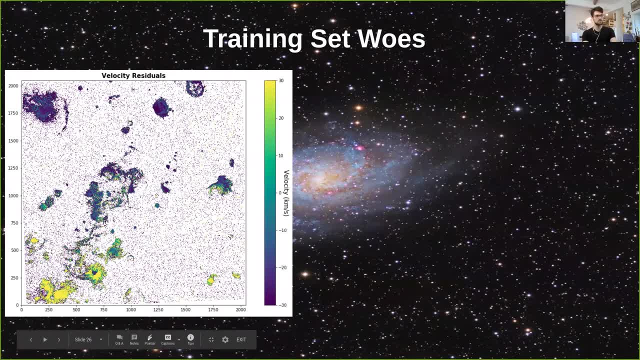 terrible. but there is an obvious systematic structure in the residuals, where at the bottom it's overestimating, near the middle it's doing a really good job getting the right value and at the top it's not doing such a good job. And I'll also mention that these residuals are calculated. 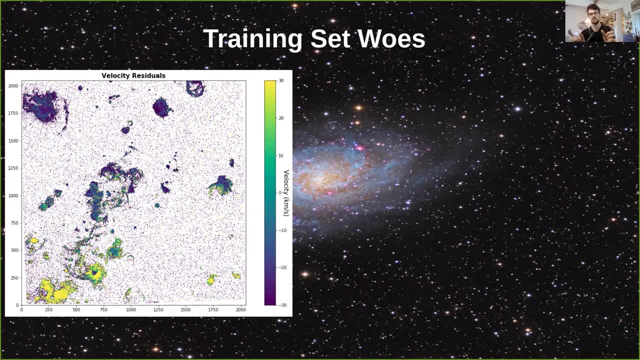 as the difference between our neural network and the standard fitting procedures for Sattel. Well, there's a fun thing about Sattel- and I'm only mentioning this because everybody who does machine learning gets really excited. but you're going to have a lot of fun with it, So I'm going. 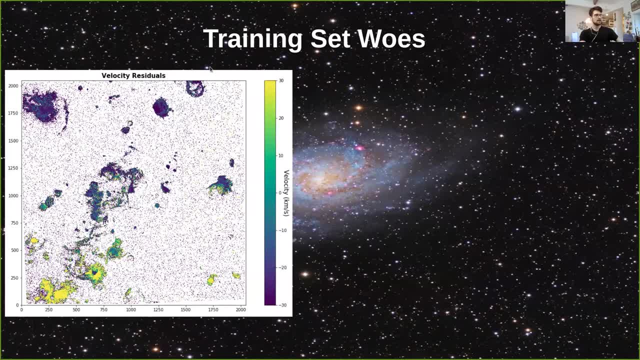 to talk a little bit about Sattel. You have to remember if your training set's not perfect, you're going to have some problems. The Sattel resolution is not actually constant. It changes a little bit as you move from the bottom of the cube to the top of the cube. We sampled. 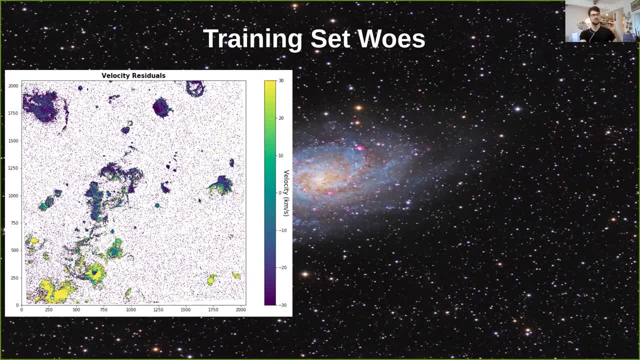 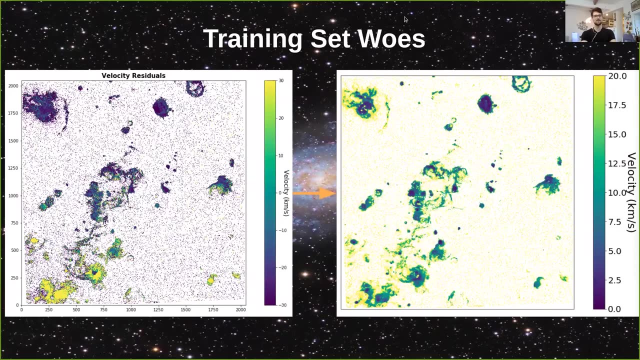 from the center. so we sampled that resolution of 5,000 from the center. So we actually had to go back and retrain our network on data that has varying resolution around 5,000.. What happens when we do that? Things get taken care of when we do that. When we do that. 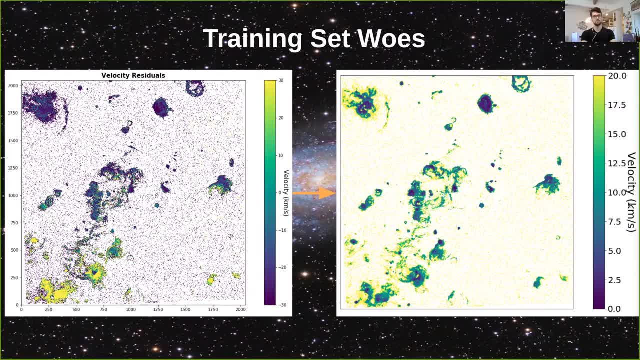 we no longer have the systematic, and you can see that now our velocity residuals are much lower in regions of strong signal-to-noise, so where there's a lot of data and a lot of flux, which is wonderful. So this is showing us that, yes, we can actually use our neural network now. 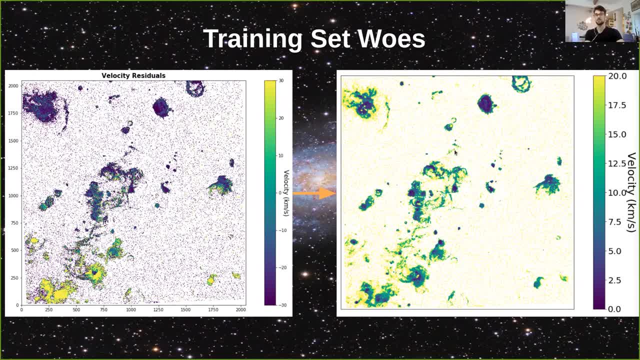 for real Sattel data to get these velocity and broadening estimates. These are the final maps for velocity and broadening. You'll notice that, once again, broadening isn't doing quite as well as the velocity is doing. There's some known systematics that we discuss in the paper. It's mainly due to the fact 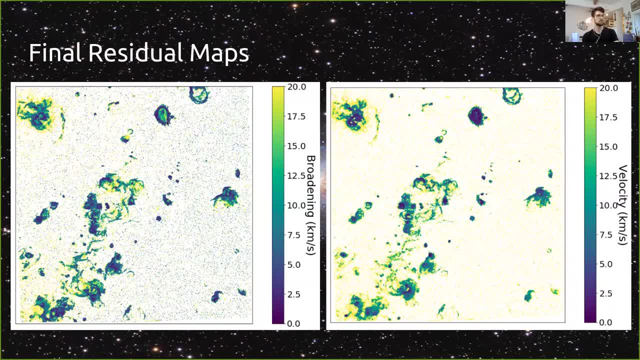 that we believe there are multiple network, wasn't trained with those, so it's not going to be able to handle that. Once again, it's in the paper or you can ask me after this if you want more information. But these are final broadening in velocity residual maps. 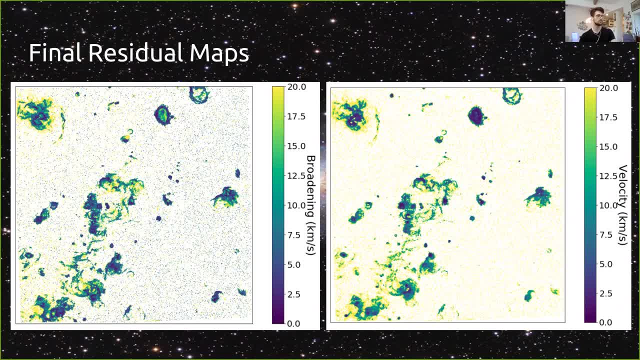 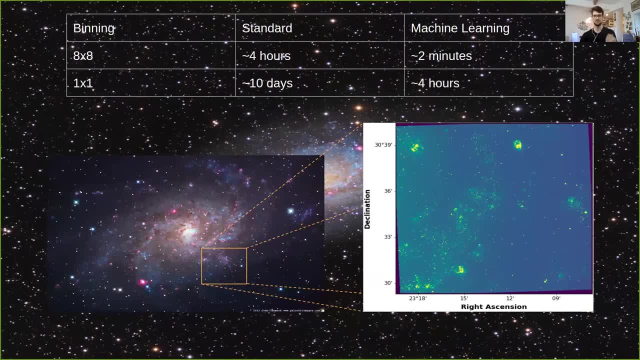 for that M33 field of our Sattel cube. Okay, so we have a neural network method that we've tested. It works well on synthetic data and it works well on real data. But why would we use this over the normal fitting procedures? Well, two reasons. One, like I mentioned, ORCS. 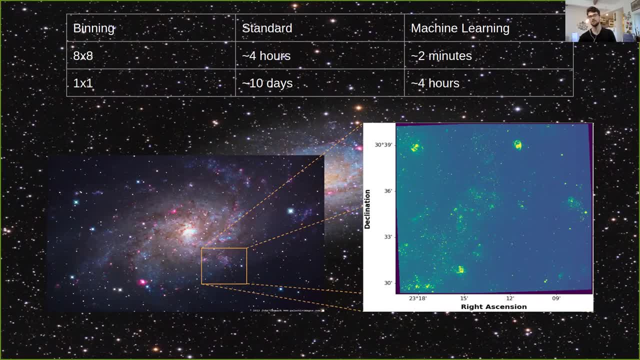 the standard fitting procedure requires you to have broadening velocity estimates that are good. This will give you your good broadening velocity estimates. Otherwise it's truly a wild guess that you have to make and see until you get it right. The other main benefit is the time reduction. 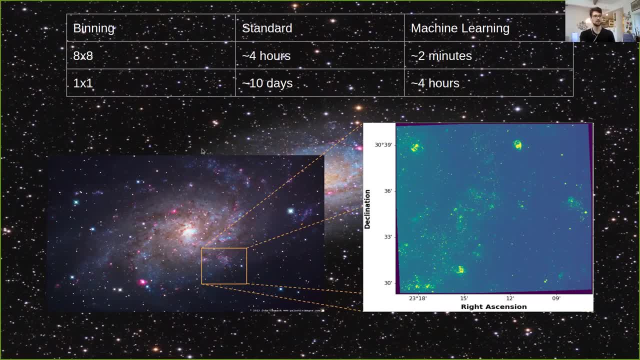 Machine learning is wonderful for bringing down the calculation time. Sattel has approximately 4 million pixels. It's about 2,000 by 2,000.. So you have a total of 4 million pixels and you have, in this case, a resolution 5,000. 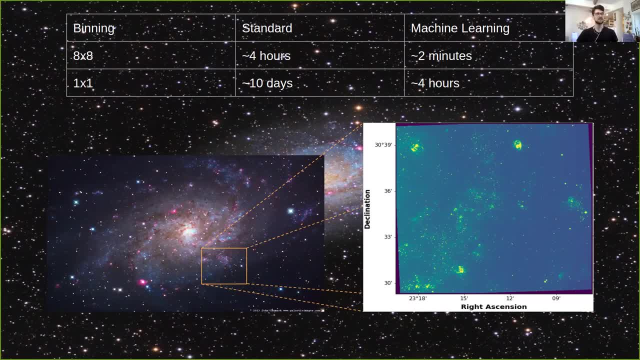 spectra at each one of those pixels. As you can imagine, that takes an incredible amount of time. Even if you bin the pixels at eight by eight regions, it takes approximately four hours on one of the computing clusters at Can-France-Y telescope. The machine learning algorithm. 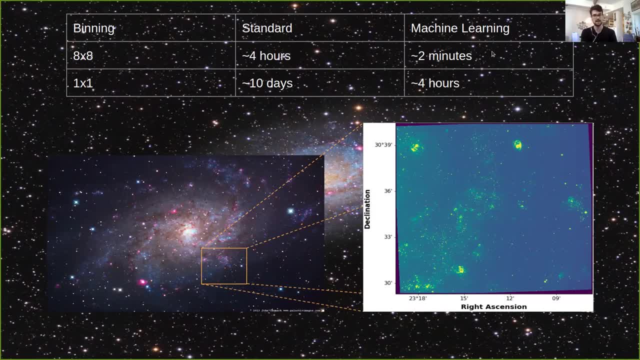 on the other hand, takes only two minutes to do that exact same region. So if we don't bin it and just look at the raw Sattel image, raw Sattel cube- it takes approximately 10 days to fit that entire cube using standard methods. Using machine learning algorithm takes 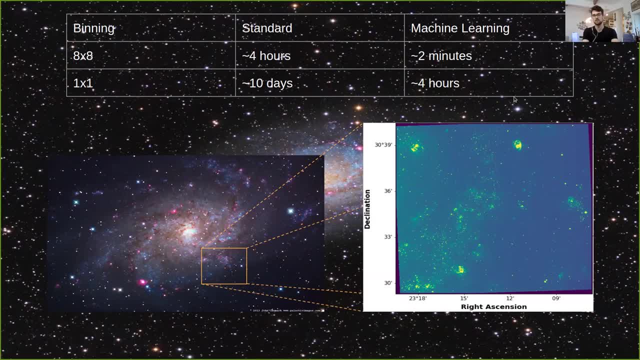 less than four hours. And these are the calculations, unparallelized. The normal code is that the standard methods are parallelized and machine learning. it is parallelized but I'm giving the unparallelized hours And it reduces linearly. So if you have two cores it'll take. 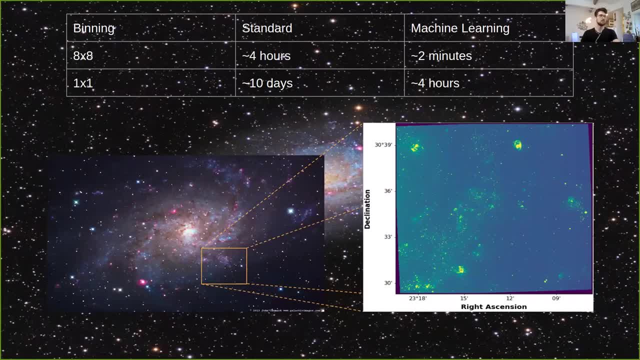 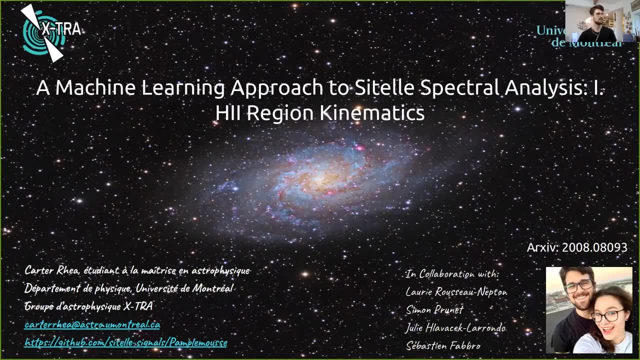 half the time, so on and so forth approximately. Okay, so a little bit of an abrupt ending there, but that is our first step at a machine learning approach to Sattel spectral analysis. As I mentioned, this paper was just accepted to Astrophysical Journals. You can find it there. 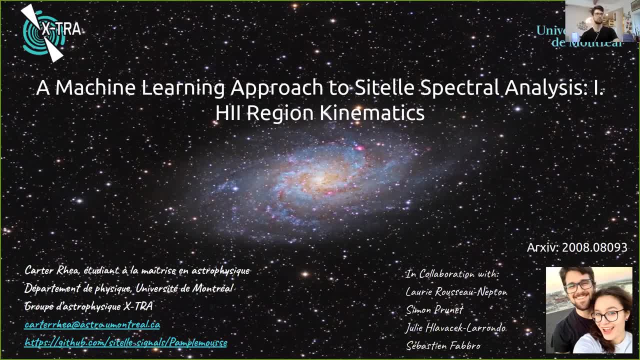 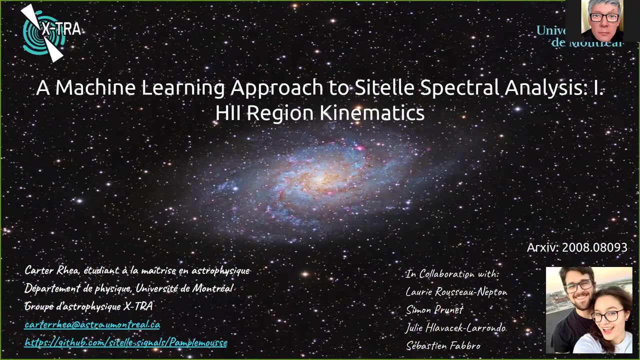 in the archive and we will be working on some more papers applying machine learning to Sattel spectra. That's it for me, And if there are any questions, I would love to take them. Thank you, Carter, Very nice presentation. Oh, you led us through the whole path of. 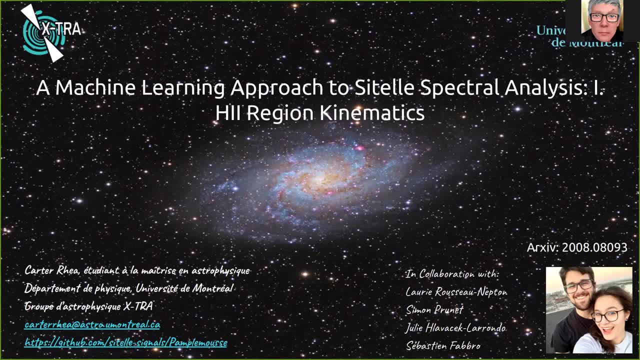 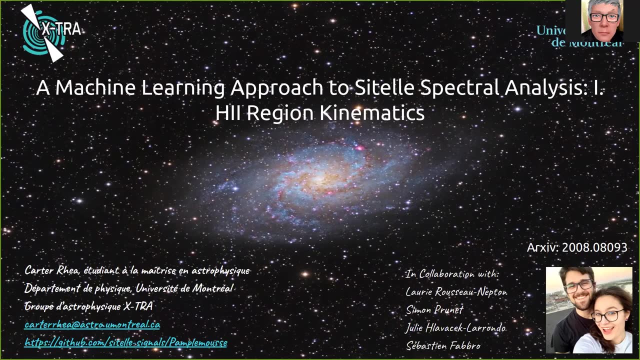 things and how machine learning works and then through the actual science and getting some results out from Sattel. So if you have questions, you can just raise your hand in the comment section and I'll ask them, and then you can just put them in the chat or in the 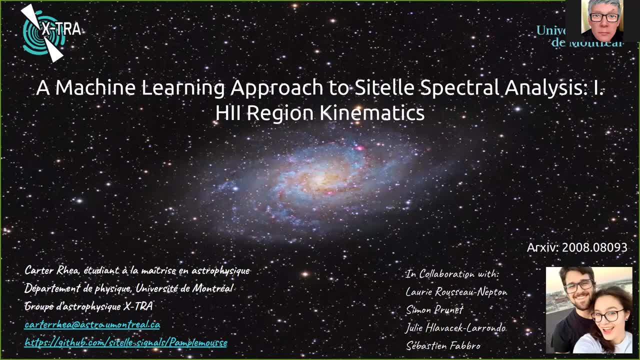 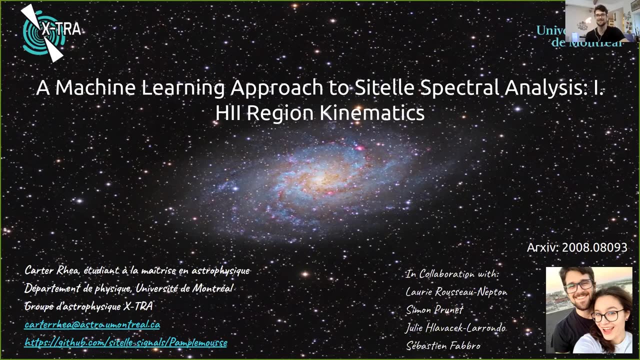 chat- chat window. Type them in the chat window. Either way will work. So a question I have is how many Sattel data cubes will signals end up with? I think right now they're shooting for 50.. No, 60. Sorry, they're shooting for 60. So this is. 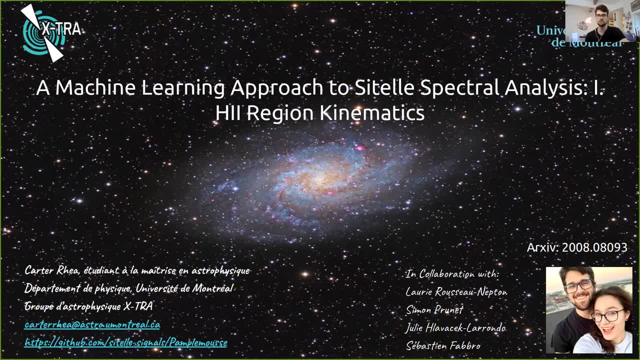 going to be really helpful on getting velocity and broadening for those 60 data cubes rapidly. Right now they we have approximately 30 of it And I should mention I'm part of the signal research team collaboration. yeah, okay, blake, you have a question? go ahead. uh, yeah, thanks for the great talk, carter. 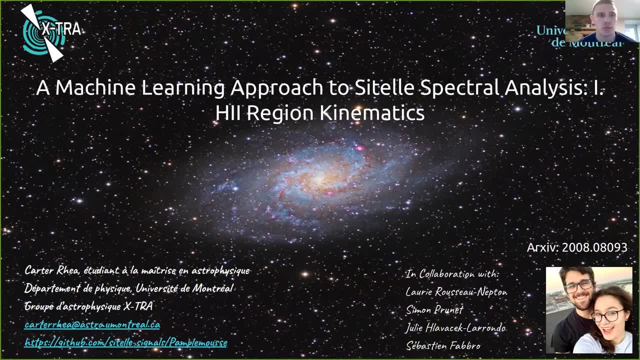 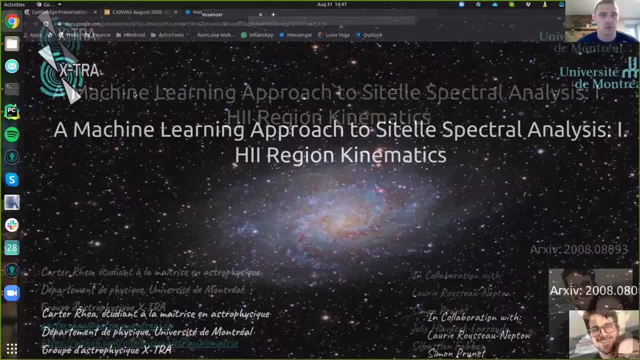 uh, it's good to see your research. um, i had a question about kind of at the start, when you were talking about the neural networks and you had that step where you're including the weights and and plus or minus some bias, um what would be like an observational bias that you would be 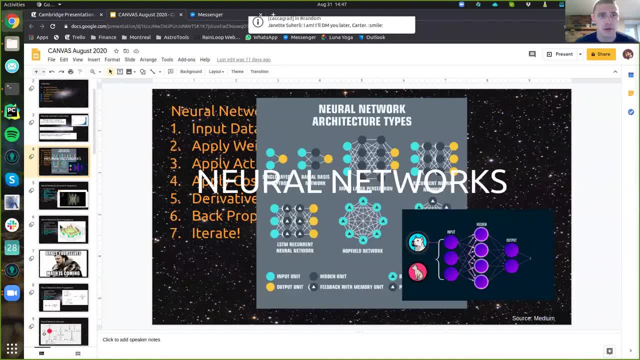 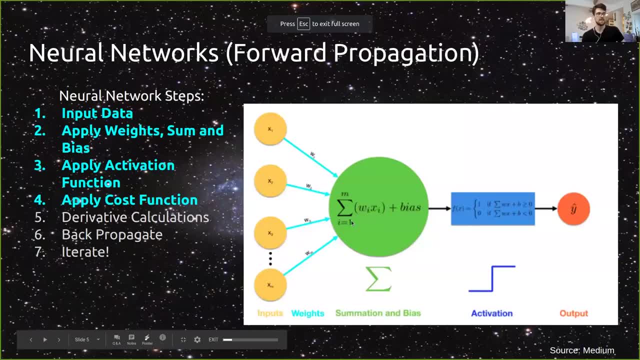 like a real life bias that you could be including at that step um when you're changing your weights. yes, so normally the bias is actually just a numerical um artifact that we'll be adding to shift the node value um. i don't know uses of. i know you can use real biases from systematics. 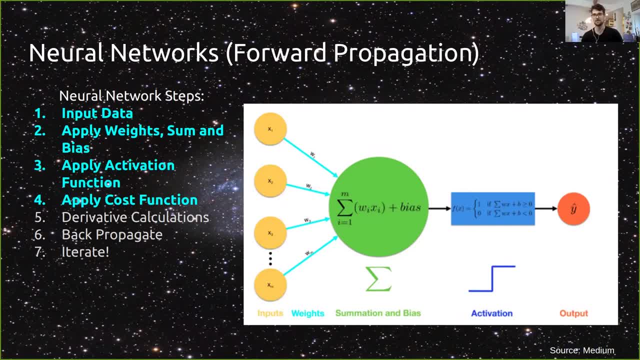 i haven't seen much of that incorporated into neural networks. um, with my little archive plot, you saw that neural networks in astronomy are really or. machine learning in astronomy is really starting to blow up and i think we're going to see that introduction of systematics more into. 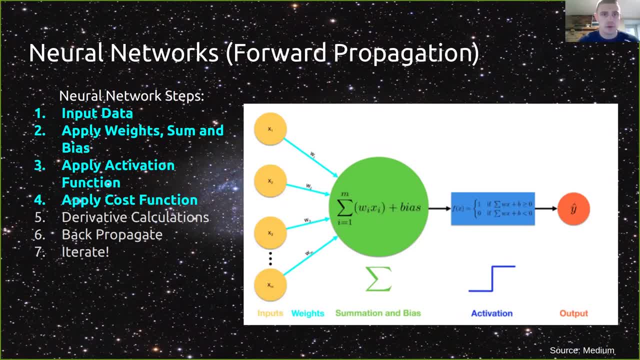 the networks themselves at a later point. yeah, the idea is right now. you want to take care of the systematics in the pre-processing of your test set their training set as best as possible. yeah, cool, all right, thanks, thank you, james. you have a question? yes, uh, hi carter. uh, that was a really nice talk, thank you. 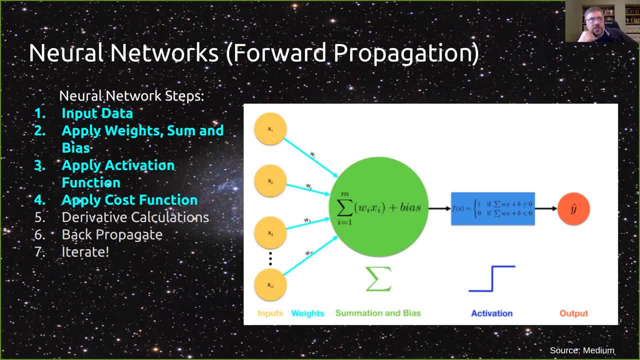 very much for sharing with us today. um so my question is regard with the, the method that you've used here. um so, um, i'm not sure if you're aware, but i have a. i had a student named jared cowan who also developed a convolutional neural network for determining the kinematics of gas. um, and in his case it was for. 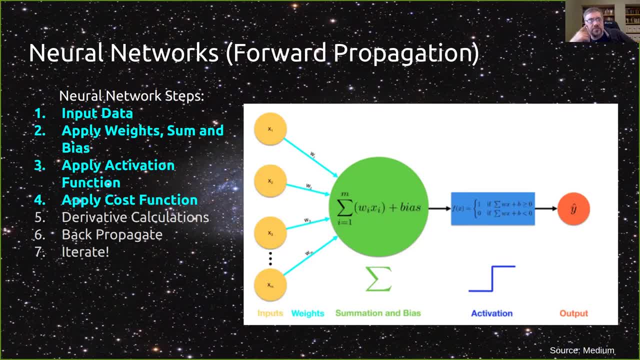 um gbt data, that we obtained, um of ammonia, and that was that paper and we discuss it actually in ours. um. okay, i just wondered, could you, could you elaborate a bit about the differences between what you've done here and what my student did um for his time? what i remember, absolutely so, from what i remember the, the data um was of a. 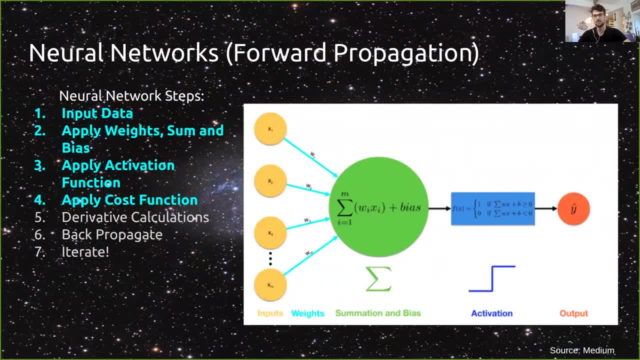 much higher resolution and in that case, if i remember correctly, you're looking at uh, disentangling multiple components that you might see uh in radio spectra, right? so that disentangling radio component or disentangling multiple components in a radio spectra, and i, for everybody else, let 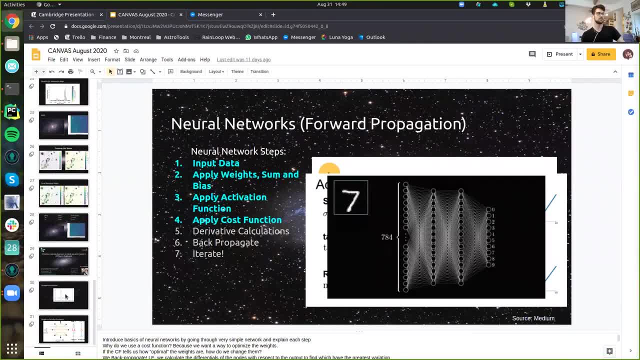 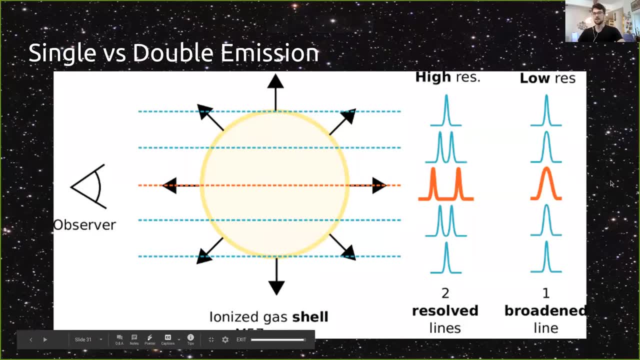 me pull up a slide really quickly. um, that's absolutely something that we want to tackle with this approach for satel. the idea behind these multiple components for everybody is, if i'm an observer looking at h2 region or whatever, depending on where i'm looking, i 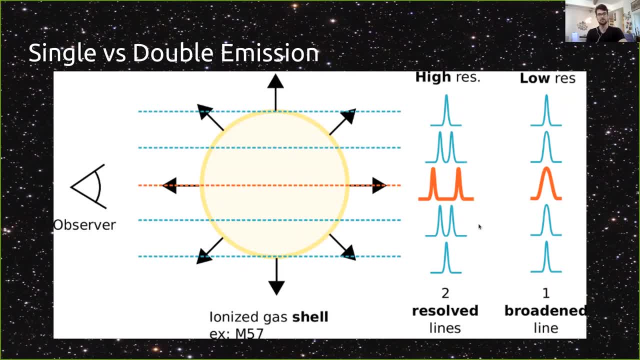 will be seeing different pieces of the gas. depending on my resolution, i will. i might be seeing those different pieces of the gas. so, for instance, i'm looking right through the middle of this- um, wonderful, wonderfully spherical h2 region. i have a piece coming towards me and a piece going away from me. if i have high resolution, i can disentangle it and see. 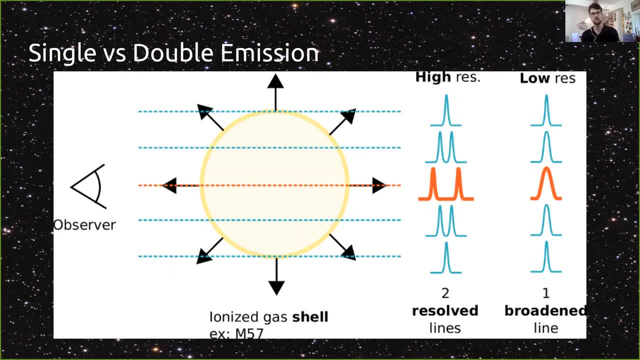 those two. If I have low resolution, I cannot disentangle those two. If I remember correctly, the data in Jared's case was a little bit higher resolution than we normally see on Sattel, so you were actually able to do a decent job of disentangling these two resolved lines. 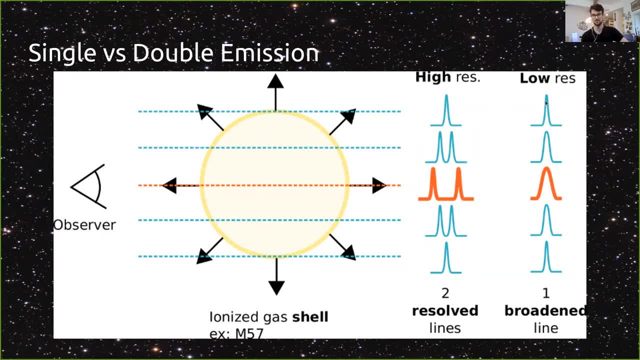 Unfortunately, with the lower resolution of Sattel, normally we're in this low resolution scenario, Not always, of course, but oftentimes we are. You need to go, at least for Sattel, closer to 7,000 or 8,000 spectral resolution to actually be able to see the two lines. 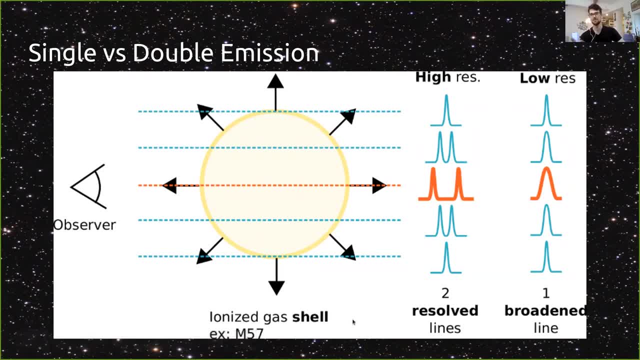 That being said, we are very interested in one of the last paper that we plan on working on on this is to see if we can't train a neural network to disentangle these lines, or at least give us an indication if we can disentangle these lines. 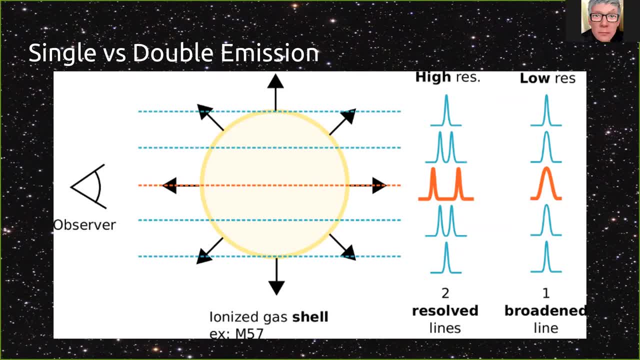 Can I ask a follow-up question, Dennis? Yeah, sure, Okay, thanks. So just the data that you showed, where you had a line that was a little bit higher resolution and then you had a line that had the fit, was that of a single line or was it one of the three settings where you have? 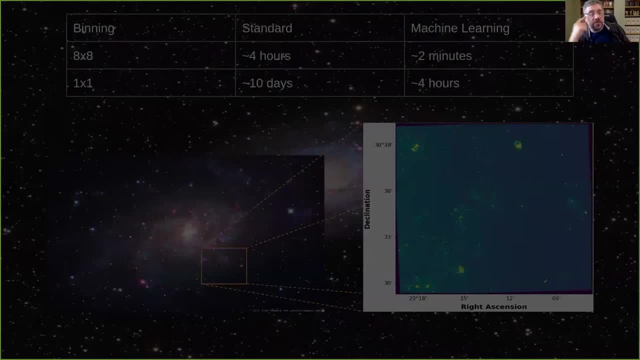 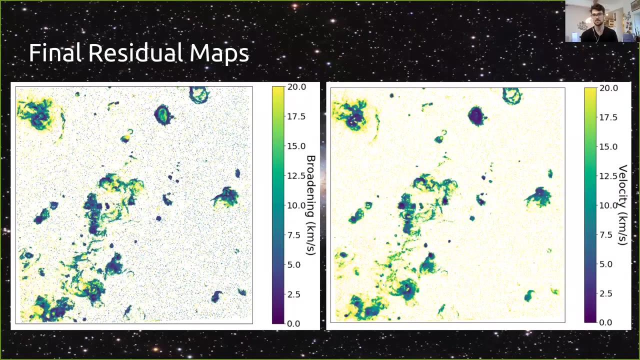 multiple lines. It wasn't clear to me if it was H-alpha or oxygen, Sorry, so we're looking at the. we're looking at H-alpha, the N2 doublet and the S2 doublet, So we're looking at all those. 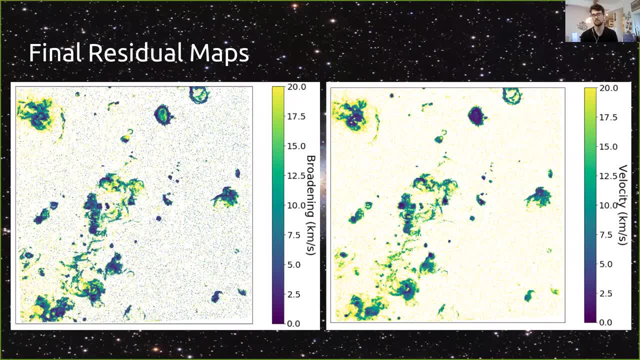 lines that are apparent in the third filter of Sattel. Okay, Higher resolution: 5,000 Sattel. So my question is: my later question is what. I can see that that's another layer of complexity added to the situation. 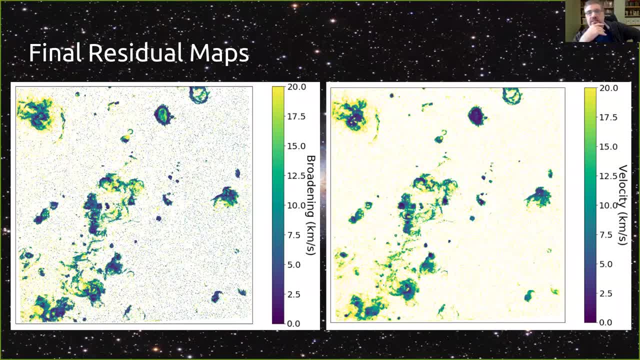 because you might have different lines at different heights. How do you, how do you account for that? Like, how do you train your network to account for that extra complexity? I mean, you could almost have an infinite amount of different. well, maybe not infinite, but you 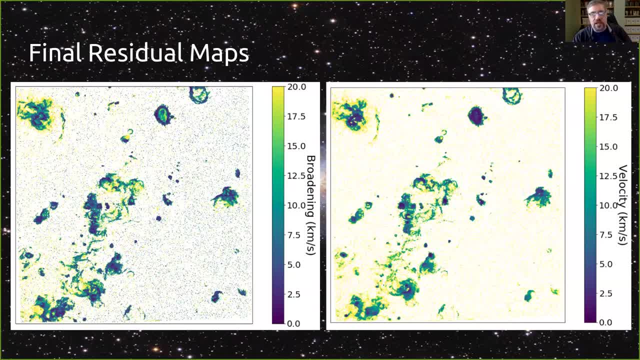 could have quite a wide range of different inputs for having different lines of different inputs. So you can have significantly different inputs in your H-alpha. even though in my examples it was always the strongest peak is not in fact always your strongest peak. Sometimes the N2 doublet. 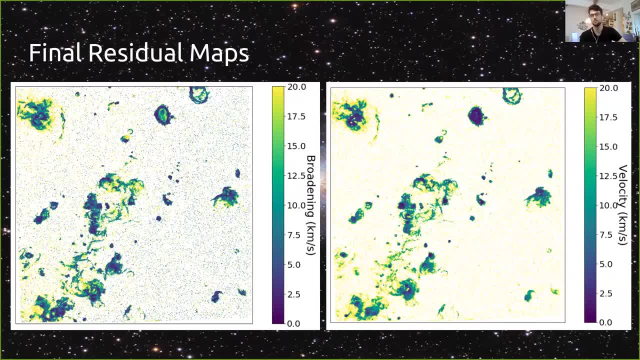 has a higher flux than H-alpha, which means, as you're suggesting, template fitting in the scenario would not work very well, which is exactly why we're using a neural network. What we do is we normalize our data to the peak in SN3, whether that's H-alpha or N2.. We tried normalizing it to. other peaks as well, and we found that as long as we have a higher flux, we can have a higher flux. So we can have a higher flux, but we can't have a higher flux. So we can't have a higher flux, but we can't have a higher flux. 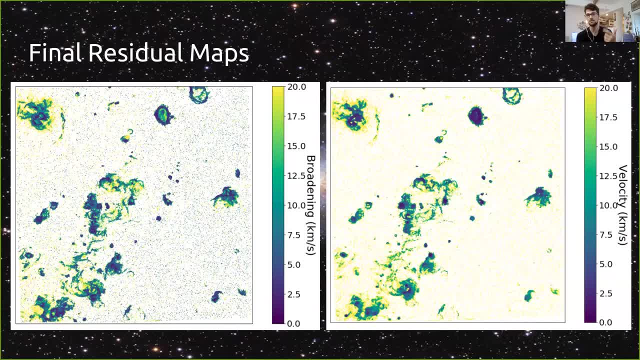 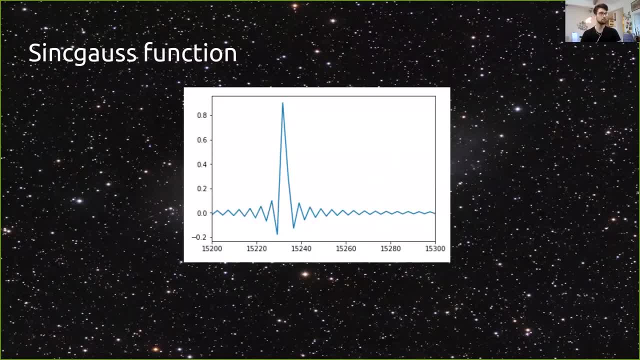 And we found that as long as it was either the max peak or H-alpha, we get consistent results. I'll also mention one very lovely and annoying thing about Sattel. Sattel, if you take a look at it, if you pick a line, this is H-alpha, for example. 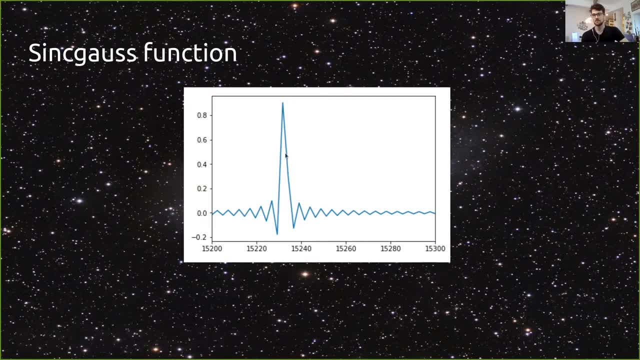 you're not going to come up with a beautiful Gaussian. That's not the response for Sattel, It's actually the sink Gauss function And you see these lobes here. They're incredibly important and they're affected strongly By your velocity and broadening. So it's not as simple to just look at the main peak. 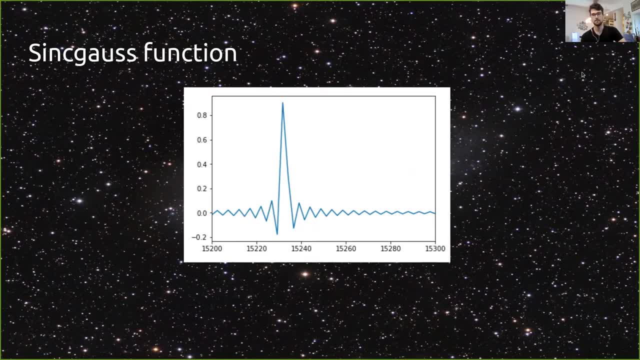 You actually have to understand what's happening elsewhere. That also sets it aside, if I remember correctly, a little bit from Jared's paper. Okay, Thank you very much. Thank you, Jared, you're next. Okay, thanks, Yeah, so I'm Jared. I'm the student that James was referring to that worked on the. 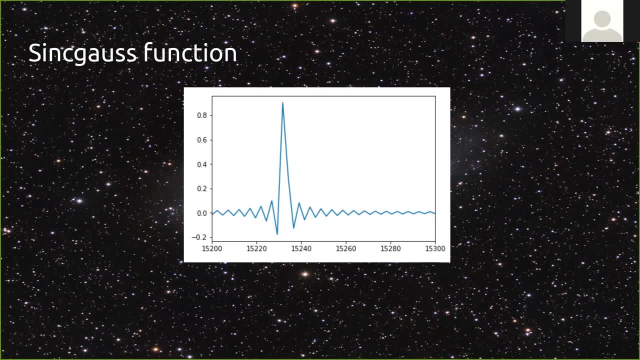 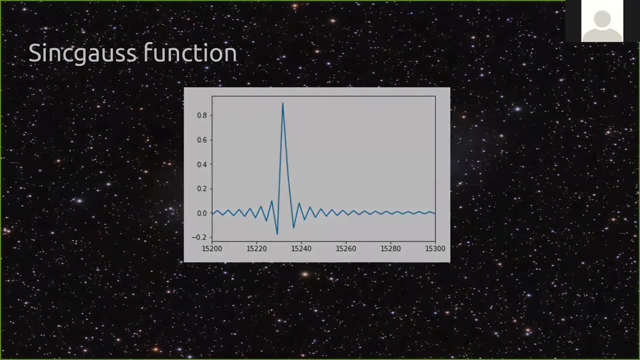 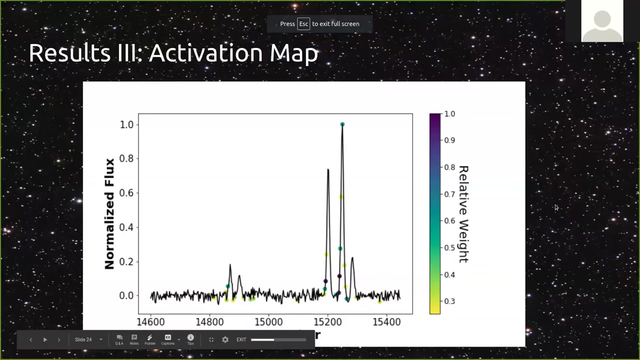 the clover paper. But I just had a question about why you didn't include the brightness of the emission lines as an additional output. Because if you look at your saliency map it already looks like the network is using those peaks. So it seems like a natural follow through to just go ahead and add the 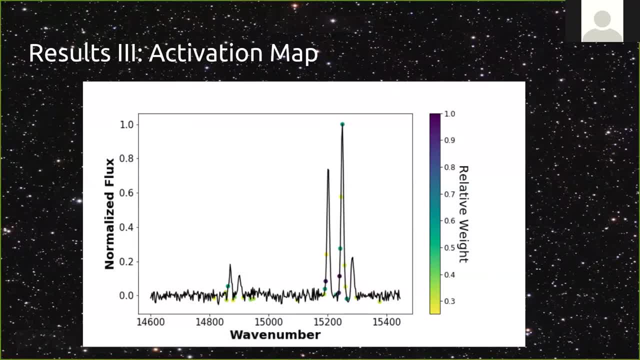 height of the emission lines as an additional output. I know I've asked- You had planned to do that later, but I'm just curious why you didn't add it onto this network. Yeah, why not predict the height of the emission lines as well? 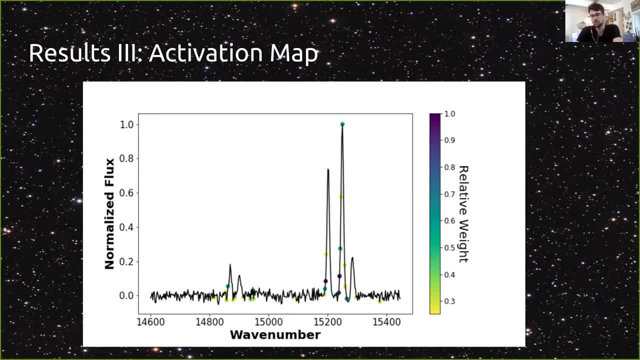 So you've asked the perfect question. There's a couple reasons why we weren't adding the height to the emission lines initially. One of the main things is that they're all normalized. So even if we get the height of the emission lines, that doesn't. 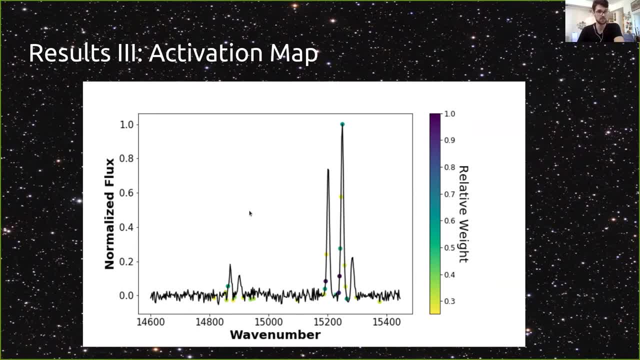 necessarily give us a flux. We have to know base flux to denormalize from. That can bring up another question of another really important piece in H2 regions in the study of H2 regions is to look at line ratio fluxes, So the ratio of the flux from, let's say, H alpha to an N2 delta. Normally it's the other way around, but that's okay. 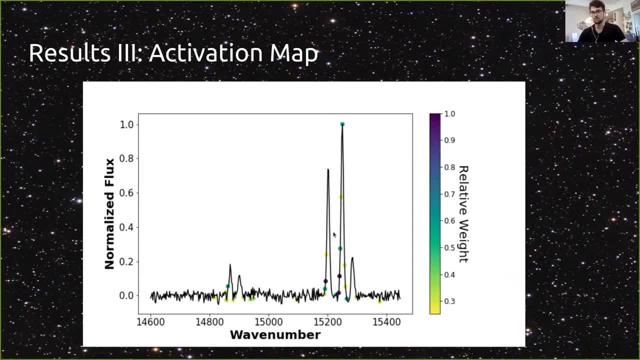 That's exactly what we're doing in our second paper, which is at a very mature stage, So it should be sent in for publication sometime soon, Within the next, sometime at the end of September, I bet. Okay, Sattel again is a little tricky because, as I showed, it has that sin Gauss function, So some of that flux is held in those lobes of your sin Gauss function. So it's unfortunately not as simple as just looking at the peaks. 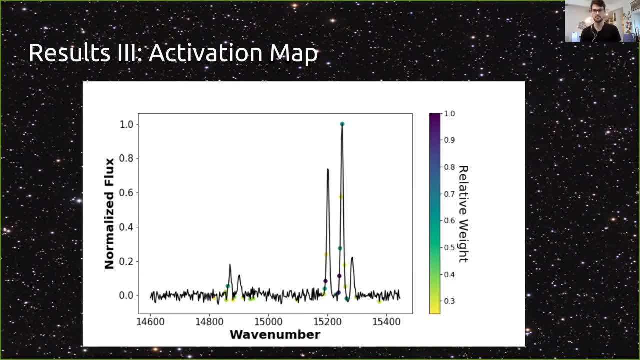 You can't just get the amplitudes and then take those ratios. to get those real line ratios You actually have to take the fluxes. So we are using another neural network- this time not a convolutional neural network, just a normal neural network- to tackle that problem of line ratios. Sattel again is a little tricky because, as I showed, it has that sin Gauss function. So it's unfortunately not as simple as just looking at the peaks. So this is unfortunately not as simple as just looking at the peaks. 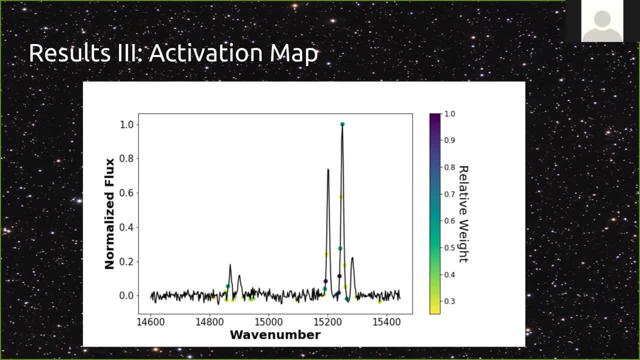 Okay, Does that answer your question? Yeah, that's great. Thank you, Toby. you have a question? Yeah, Hey, thanks, And great talk, Really enjoyed it. And so I'm not expert in this, but it's my understanding that with this type of stuff, you really get out what you put in. 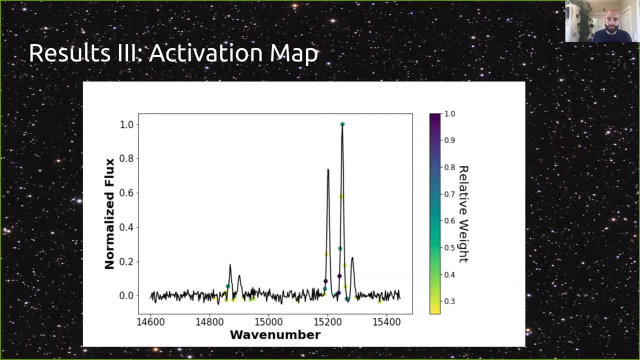 And you can. Okay, Okay, Okay, Okay, Okay, Okay Okay, touched on this throughout the talk and spoke a bit about it, but i was wondering, um, if you could sort of encapsulate just how much the choice of your training set or whatever you're training? 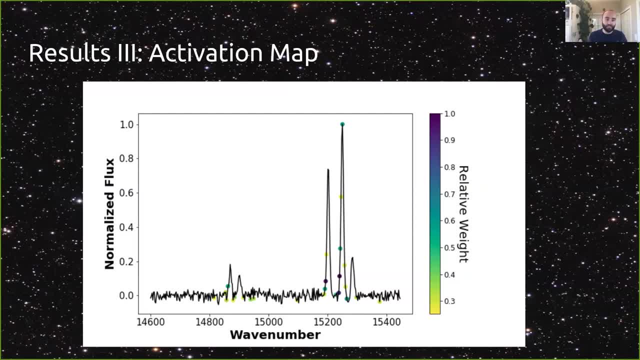 your network on really impacts your results? and also if, like down the line, when you make, say, the code public or where you want other people to use it, would they be choosing their own training sets, or would this be something you would set and it's hard coded in? okay, um, so you're? 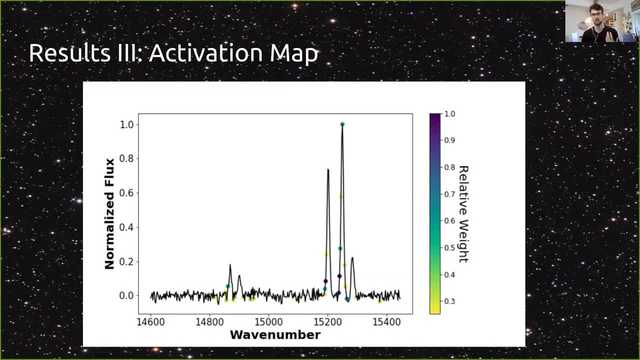 yeah, i think you summed it up perfectly. and there's an old adage: garbage in, garbage out. if your training set isn't good, it doesn't matter how perfectly tuned your neural network is or whatever machine learning algorithm you have. if your inputs are garbage, your output is going to. 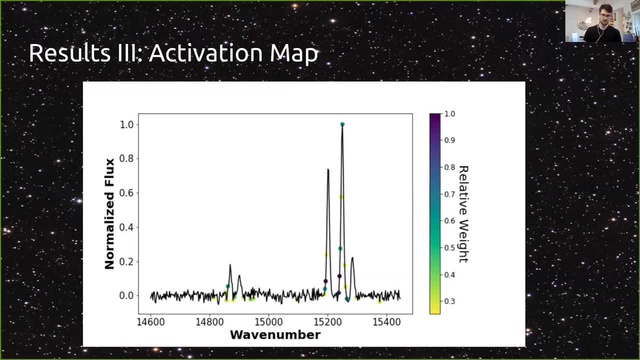 be garbage all day. there's a lot of fun memes about that um, so your input obviously matters quite a lot. it took us a very long time and actually the one of the hardest things to do in this project was coming up with the kind of perfect um input, the perfect synthetic data, which is why we were so 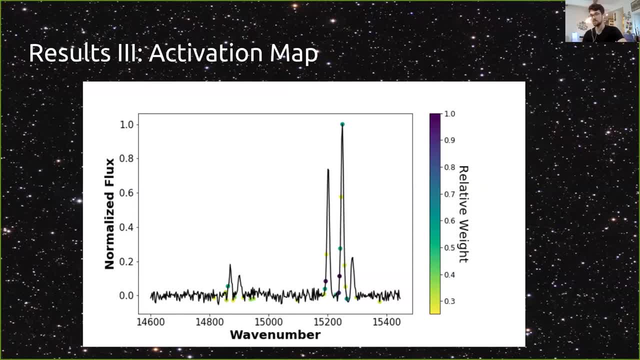 careful and tedious when choosing, for instance, the bond simulation to pick out our amplitudes for those different emission lines. the bond simulation has has a lot of success, um, and doing a good job of replicating observations. uh, as for, in the future, people using um and building their own training sets and and using this neural network for their 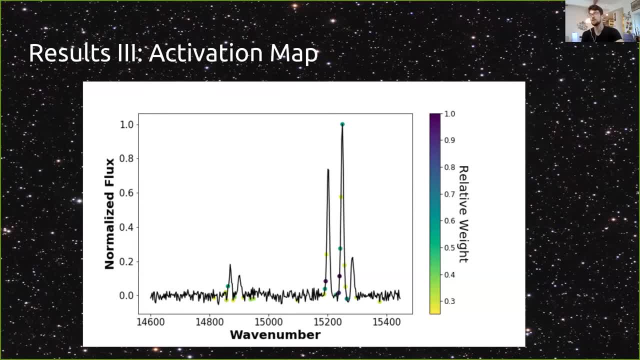 own data. it has been trained for multiple different resolutions- uh, just for sitel. so a user has an option of picking the resolution they want and simply typing it in and then running through the code um and i. there's an example- my python notebook in the github repository that demonstrates how we build the synthetic data sets. 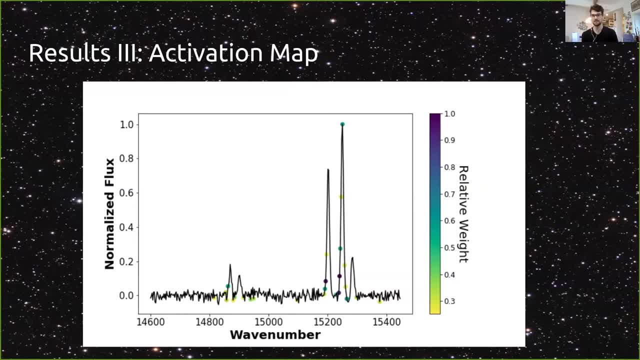 set. so if people need to tailor a synthetic data set slightly to their problem, they'll be able to build their own, and there's also a notebook that shows you exactly how to retrain our algorithm so that users can go back, tweak for their exact case, rebuild the network and use it from there. 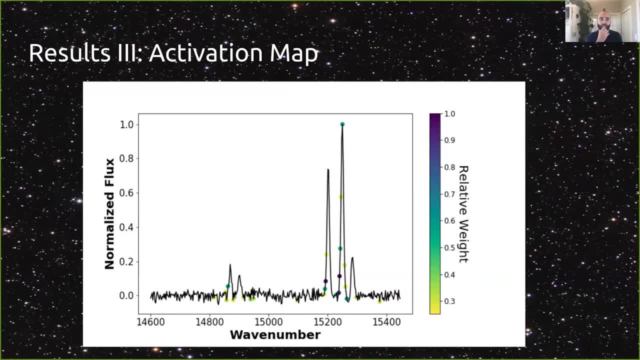 nice, that's good. and then sorry, just one follow-up. so you built this for sitel, but presumably you could use it for other ifu right or ifs, absolutely. instruments, absolutely. we've been talking, uh, with the people at muse about using this um as well, and it would. oh, that's great, it's the same idea. 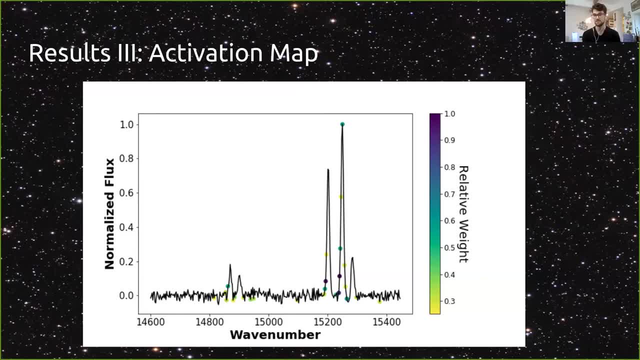 you just want to train it on data that's specific for a little more specific from you. so the resolution, and you also want the instrument response for muse. when building the synthetic data, we use the exact instrument responsives to tell, which is why it's a little more tailored. 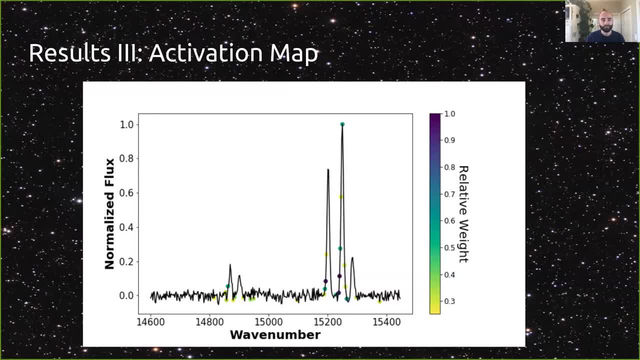 towards the tail because of those weird side lobes that drive everybody nuts. yeah, sounds good, great. and another reason why we put those ipython notebooks and everything online- uh, i think they're pretty well documented- is because we want people from other instruments to go through and simply train a little differently. they'll be a different training. 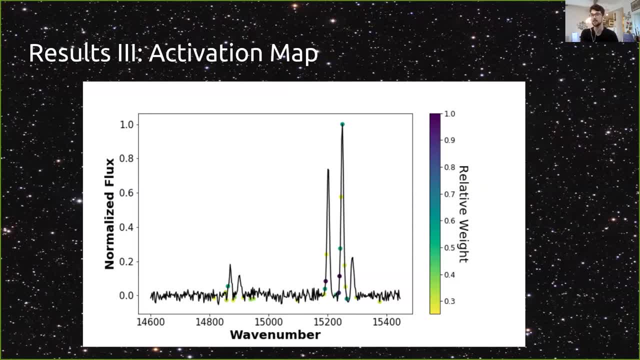 set and then be able to use this algorithm directly on their data, so it's tailored for them. so, carter, i have a question: uh, is this being will be utilized by the signals project, uh, replacing the standard data set, so the standard reduction code, or how will it actually be utilized in practice? 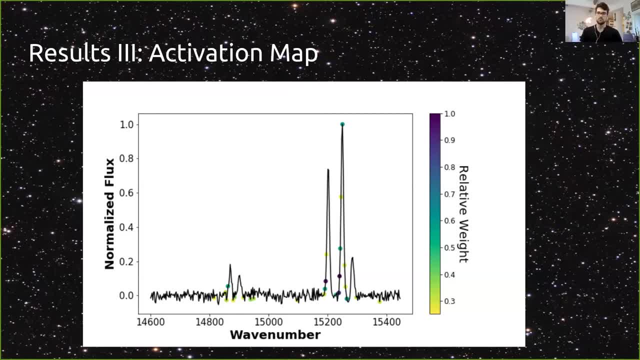 so it's- uh, we haven't decided if we're going to use it to to calculate their velocity and broadening parameters instead of the standard methods. it's absolutely going to be used to calculate the priors that are necessary for those standard methods. so that's actually being i'm working with the orcs team at university of vol to incorporate. 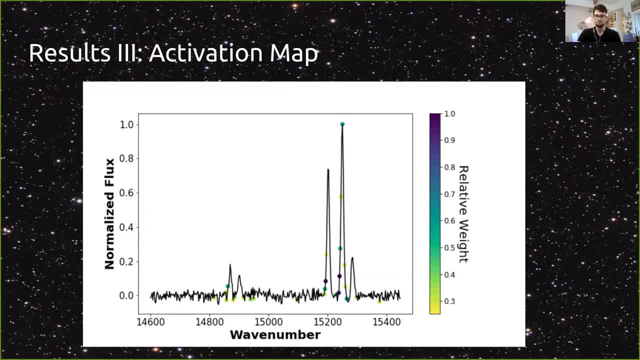 that into their standard pipeline. um, we are also working on some other things. like i mentioned, we're working on the line ratios and we're actually seeing really wonderful performance on that uh, and that will very likely take over as the main mechanism for calculating line ratios. uh, for the signals project. i can't say for sure, but that's, uh is certainly something we're thinking. 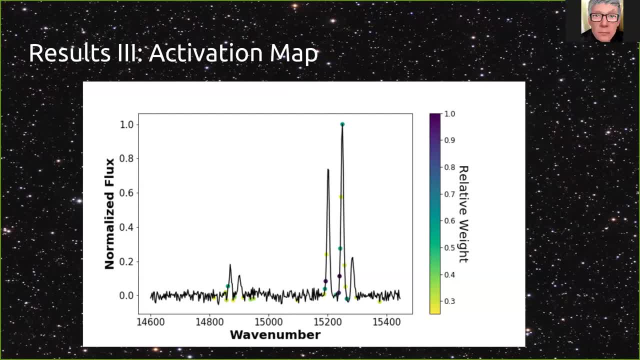 about and blake has a question. yeah, sorry, uh, thanks, i hope i can ask one more quickly before we end up. but um, carter, when you were showing your about your final um residuals- and you were, you went from like the negative 30 to positive 30 spread to just having 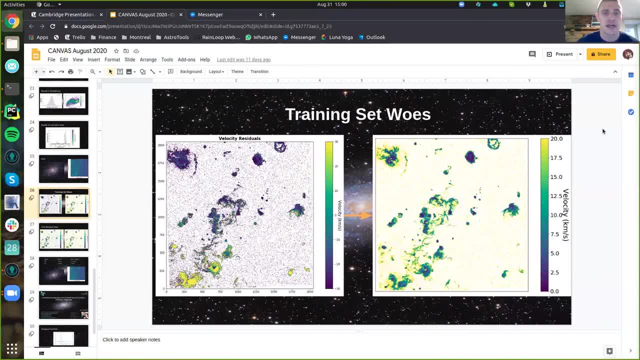 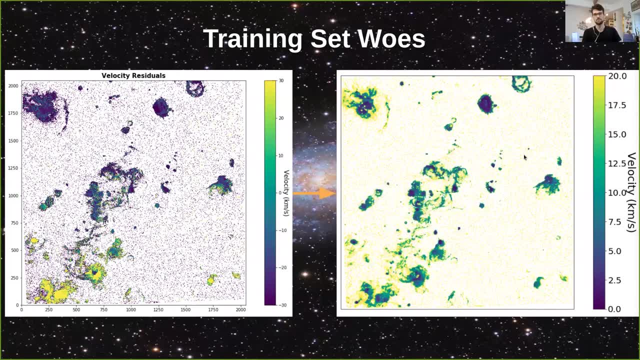 uh, the positive 0 to 20.. um, yes, was that map on the right also the residuals, or is that just the velocities that you obtained? i'm sorry, that's also the residuals. um, so that's right after you've kind of shifted your resolution to have like that normalized baseline, right, that's correct. so. 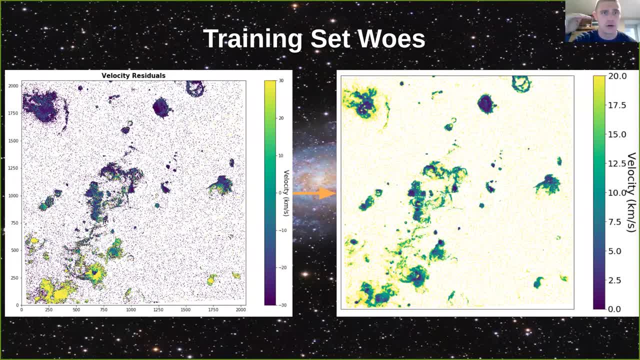 does that? is there an implementation of like a positive bias then in your um, in your new velocity, there is is. this image is a little misleading because this is absolutely on the right hand side. it's the absolute value of those residuals. of course they're always going to be positive, okay, but 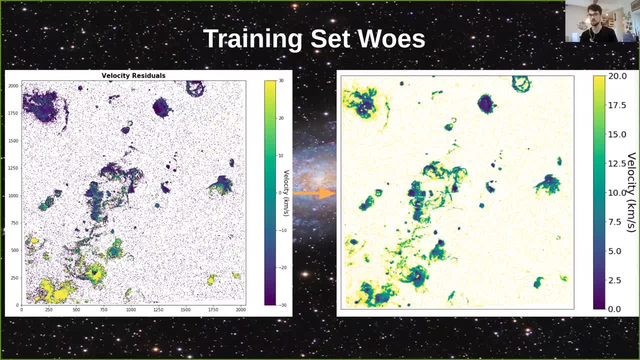 when you look at the non-absolute value, yes, there is a slight bias towards positive velocities. the reason why we chose to have the absolute values here and not here is because we wanted to show the systematic spread, yeah, and how it really changes from negative to positive. 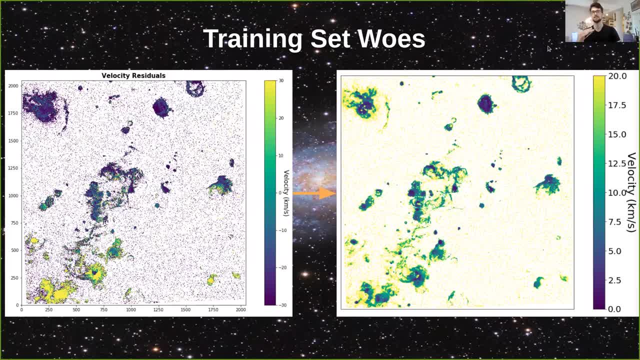 but yes, there's an overall systematic, uh, positive, like we're over estimating the velocity slightly, but yes, there's a trend and that's just like a result of the network, or just we think it is a result of the network. um, another issue is that, the signal to noise ratio. so, even though we 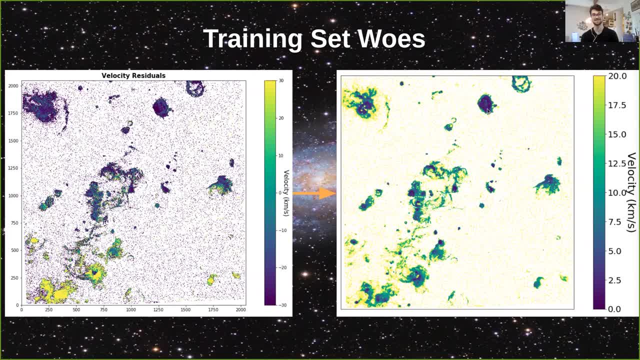 have high resolution, the signal noise varies drastically throughout the cube. um, here we've done some masking to only pick out higher signal noise regions. but here, where you have the yellow um so the the worst residuals, that actually correlates, that actually correlates perfectly to um. low signal to noise, yeah, the worst data. so there is a very strong correlation between bad data. 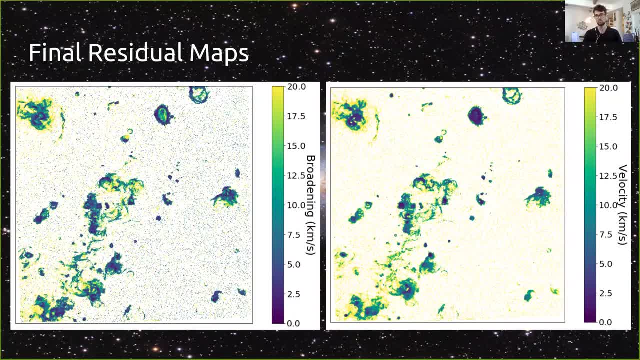 or not as optimal data. bad signal to noise and you know worse estimates, but in these high signal to noise regions the errors are normally within a couple kilometers per second. right, cool, yeah, thanks so much, appreciate it. and one quick question for me: what is your phd thesis on? 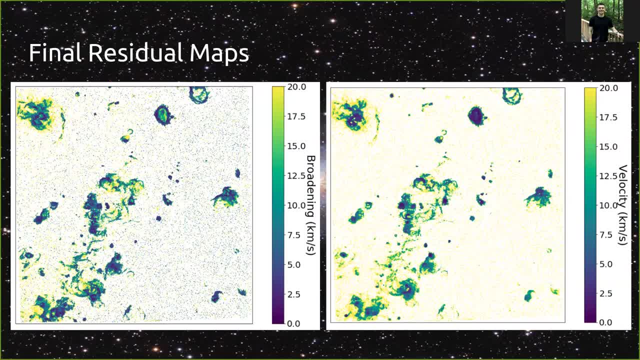 uh, my phd thesis. uh, instead of just a project, it's more of a theme. so the idea is to use machine learning techniques in the future of optical and x-ray astronomy. i have another paper that just got accepted, actually right before i started this talk- on using another machine learning technique. 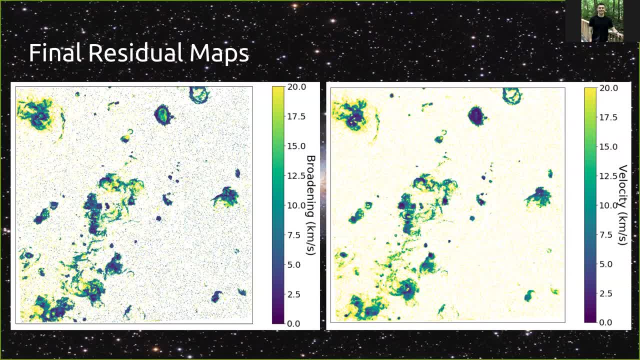 called principal component analysis to disentangle multiple temperature components in x-ray spectra. so i'll be doing some follow-up work with that with the people at cfa. excellent thanks again for your time and i hope you enjoyed this very, very well presented talk, very interesting subject and